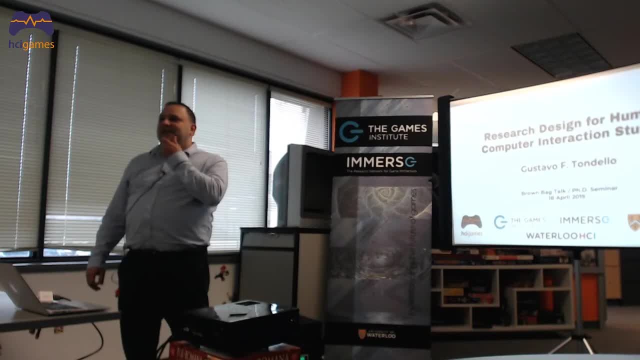 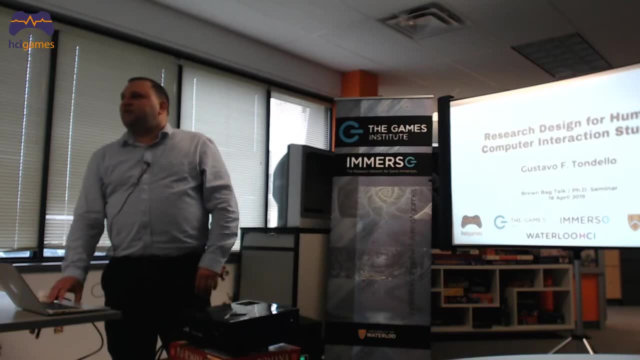 the end. I want to bring a little bit of this experience, hopefully bring something that is going to be helpful to you. Maybe some of these things are obvious or maybe you already heard someone talking about them, But if not, I hope that my experience you can learn something. 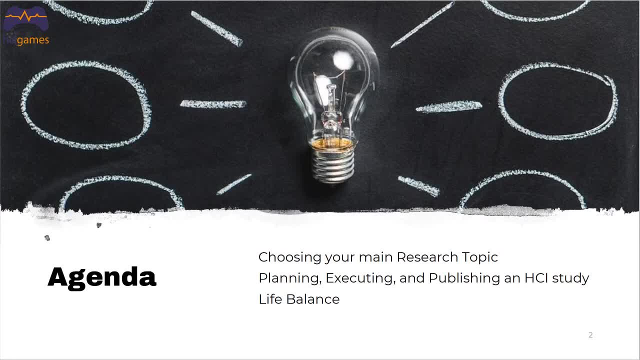 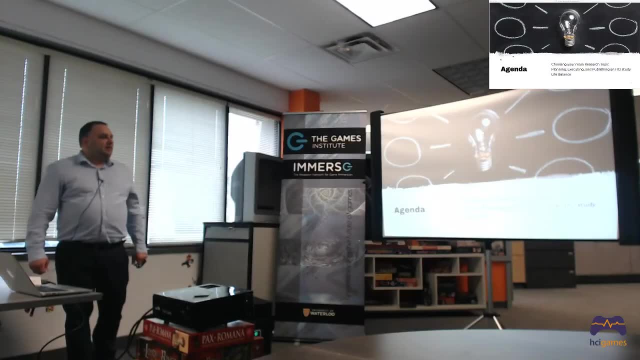 that will make your life easier when you're doing your studies, Thank you. So I'm going to talk about choosing a research topic And I'm going to spend most of the talk talking about planning, executing and publishing studies, And I'm going to talk. 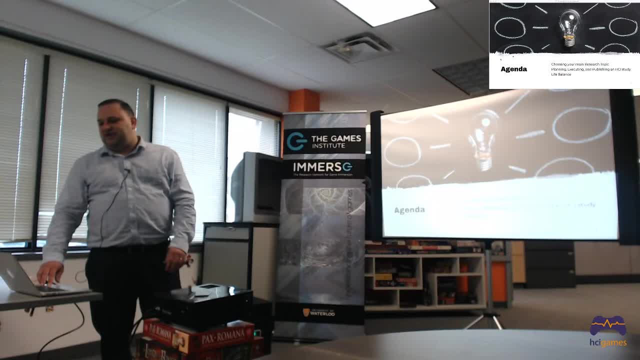 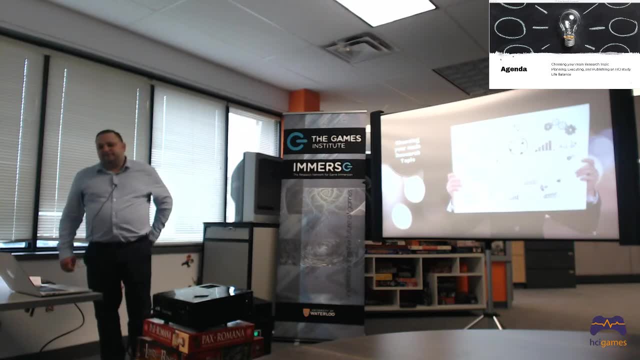 a little bit about how to balance all these things in your life, which is not exactly part of the study, but it's an important part that also influences everything. So, okay, Before you actually begin planning individual studies, you need to have a very 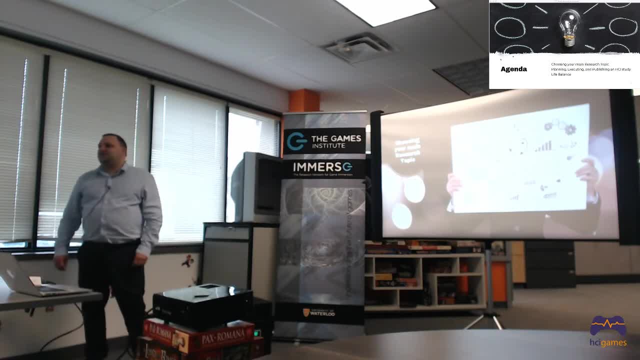 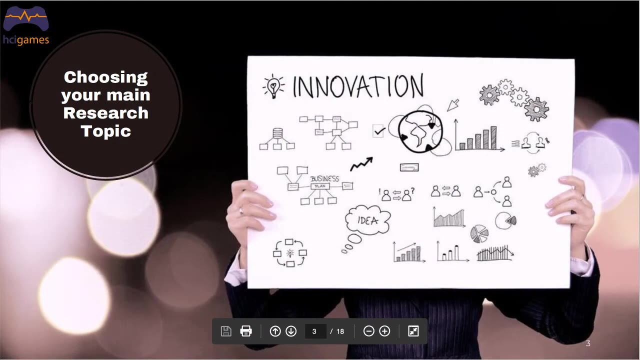 main research topic right, So there are lots of different ways that people use to choose a research topic, So some already have an idea that they carry from previous research work. Some have just an inspiration for something that they can do and that they want to do. 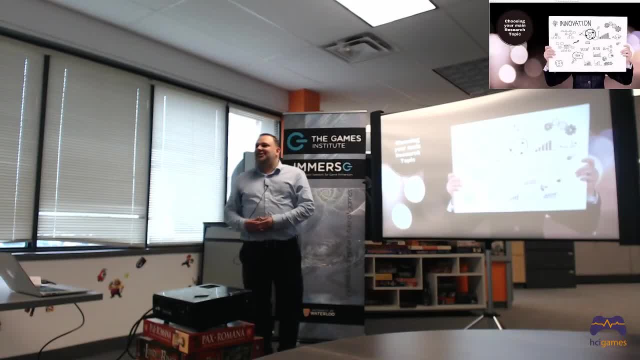 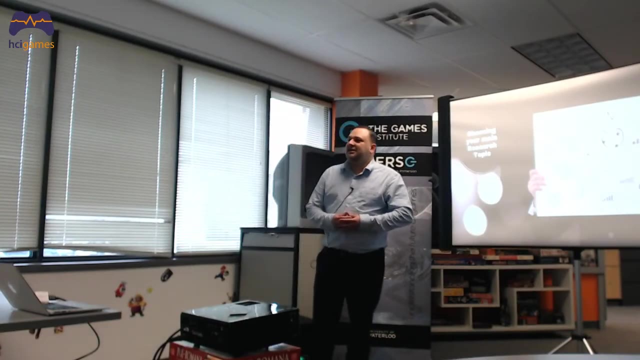 Some can begin their graduate studies not entirely certain exactly what they're going to do, And they need to find exactly what that is. So how do you do that? So, again, I cannot tell you exactly how you're going to do that, which is different for everybody, But I just 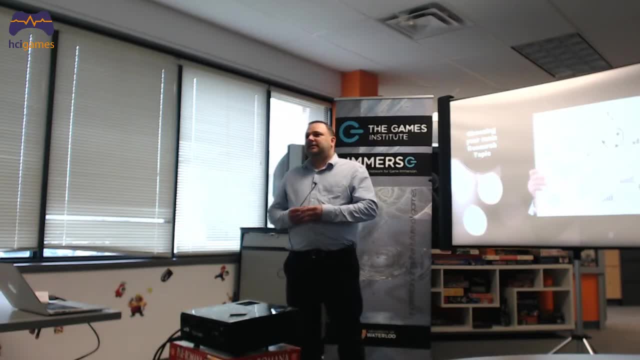 wanted to bring that from my experience. If you still don't have your topic and you're still looking for something, it is a good idea to get involved with what people around you are doing and see if you can fit your research there, Because sometimes it might. 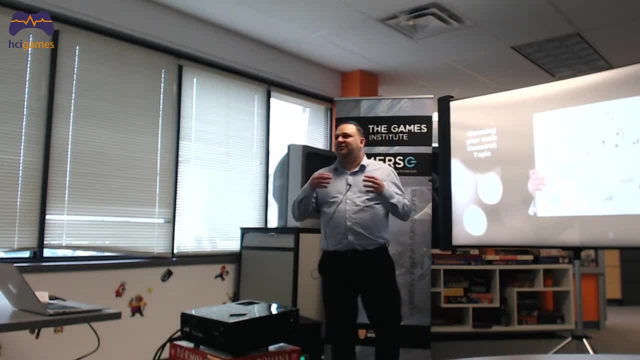 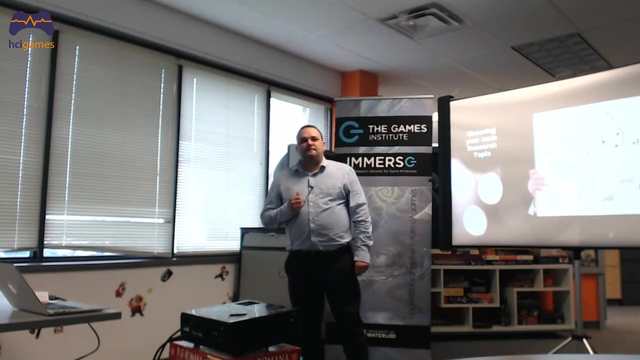 have this expectation for ourselves that since we have to do something regional, then we have to come up with that amazing idea that nobody has ever thought about And that puts a lot of pressure And that isn't really necessary. Research is done a lot of times. 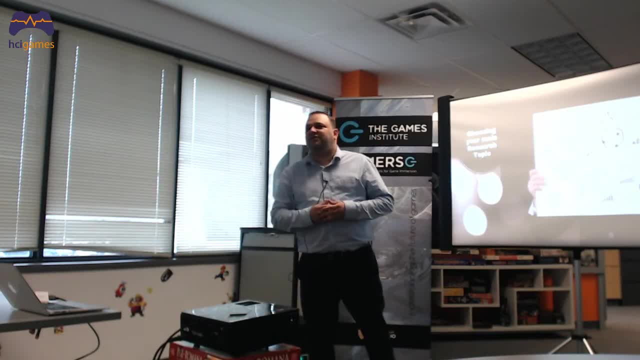 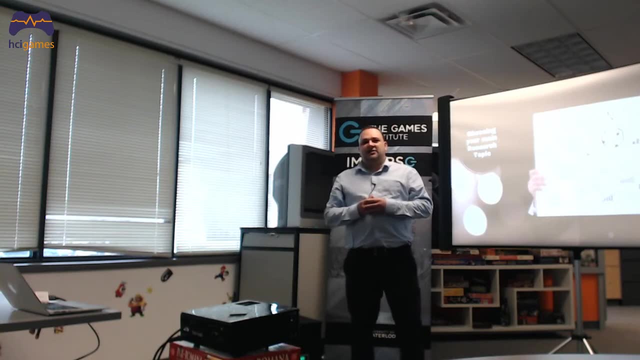 just by building a new block on top of what has been done so far, right? So if you look at what has been done so far, what people around you are doing, then you can find there one block, one, the next step in something that nobody has done yet. that's a good topic. 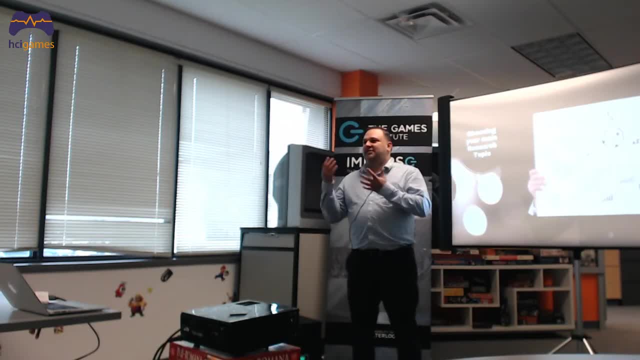 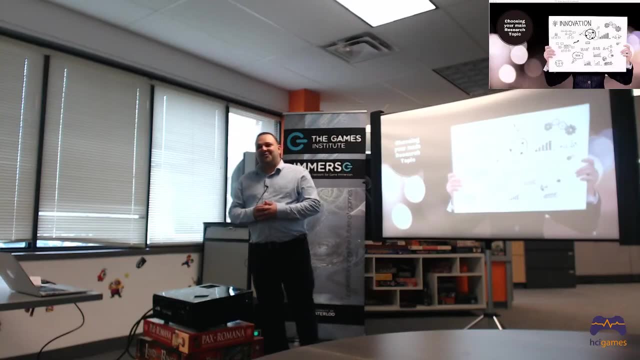 right there, And it makes your life easier if you're working with people that are also doing similar things, right? So if you do have an amazing original idea, you're going to invent a whole new research field. It's great. Go ahead and follow it. But if you 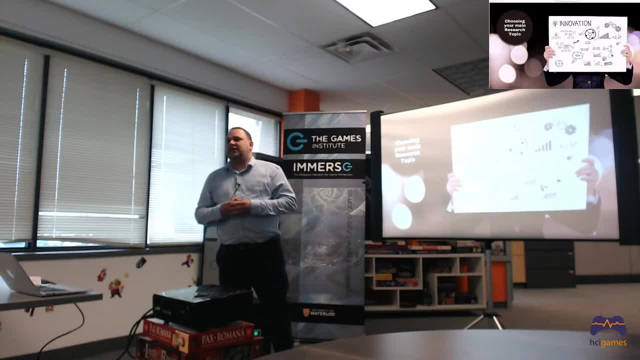 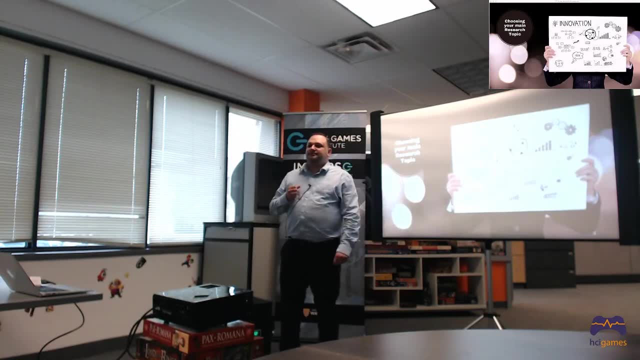 don't, and if you look around and you see opportunities, I think I'm probably looking for a good one. or just learn from the experiences To choose a topic that's going to be quite enough right? That's what happened in my experience. for example, I came here to the 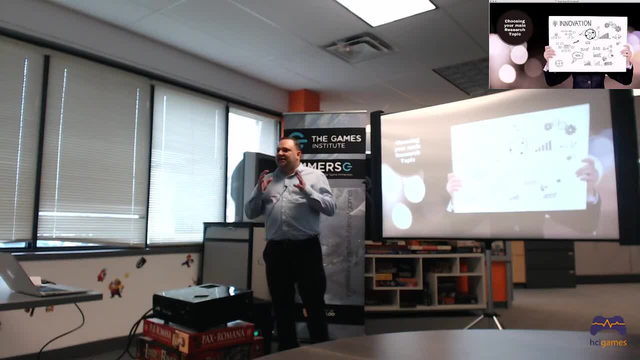 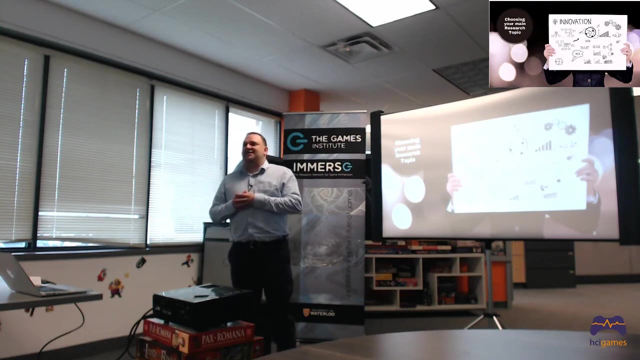 MIT, knowing that I wanted to work on gamification, But I didn't know exactly what I was going to do. The original idea that I had was related to developing some health gamification application, But when I arrived here I didn't find anything I was interested in. I didn't go into the 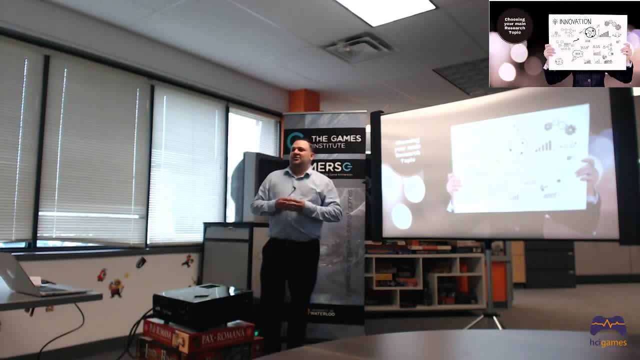 around me so I was already working on that. But on the other hand, the first months when I was working on my PhD, there were people talking about how to study user touch, to personalize in applications. There was a person from the gamification industry. 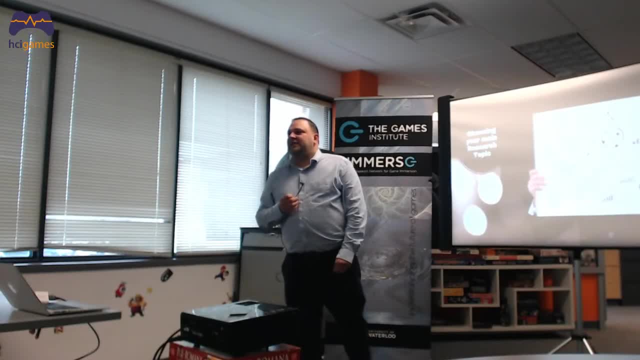 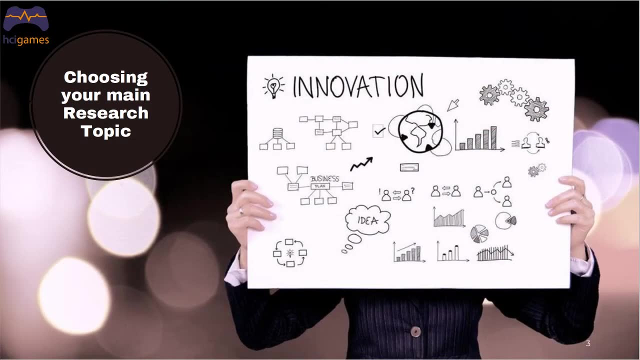 that was starting a project on that and looking for academic collaborators, And I contacted him and began working with him. There I ended up working on how to personalize in applications, and it has been a great topic that I really enjoyed studying so far. 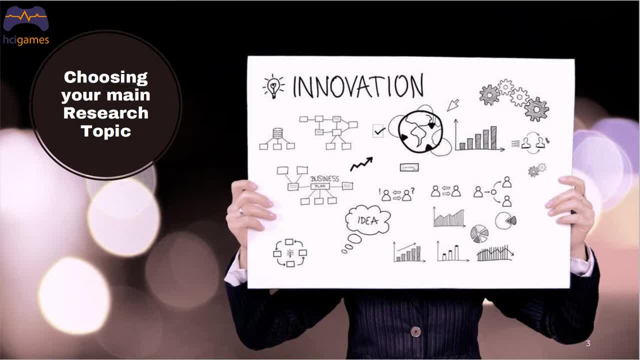 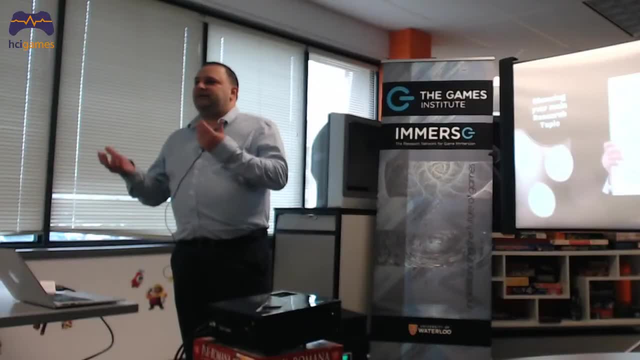 And I think it's going to be a good topic for my PhD- then So I'm saying, if you look for opportunities and one opportunity appears to do work together with other people or just to build on the ideas, go for it. 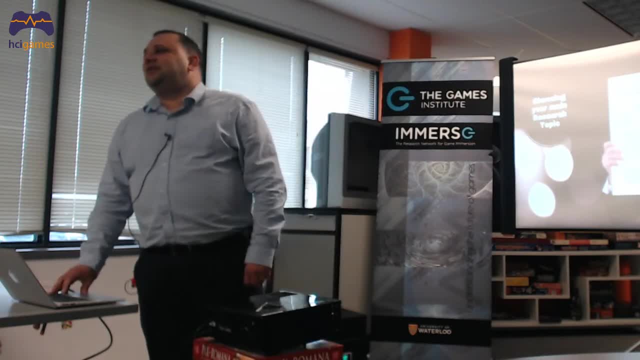 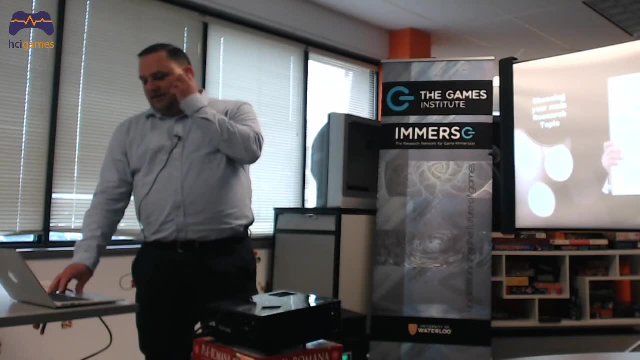 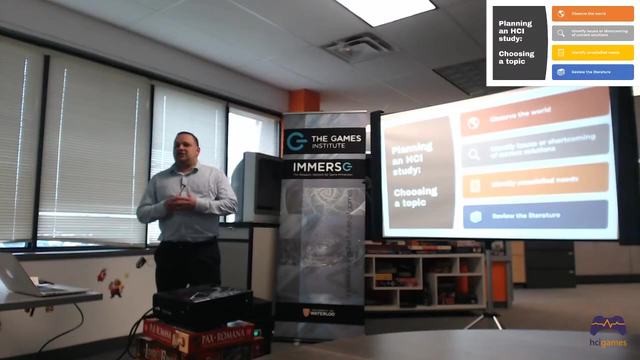 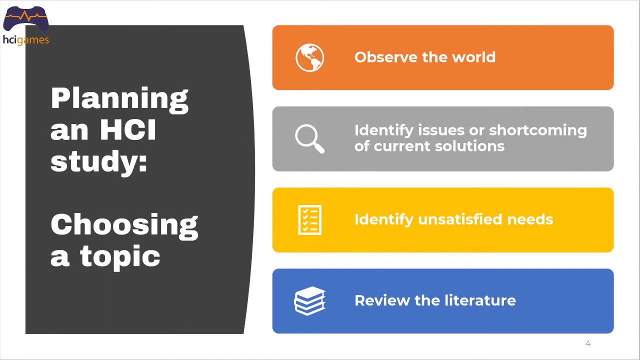 Never feel that it's not enough if you didn't come up with your main topic alone by yourself, because that's not the way, It's not necessary. OK, So moving forward. now say you have a main idea and then you're going to plan a few studies around that idea. 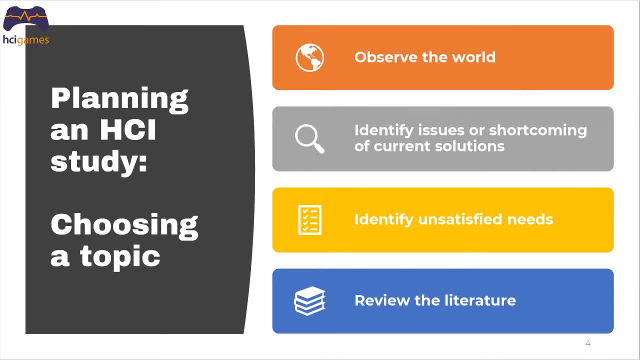 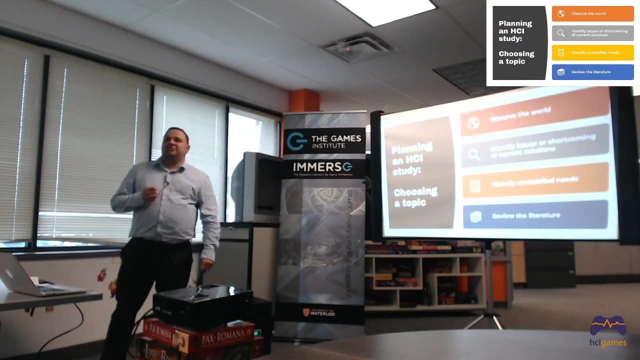 So how do you begin study? How do you choose a topic for a specific study? So I would say my experience, some of the ways that can help you. One is to investigate this, Observe the world around you, of course, so that you are studying. 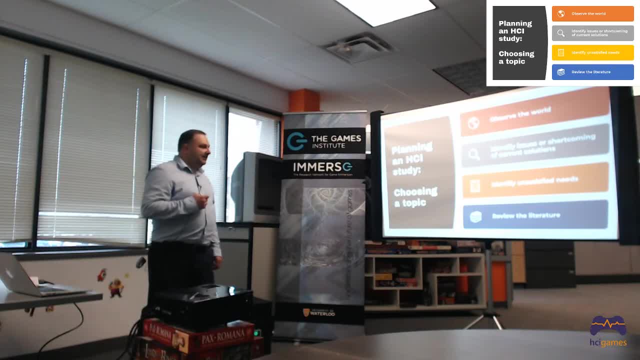 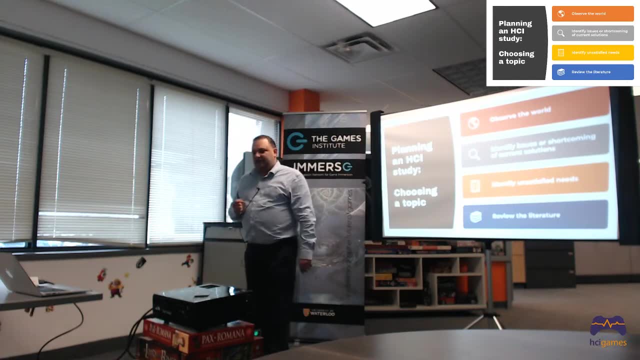 See what people are doing, what they need, And I would say what I have been trying to do and has been working: identify what are the issues or the shortcomings of the current solutions or what people need to do that they cannot do that. 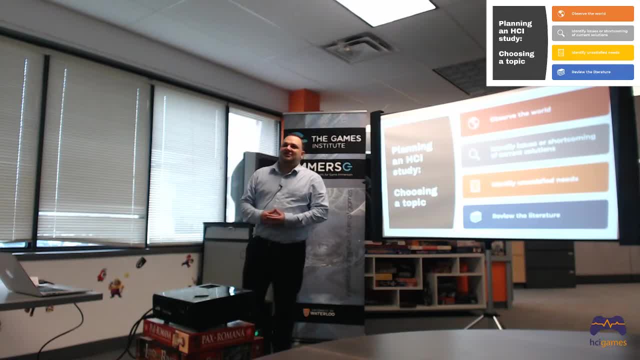 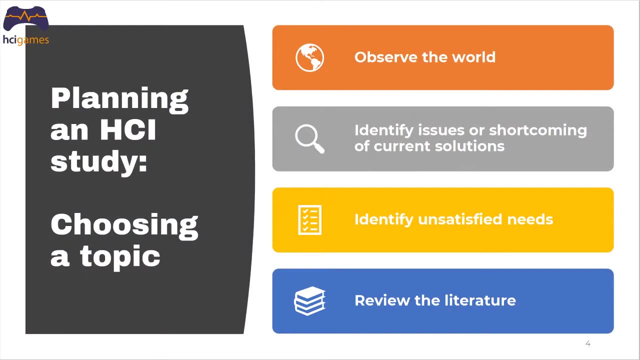 So again, if you have an amazing original idea nobody's going to have done anything about it before, it's great, go ahead. But sometimes very good ideas just come from. let's see what we have done before and how can we do the next step. 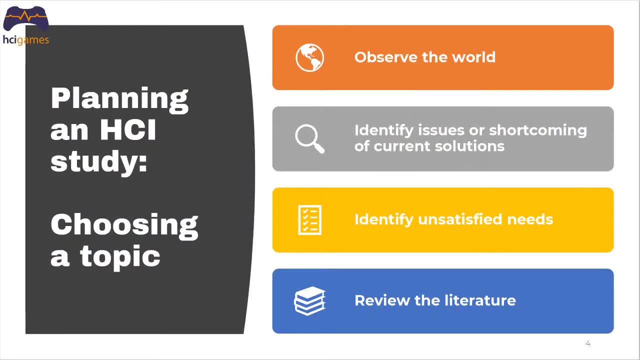 So, for example, some of the work that we have been done here around player types was just by taking on the work that had done previously- Some of you are familiar with the BringX- And then looking at that work and seeing that it had some shortcomings that we could try. 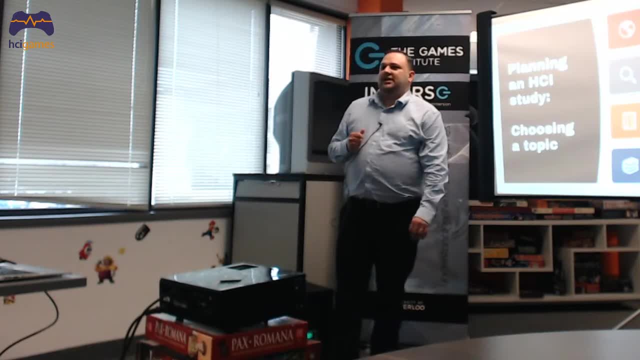 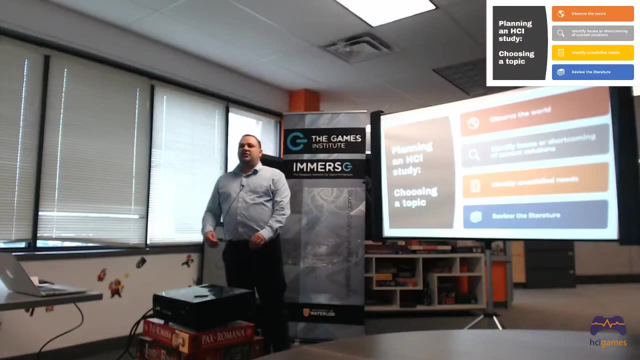 to further explore. So that ended up being not only one, but a few good research projects and publications that we have been doing Just by identifying this case, by shortcoming of a previous work and then thinking about how we could improve it. Other works that I've done came from identifying things. 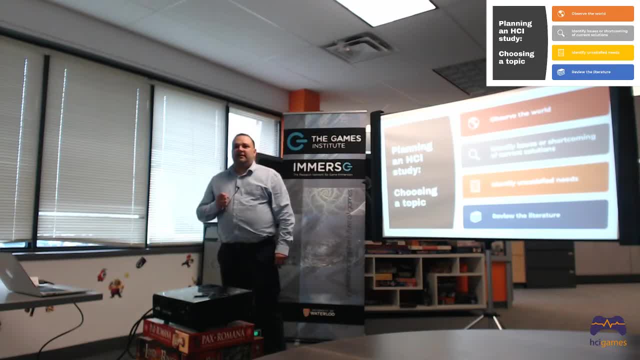 that people needed So in my work with personalized identification, because this identification consultant had an original idea how to classify user types identification But he needed to test if that was really going to work, if that model was really valid. So there was a need. 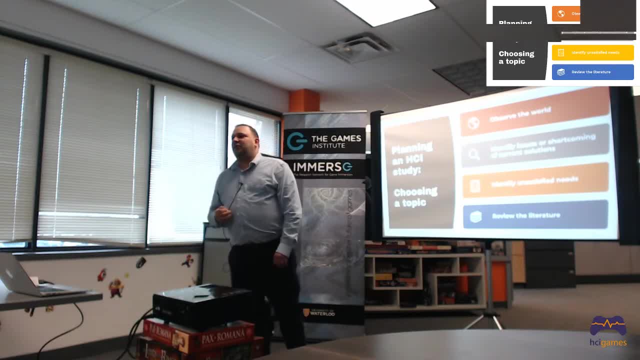 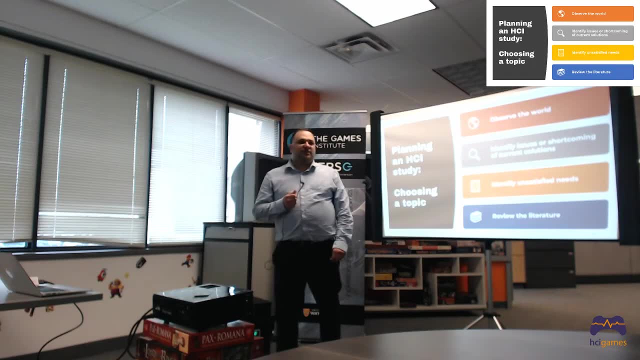 Someone was already looking for a partner to do that work, So I stepped in And it worked, Thank you, And it turned out to be really good work as well. Another example that we identified was the work that I did with the chemical design. 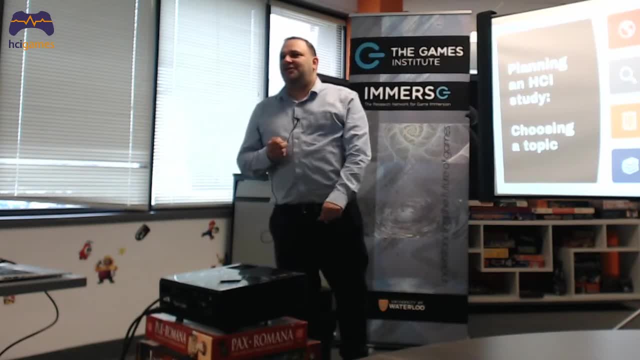 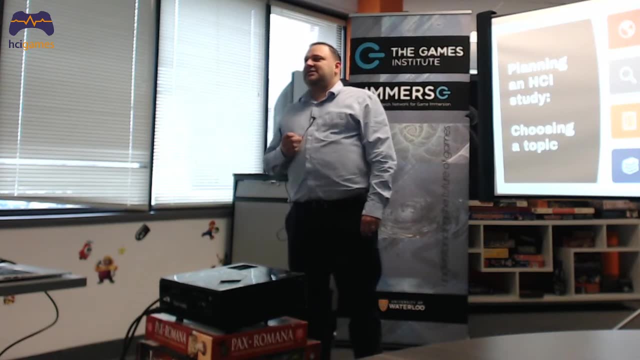 listings, maybe for the power poster there in the hallway. So for that work. basically we were working with another master's student And he was designing a game And we were asking ourselves: OK, how can we evaluate this game here? 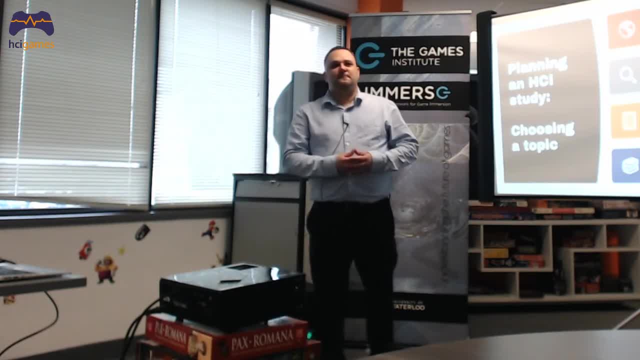 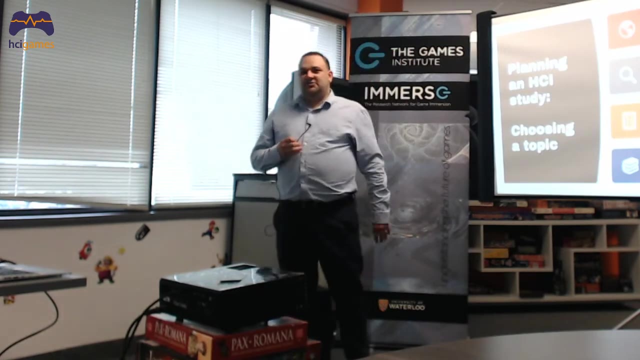 Just how good it is in terms of motivating people. And then we realized that we didn't have in the literature any formal methods to evaluate games regarding motivation. We had games evaluation regarding other things, but not regarding motivation. So there was a need. 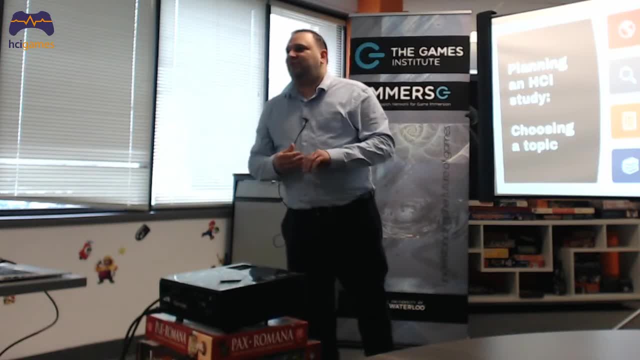 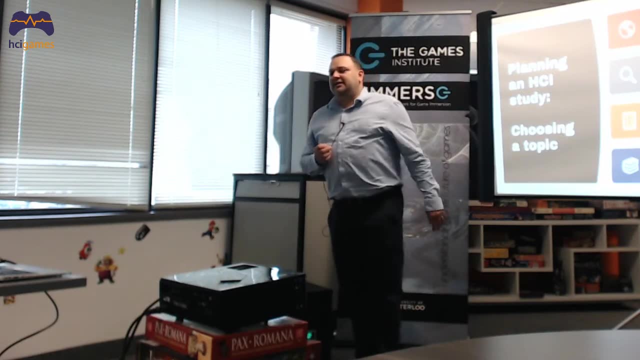 We needed to do something. No method was available, And then maybe, if we needed that, other people could also need similar methods. So, identified that need, I started a project to create the game for designer listings, which then is a method to evaluate. 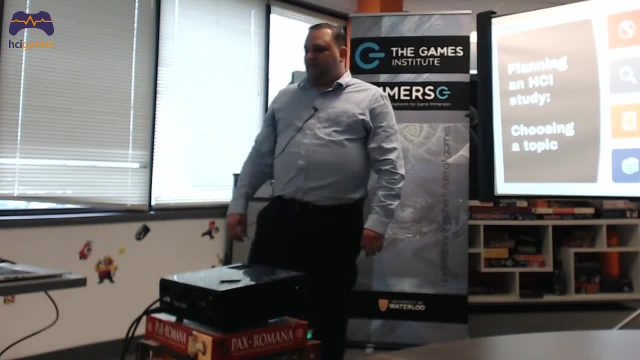 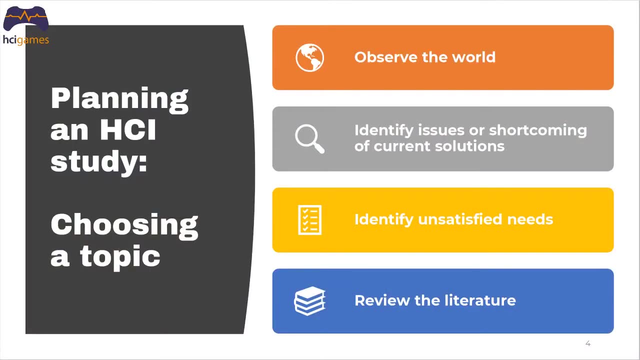 how good your application or game is on motivating people, And I put here review the literature as the last one, It should be one of the first. So a diagram that Joe posted on Slack yesterday that kind of said: observe the world, then come up with your question. 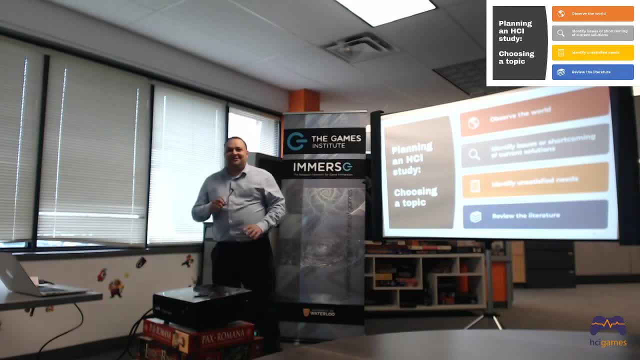 and then review the literature. I don't see it exactly that That way, because if you come up with your question before you review the literature, then chances are that you're going to ask a question that somebody already asked before, Because most of the questions that you can ask- 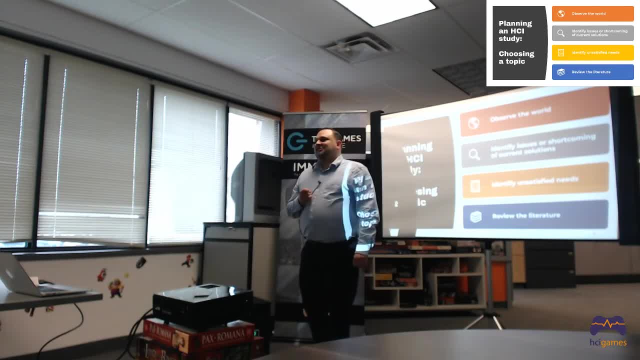 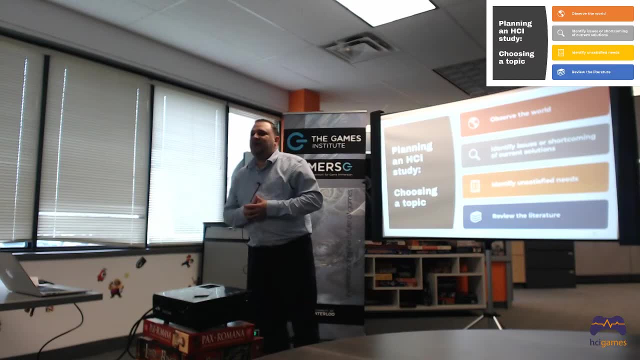 people have already asked that question before. Sometimes you might reach, you might find something that's really new and then maybe nobody asked the question before. Most of the times people already asked that question before, But that doesn't mean that you don't have a research topic. 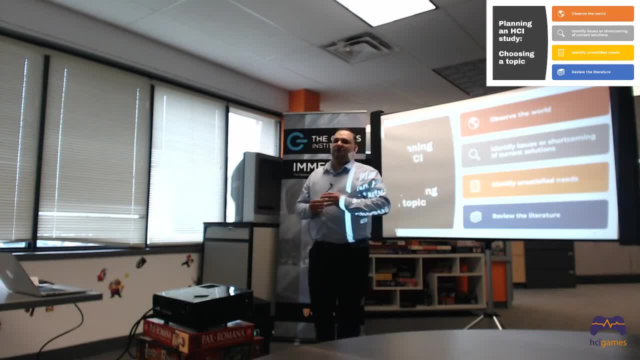 there, because chances are as well that, even though people asked that question before, they don't have a final solution to that problem yet, And that's the very old problem that people have studied over and over. Most of the newer problems have somebody. 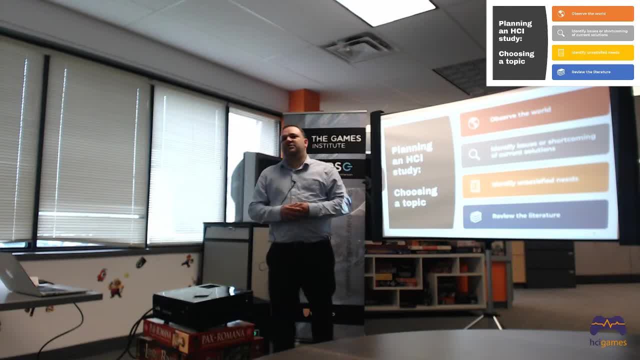 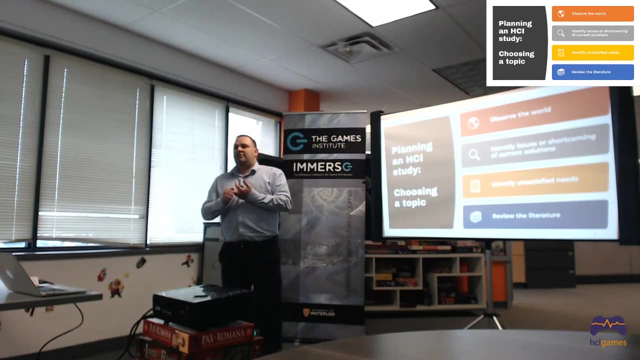 asking questions about it in some initial studies, but with still problems to solve. So I would say: review the literature also comes- before choosing a topic for your study, Because you need to have that idea about what people have asked before and what solutions are they still missing? 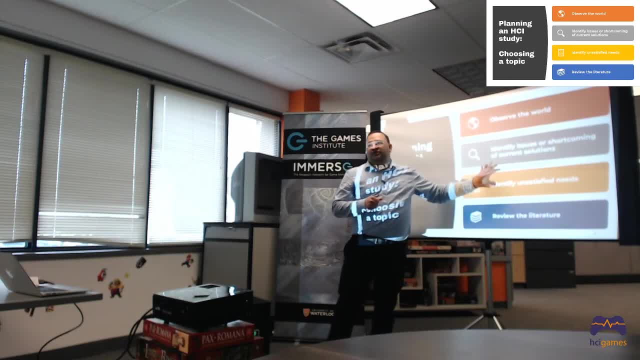 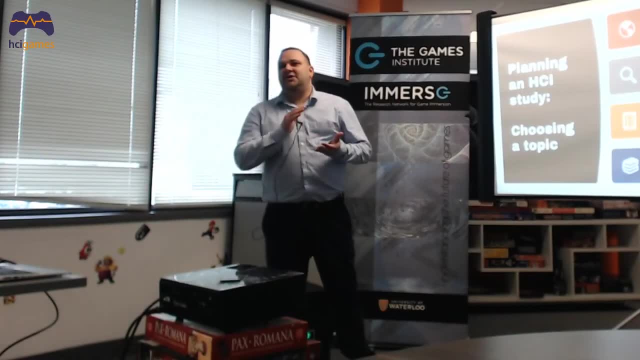 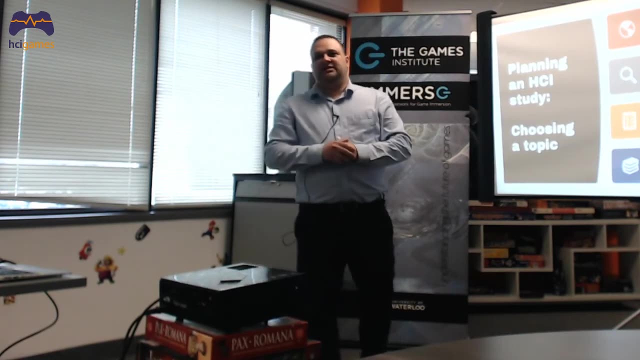 And that is also related with identifying issues or shortcomings of existing research, identifying needs. So if you go to the literature to identify people have tried that but in the end they said that their solution was not perfect because of this or they said that for future work. 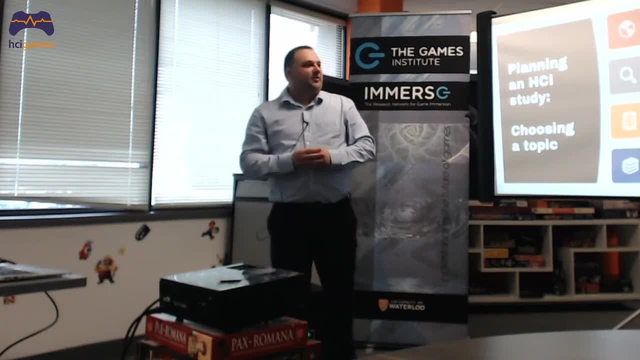 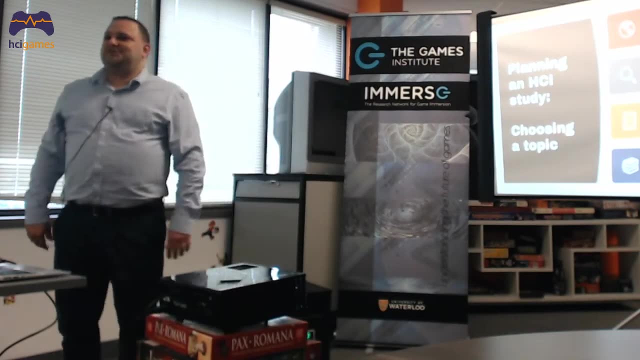 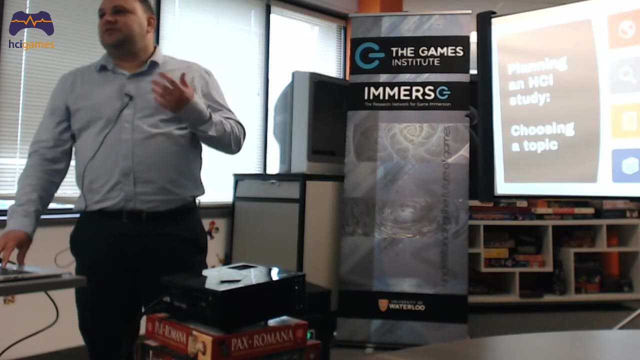 somebody should do that. Those are all good ideas for research topics, So there are many ways of choosing a research topic. maybe what's going to work for you is something different, but it's just some- just from my experience- some of the things that might help you when you are deciding. 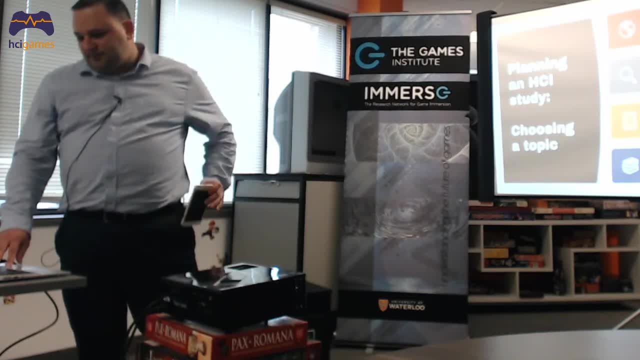 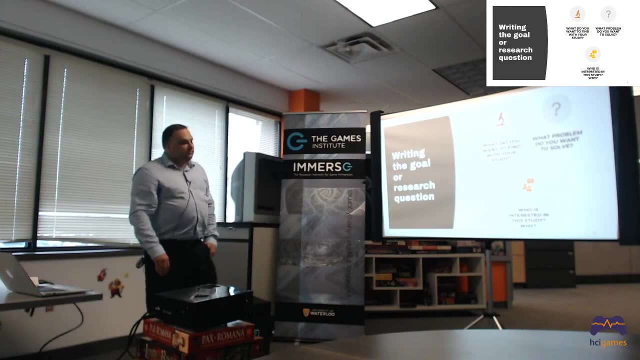 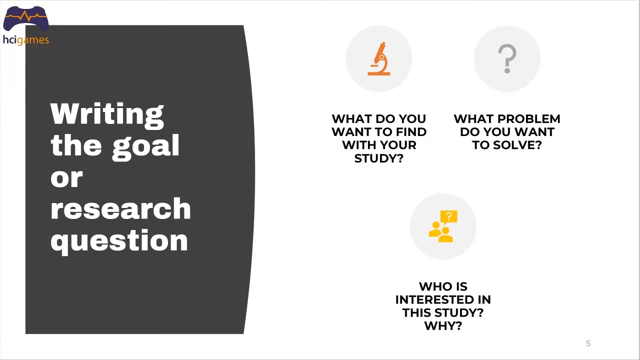 exactly what your studies are going to be about. So now, after you decide what you're going to study, probably your next step should be to write what is your goal in a research question. For my first studies I didn't pay much attention to. 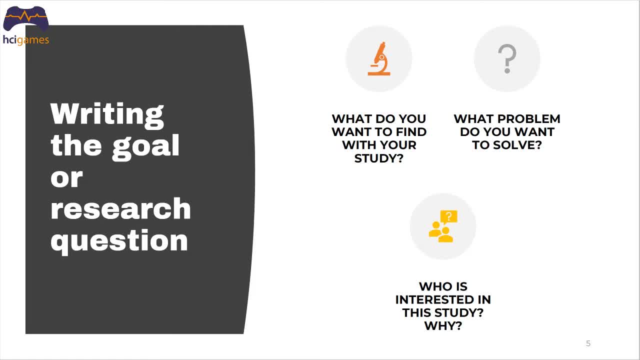 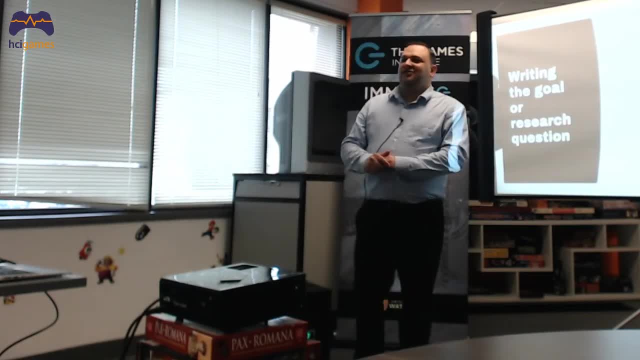 I was excited to just nice. I have a topic. Let's begin studying it, collecting data, drawing conclusions. Then later it's really difficult to explain what you did because you didn't have a clear question in the end. So this was a really interesting topic. 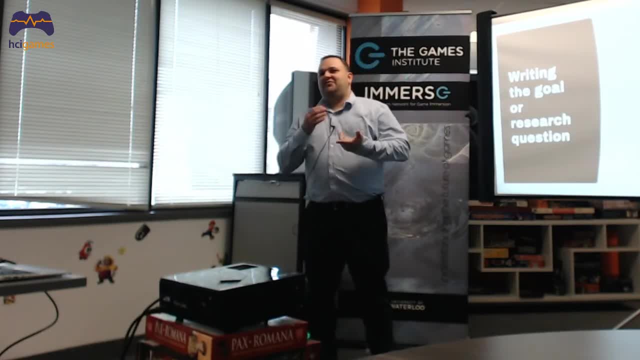 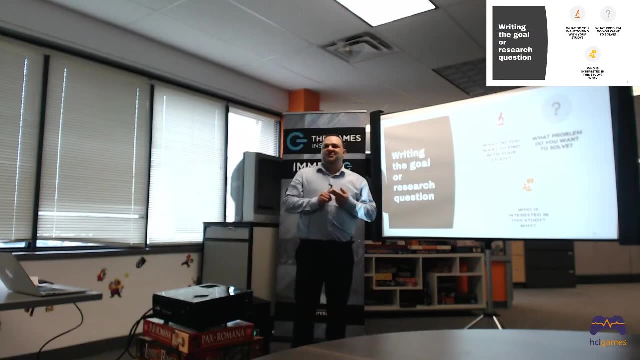 Do you have any questions? No, OK, Yeah. Yeah, you might have a lot of data, even a lot of conclusions from your data, But if you didn't know exactly what you were answering, those conclusions might not answer any clear question, right? 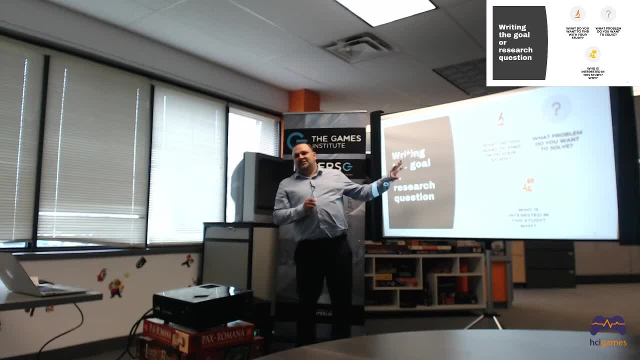 So then I learned that this should essentially be one of the first steps, right? You know exactly what you decide, what your topic is now decide, exactly what you want to answer, right? So some of those things that can help you think about your goal or your research questions. 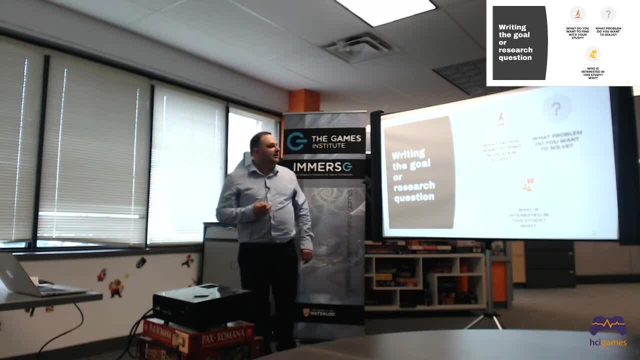 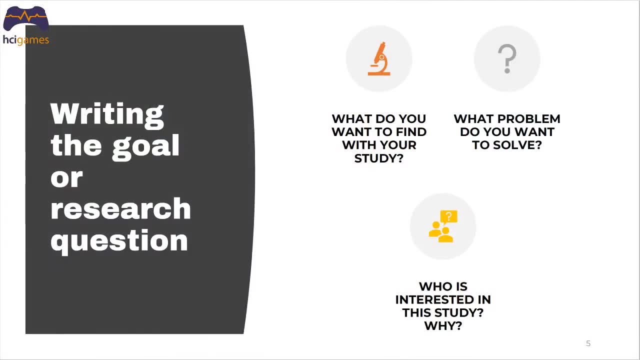 What do you want to find, What problem do you want to solve And also, why are you solving that problem? Who is going to be interested in your solution And what I said here? goal or research question? usually you have a research question, but not all projects are about answering questions. 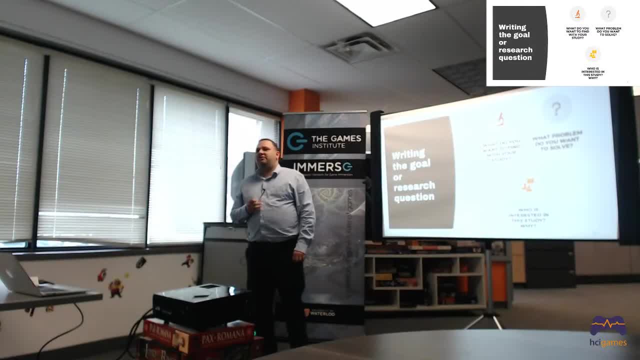 For example, one of my projects had a goal of developing and testing user-type survey for identification. I didn't really have a research question, but I had a goal of developing a user-type survey, So you will have one of them. We're going to think about these things, right. 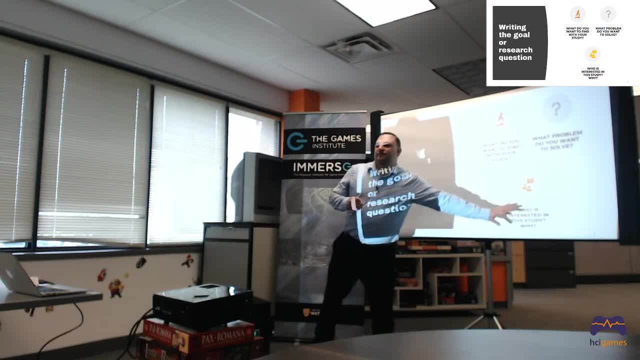 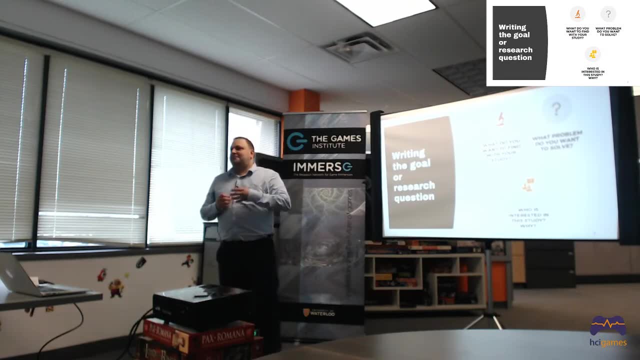 And not only what, but why are you solving that problem is also very helpful, And I've been taught about that even in some of the lab meetings. In theory, any research that produces new knowledge should be interesting, Even if you don't have a clear idea exactly why that is important and who is going to use it. 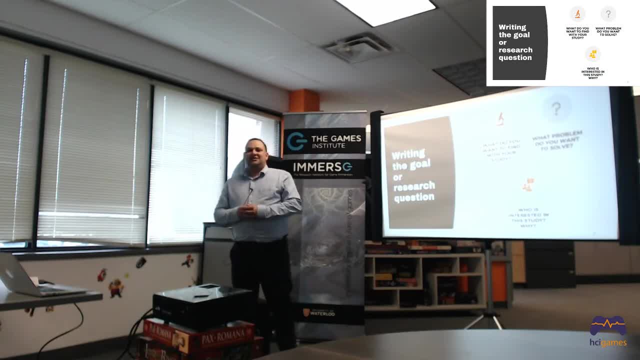 it produces new knowledge. It might be interesting to somebody. In theory, you could put the results out there and maybe somebody is going to find a way to use the results, And that is true. However, if you want to publish your research in the most competitive conferences and journals, 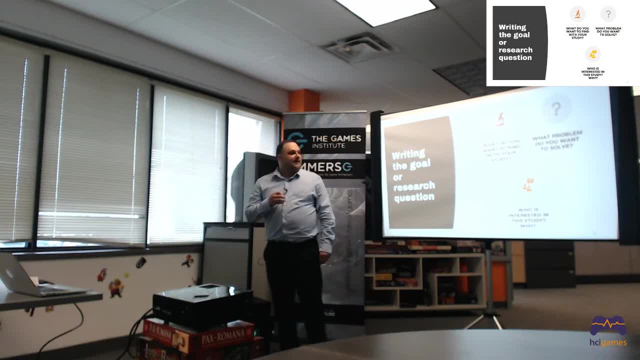 that is going to be difficult if you don't have a clear idea of who is going to use it. in the last application, That's the thing we see in reviews and I have received reviews like that. Maybe you did as well. like well, you did a good study. 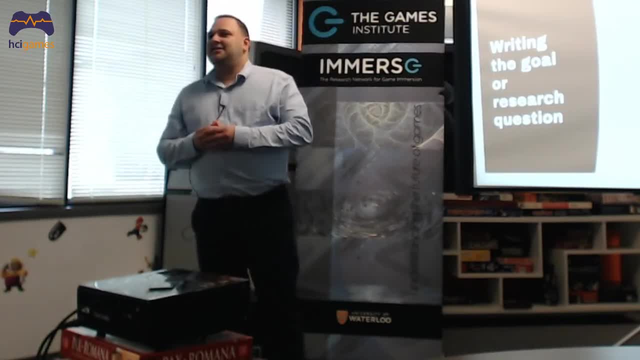 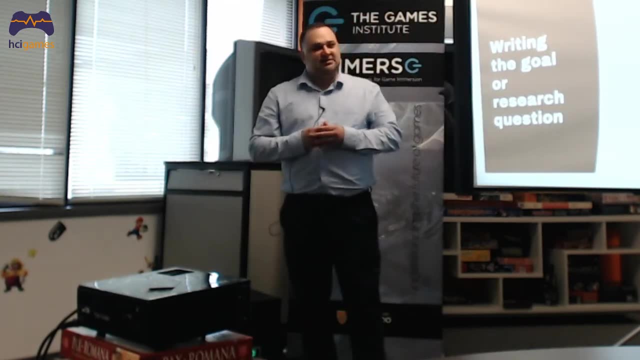 but you didn't clearly say who is interested in your study, What's the application, How that's going to be used. And that's because, well, it's just competitions for those spots, right? The conferences have a limited amount of days. 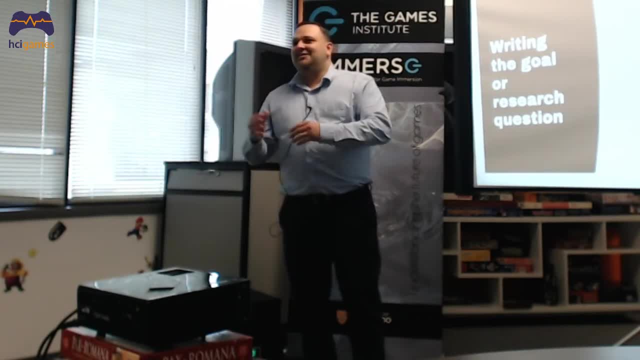 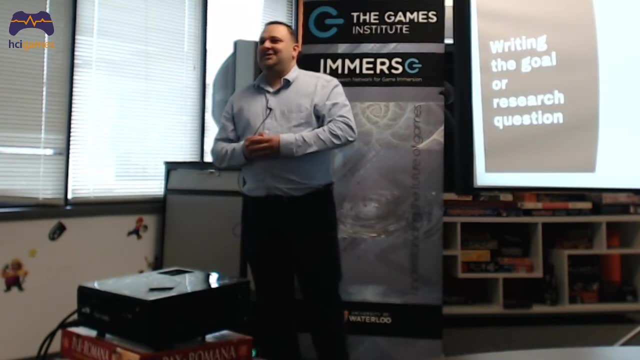 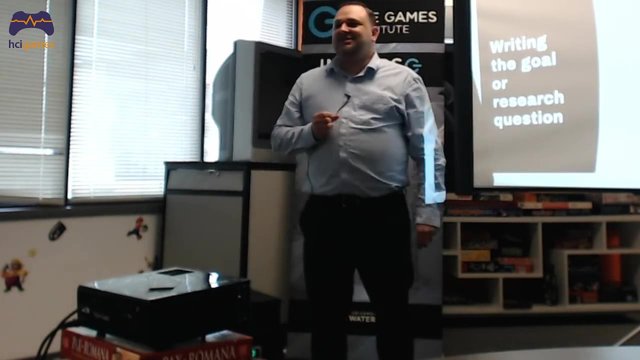 and you can only fit so many presentations in those days. I just went through this with the Far-Kite play just last week because we have lots of missions and we were trying to fit the maximum number of presentations that we could in those three conference days so we could accept more papers. 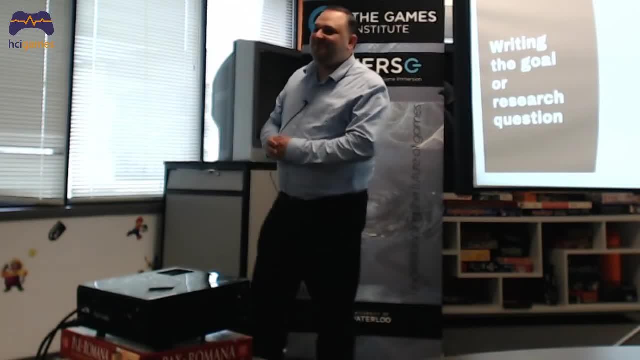 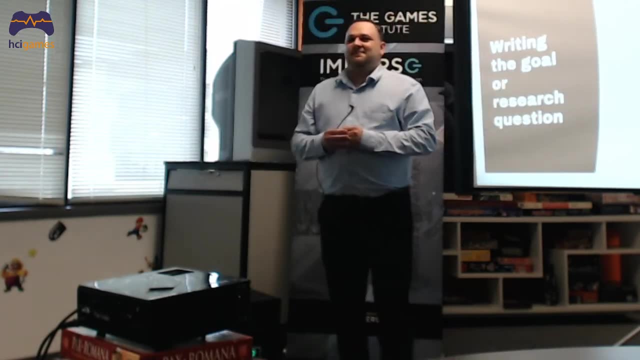 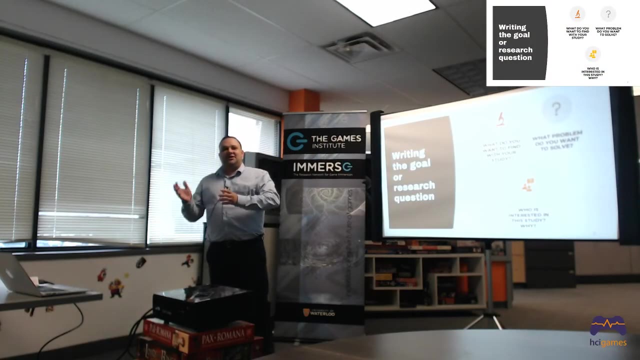 But in the end it's just: you cannot fit more papers And in the end, if people have to decide between two good studies, one of them does explain why people should be interested in those results and who can use them, And the other one is also a good study well done. 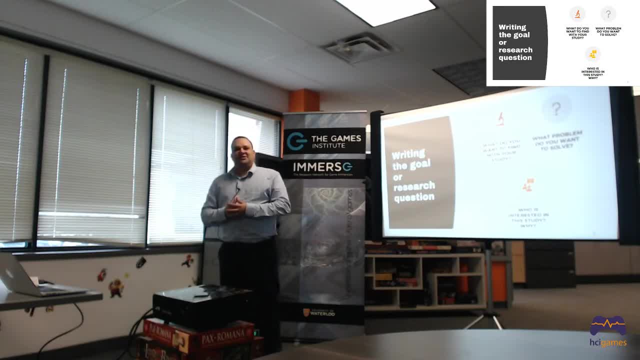 but it doesn't include an explanation. I imagine you are the person who is selecting papers for the conference and you can only select one of them. You're going to select the paper that's good and that explains why it's important, right? 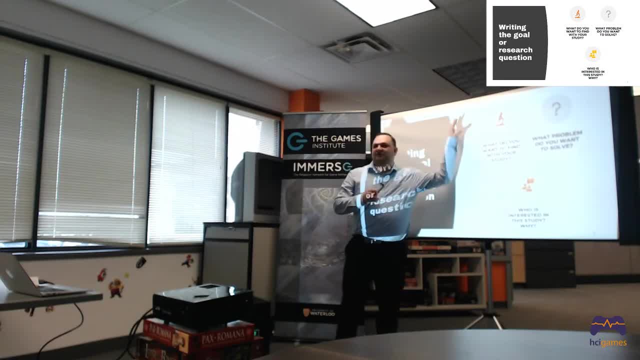 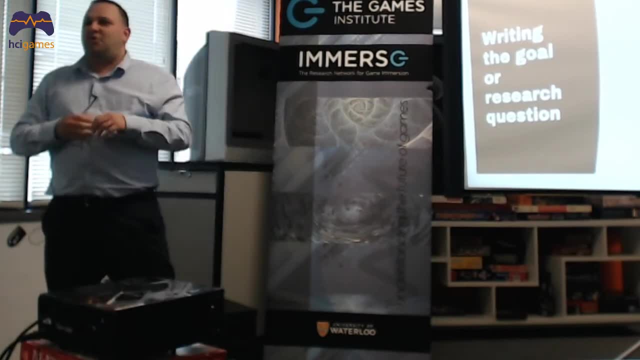 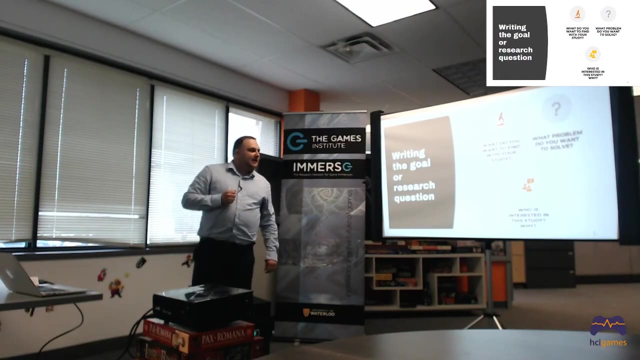 So if you do that in the beginning when you are planning your study, it will be easier later when you write the paper and you'll have more chance of being accepted in this competitive conference as well. if you can explain why it's important, 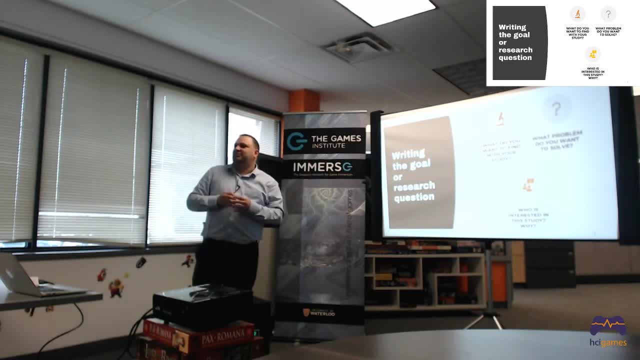 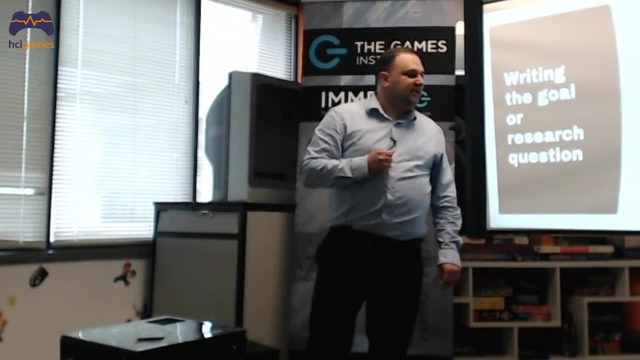 Not that you cannot categorize the publish. If you don't have that, it's just going to be harder to do. You're probably going to have to publish somewhere else, right? That happened with one of my papers, for example. It was a result of a grad course that I took. 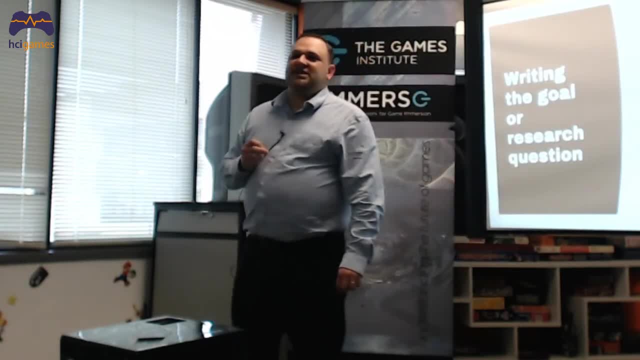 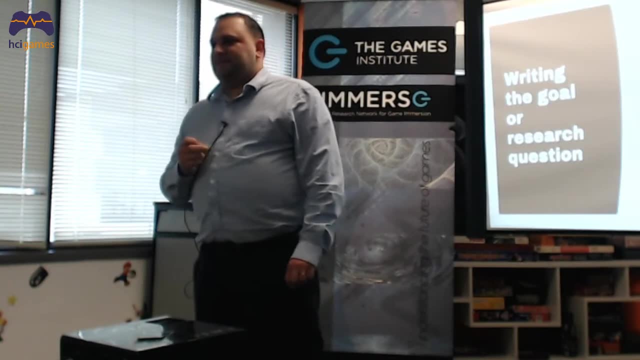 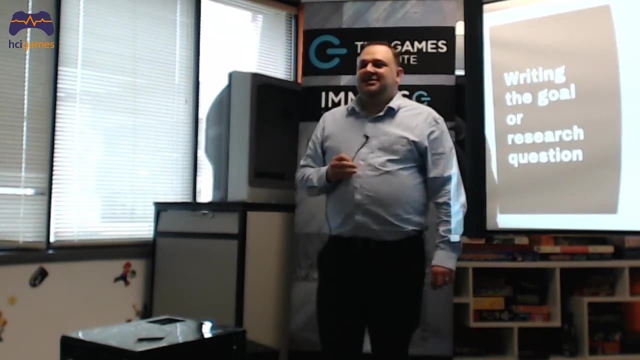 and I used a literature review and proposed the idea of creating recommender systems for again for applications, But I didn't actually implement the idea. The course finished and all I had was the idea right, So it was hard to justify. 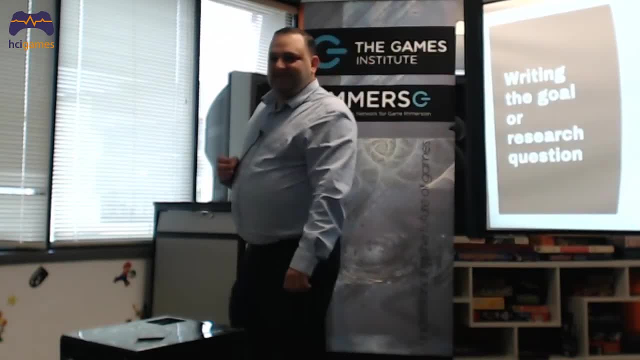 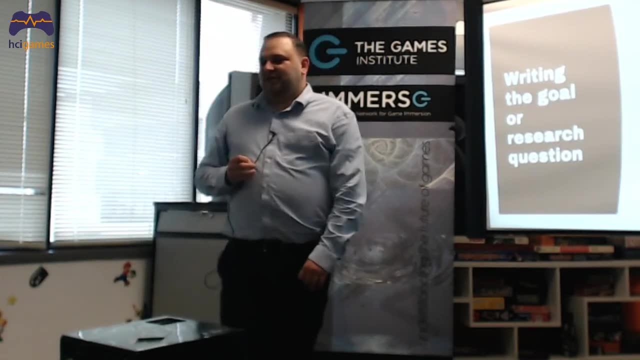 who is going to apply, Since I just have the idea, I don't actually have an application that somebody can use. And that's what happened. That paper was not accepted as a full paper because that's what people said. Well, it works just right here from now on. 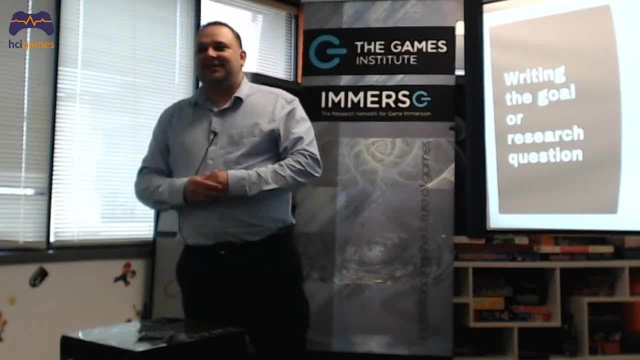 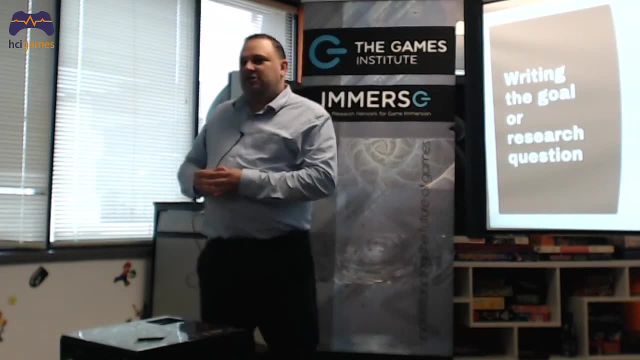 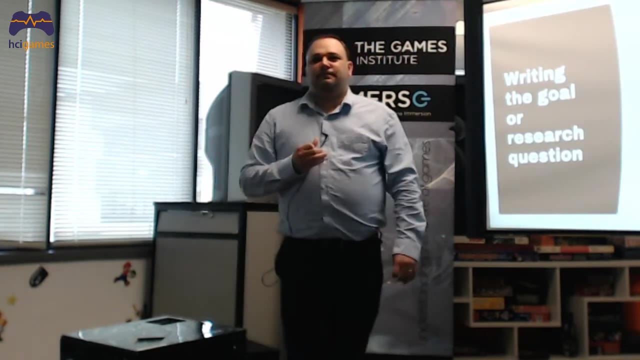 If you had the system then maybe we could accept it, but not now. And then I ended up publishing that paper just with the idea on a workshop, which is just. I think you're familiar already, but usually a lot of these conferences that we go. 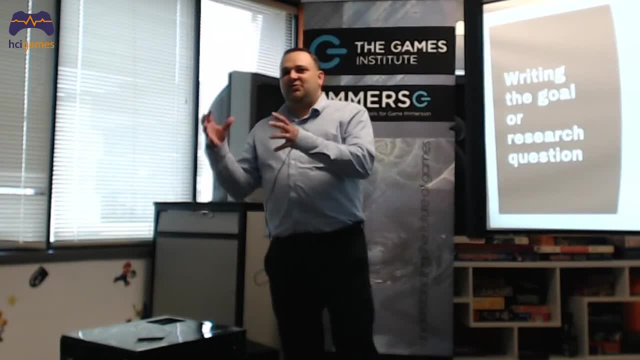 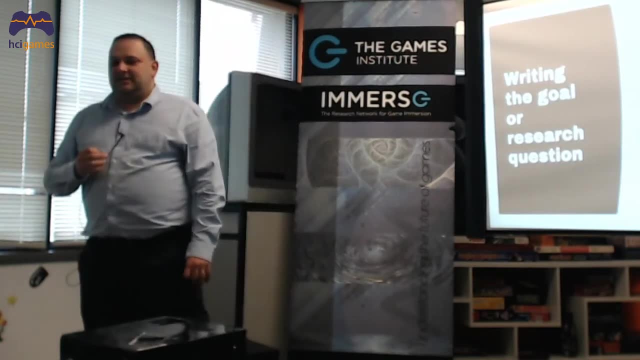 have workshops that they for the conference, where people just meet in smaller groups to discuss a topic that's maybe not so mature yet or something like that. so I published that. It was still a good publication. People are reading and citing it. 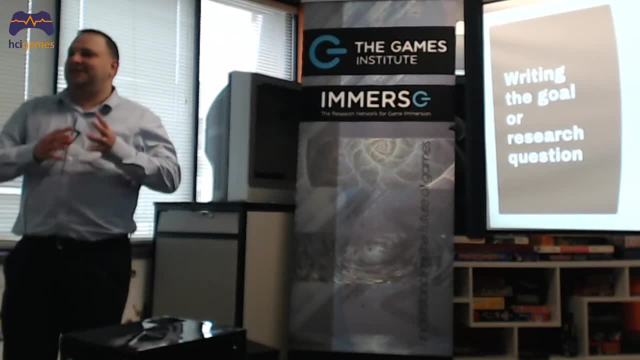 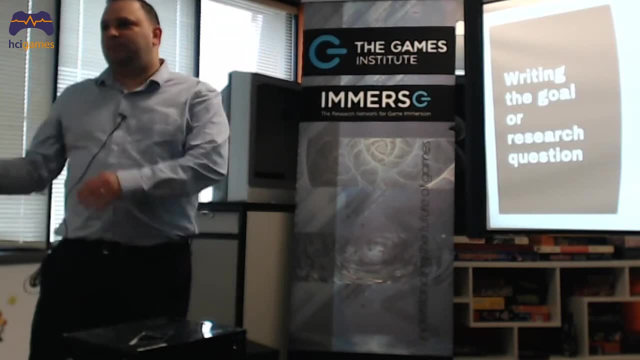 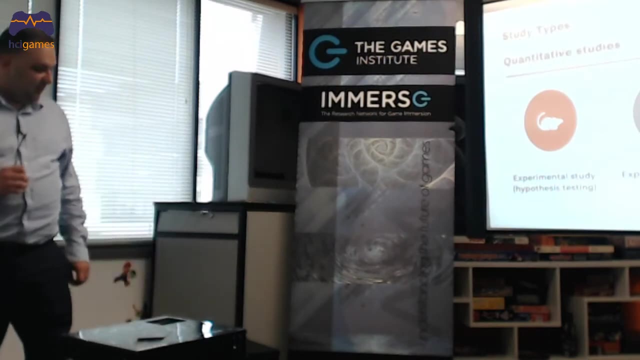 and happy with it, But, just as I said, by not having a clear explanation of how people could apply that, it's hard to get greater publishing on a conference rather than publishing it on a smaller workshop. Now, okay, after you have your calls. 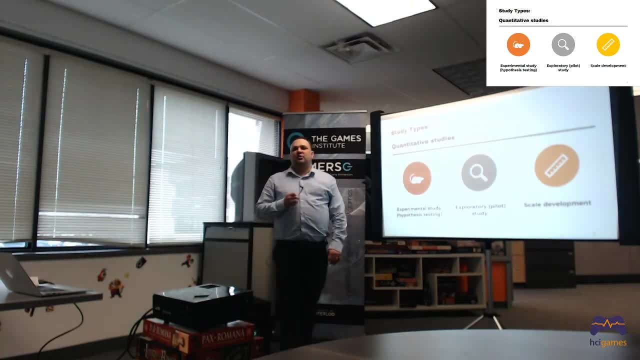 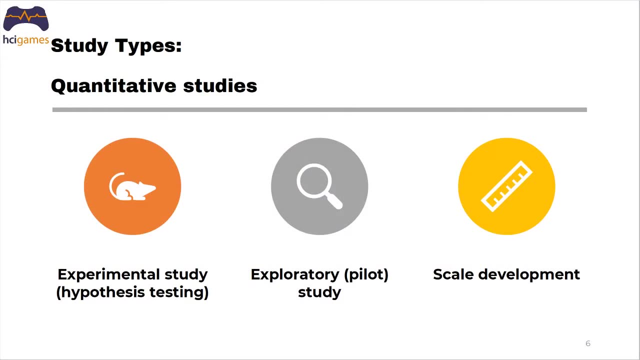 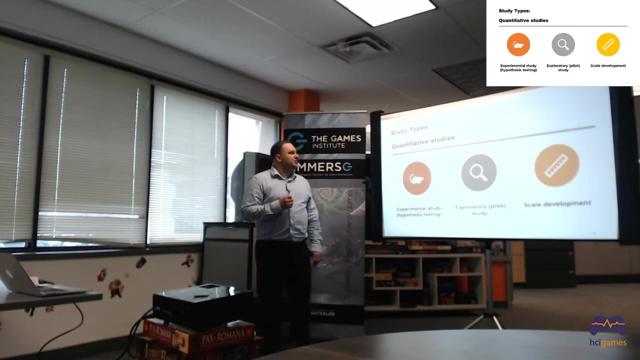 your research questions, you know exactly what problem you want to solve and who is it for. you need to decide what kind of study you're going to do, And we can split studies basically on two groups, so quantitative studies or qualitative studies, or of course, you can also mix studies. 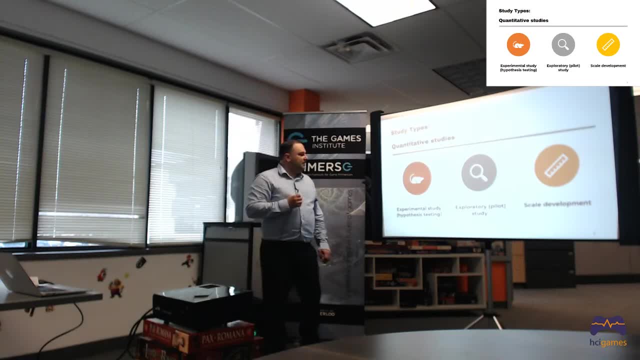 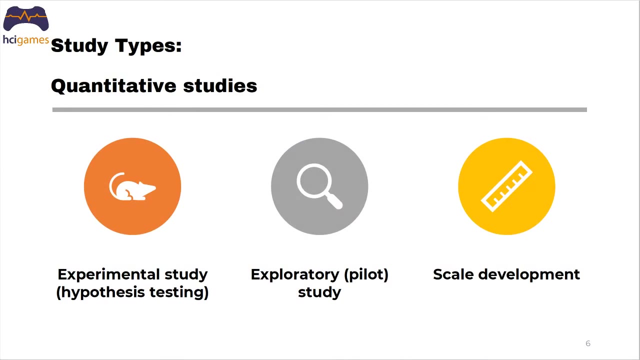 which have both components. Now I didn't formally study research methods and put all the different kinds of studies that exist here for this presentation. so I'm sure there are more types, but I just put here the kinds of study that I've found myself. 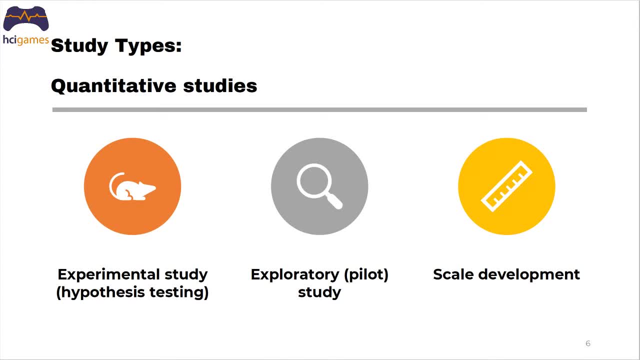 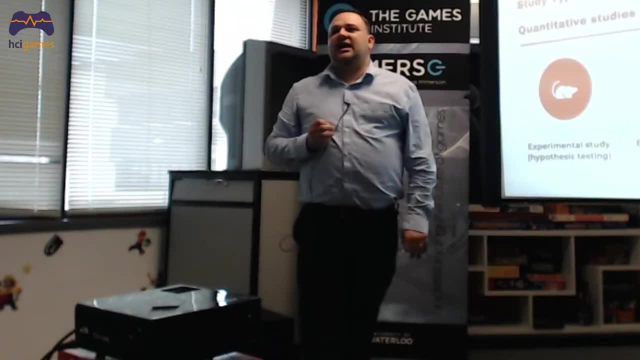 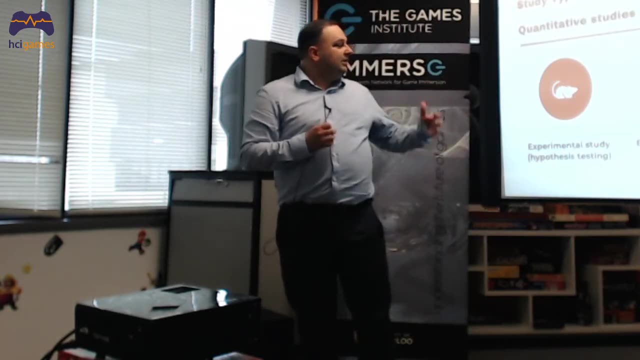 or that. I've seen people do it frequently in the conference that I went and the reviews that I did, So kind of these are common study types for the topics that we work on. I'm sure there are many more study types, But well, okay. 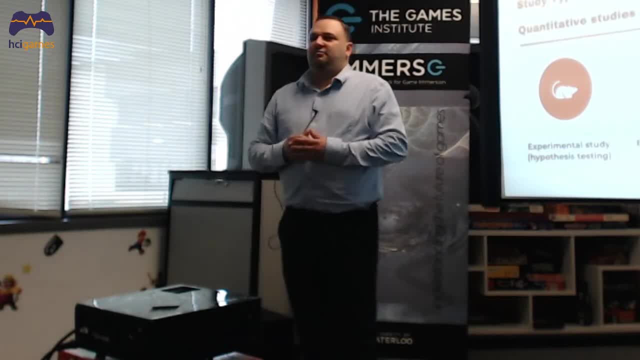 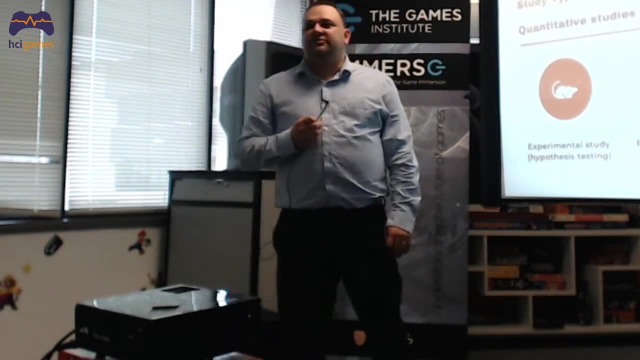 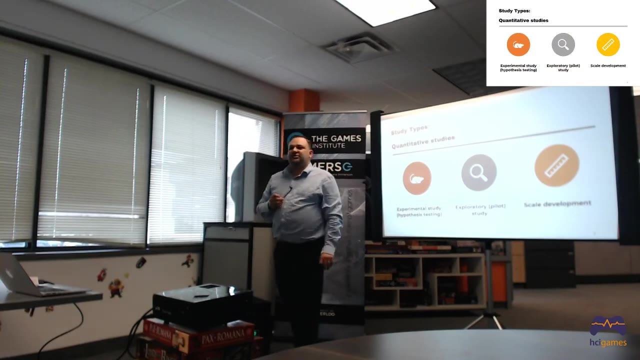 so if you are going to do a quantitative study, so quantitative means basically that you have numbers right. You're probably measuring something and doing some analysis with those numbers and then reaching a conclusion in the end. So probably the most basic common type of study. 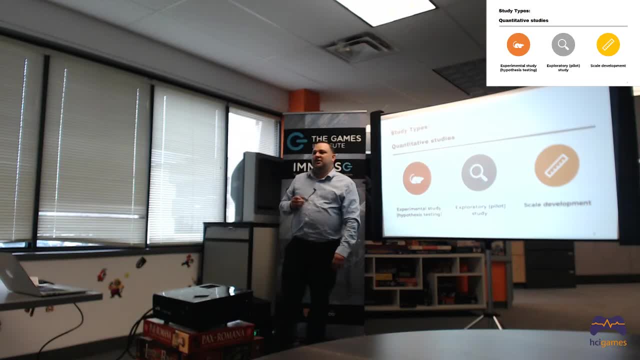 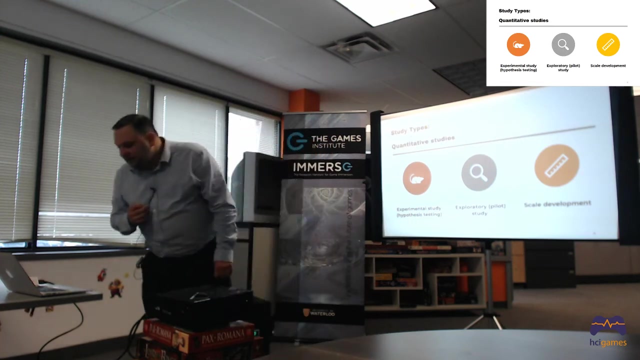 is the experimental study or where you test any hypothesis. So basically you'll have trying to do a research question. you already have an initial hypothesis of what the answer should be and then you test if that hypothesis is true or not. If you 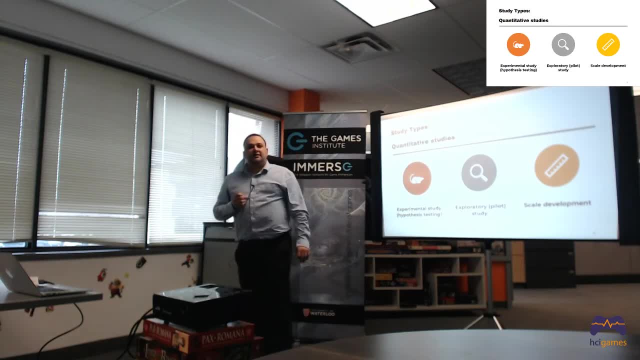 If you do a study this way, If you do a study this way. so planning the hypothesis in advance is also very important. To do a research question, you should plan what your hypothesis is right And that is the right way of doing it. 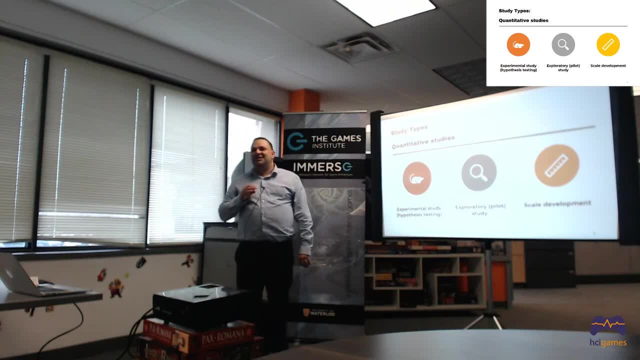 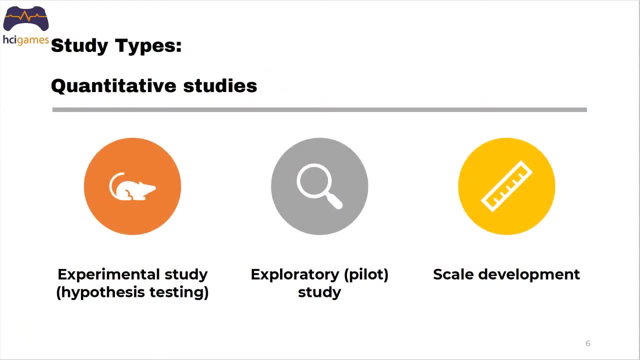 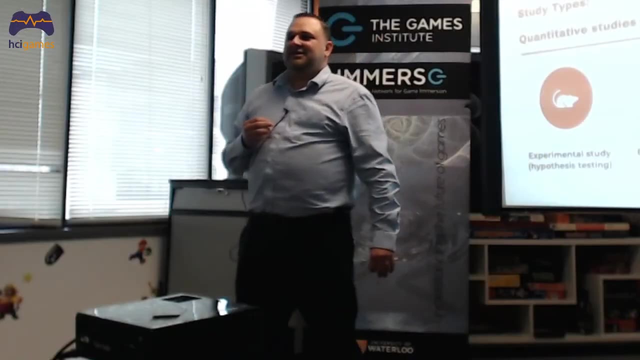 I was a bit negligent with that in the first thesis so I hope I'm very careful. The right way of testing the hypothesis is you think about the hypothesis before you run the study. Then you collect data and you do your statistical analysis and you test if the hypothesis is true or not. 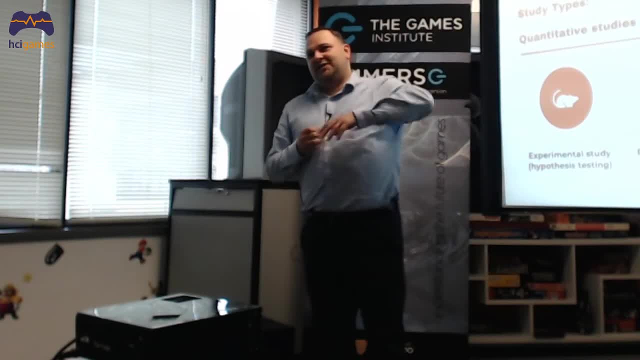 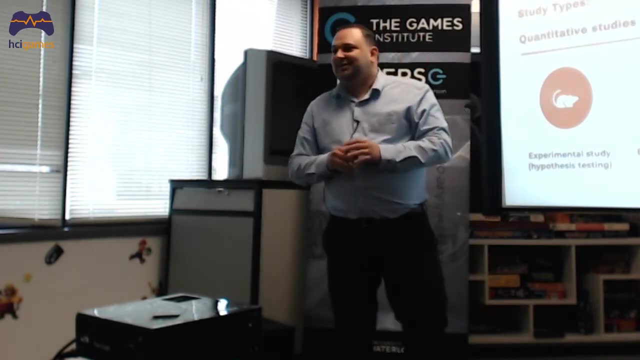 If you don't have a hypothesis before, you collect a bunch of data, you check the results and then you write your hypothesis based on your results. That's kind of cheating, because now you're not testing anything, you're just kind of. 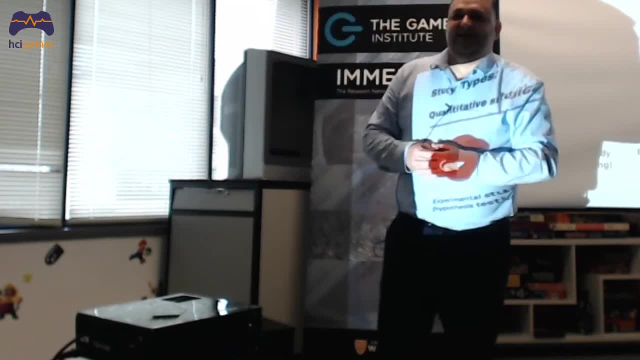 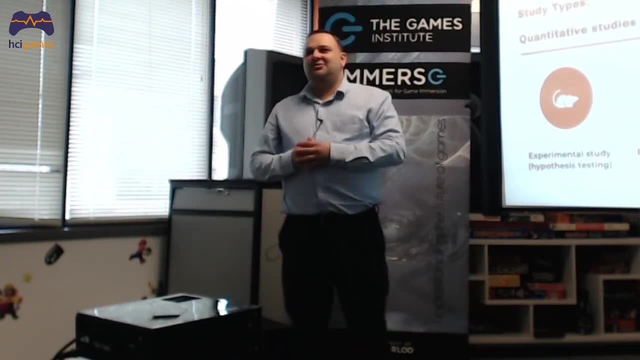 saying that your results are what they are. I'm not going to go into details because we don't have time, but if somebody wants to discuss why that's not the right way to do it, we can discuss that later. But what I want to bring here is that 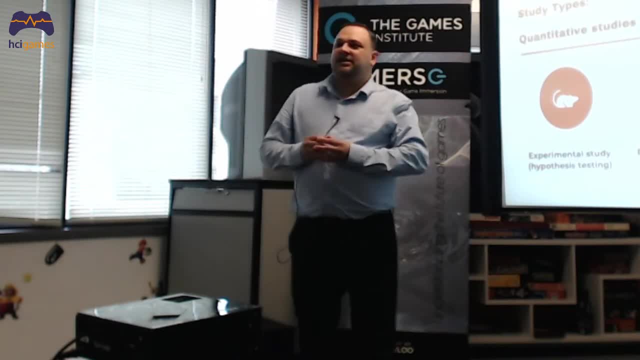 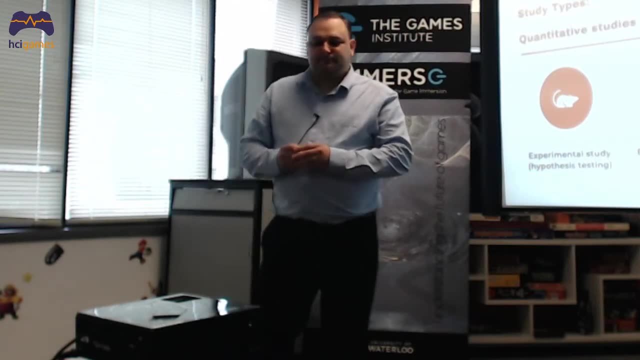 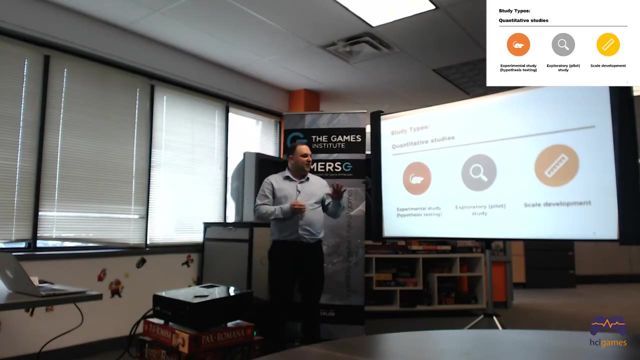 well, the right way to do it is you should think about what the hypothesis are before you actually do the study, And really the hypothesis should be based on some theory or some justification, not just because I think so. So it might be based on some theory. 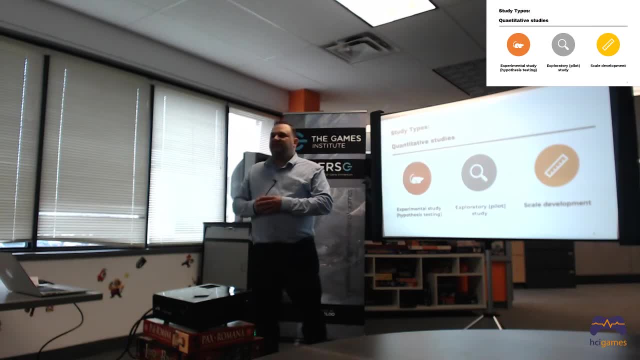 that you already have or some evidence from previous literature. So say, for example, I'm going to test again with and without sound and measure immersion, and I've read the previous literature and people say that sound helps with immersion. right, So I can say that I suppose. 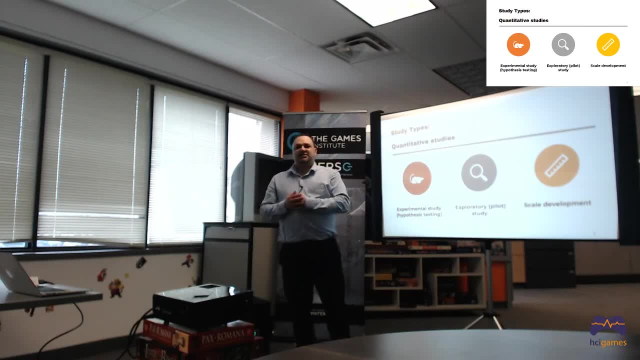 when people play with sound on, they will feel more immersed, because there's past work saying that it's probably not the case. So there, okay, I have previous literature to justify my hypothesis that immersion will be higher with sound than without sound. 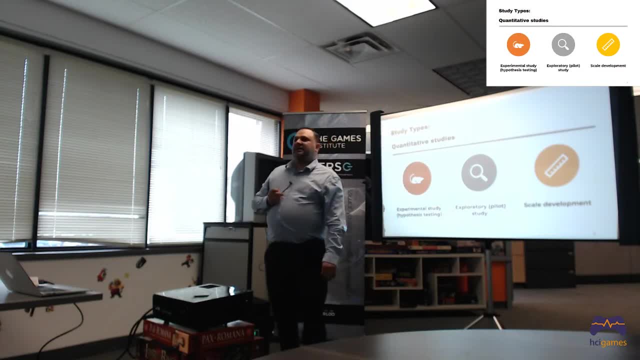 Hypothesis might also come from your design goal. for example, Say, you observe people using virtual reality and you think their controls are too clumsy and you try to design a new type of control that is going to be better. So you have this design goal. 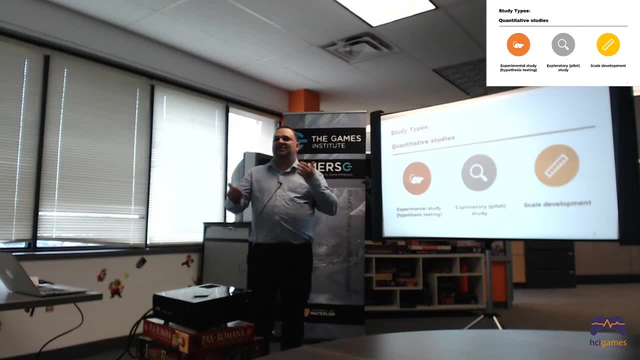 you try to make your control better than what the previous one was before. right, So you can reasonably say that your hypothesis is that your control is going to be better. That's what you're trying to do And, of course, you're going to test it. 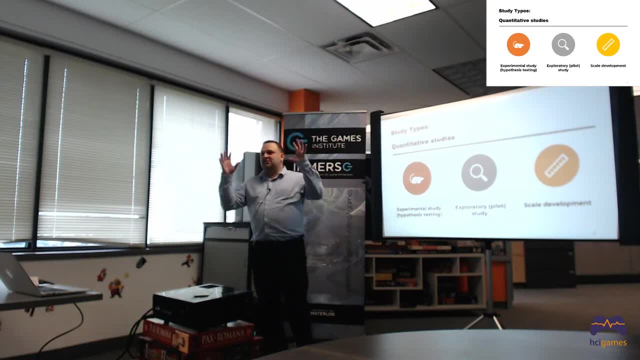 and see if that's the case, right, But what I just want to synthesize here is that what is should come from somewhere. it's not just because it is so, but you should have some reason to justify why your hypothesis are going to be better. 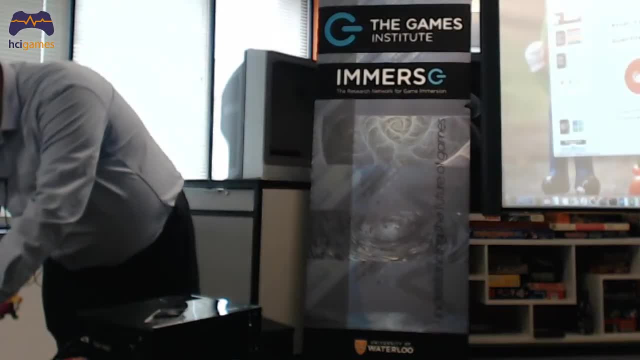 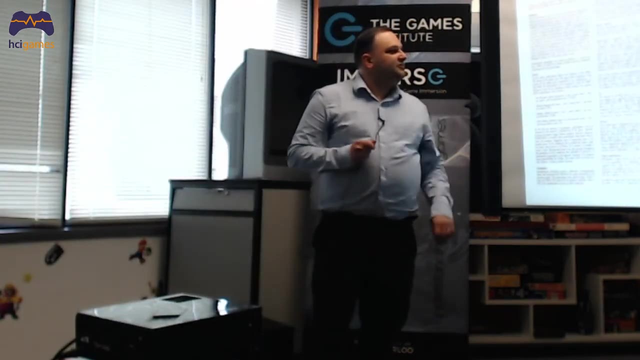 I have some examples open here just to quickly show examples of these different types of papers. So I didn't actually do an experimental study myself yet I'm doing one now. So this is one example that Katia published with some other people here from DJI. 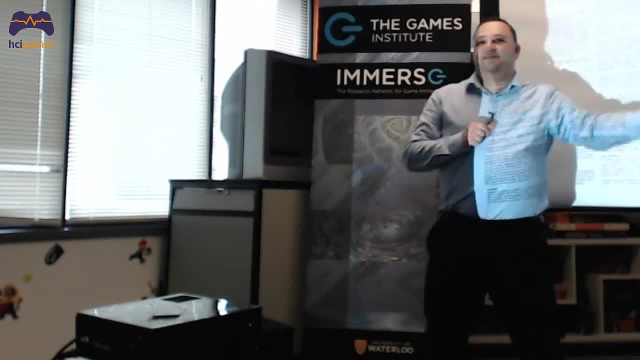 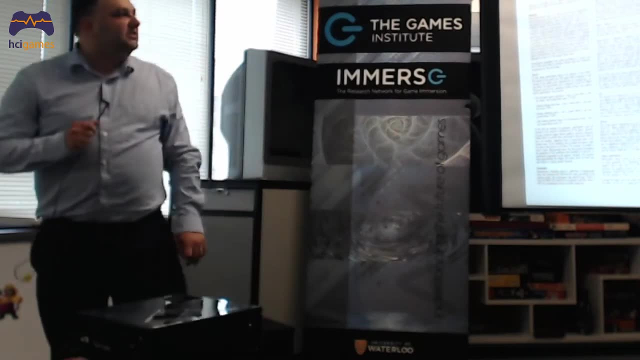 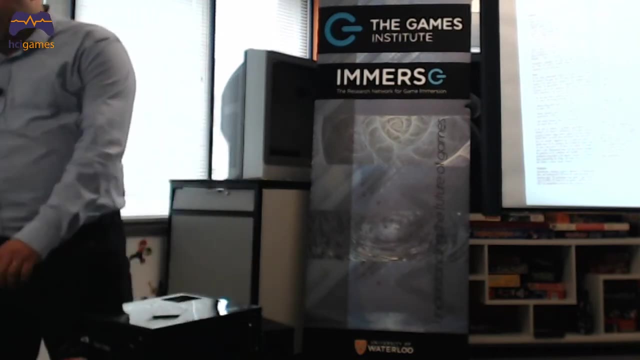 So an experimental study. you might be doing things like that, just comparing some measure throughout different conditions. So I think that was with audio: Some people played with music without music, with sound effects, without sound effects- and then comparing some values between them. 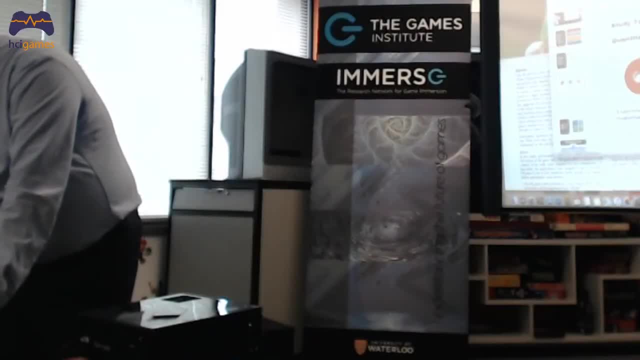 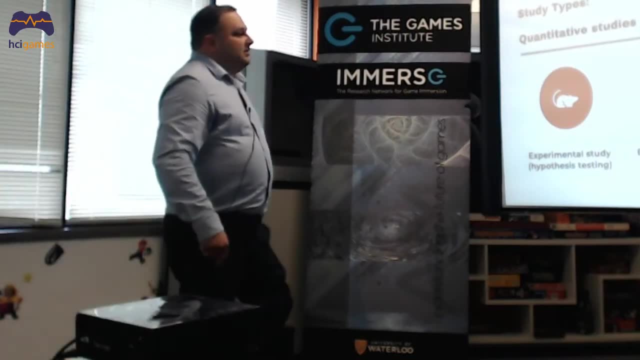 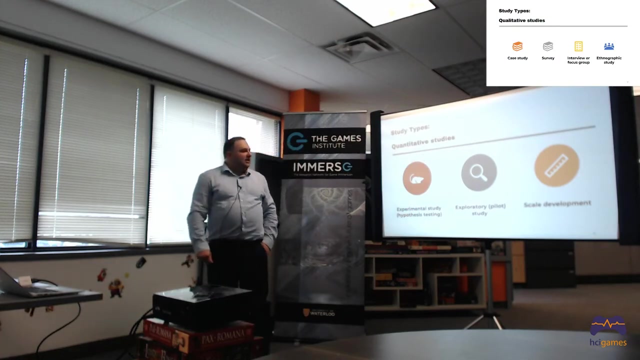 to test the hypothesis. So that could be one type of study experience. So another type of study that I've seen people talking about is kind of exploring something or piloting something. So that might be something you do when you're investigating your question and you don't have yet. 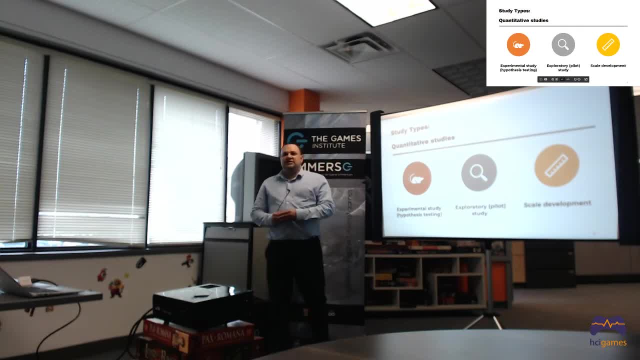 enough knowledge about it to even formulate a hypothesis. So you might be just: hey, let's just collect some data here and see what we get from it. So we're just exploring this space here and seeing what we can find out here, And these are well. 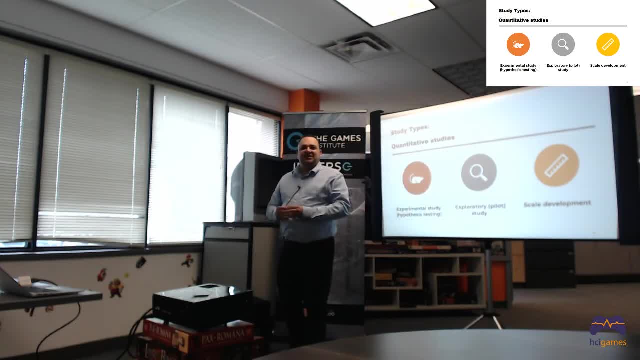 the name exploratory pilot- hints that usually these are initial studies on a topic. right, You're not going to get solid conclusions from this kind of study, but you might get indications of things that might be worth investigating in the future. And another study that 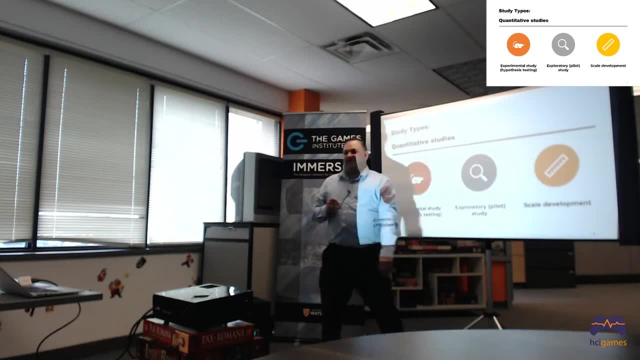 I guess not that common, but I've done this kind of study a lot, so I'll just put it. there is scale development, So I've done a lot of work. that is, creating scales that people can answer and then give you scores about your identification, user type. 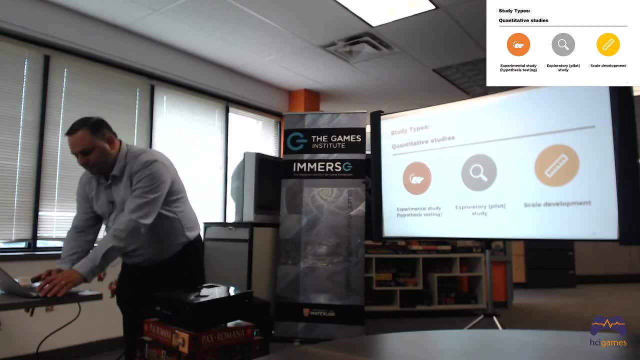 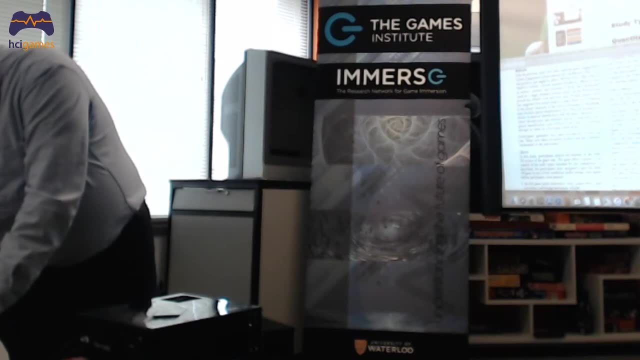 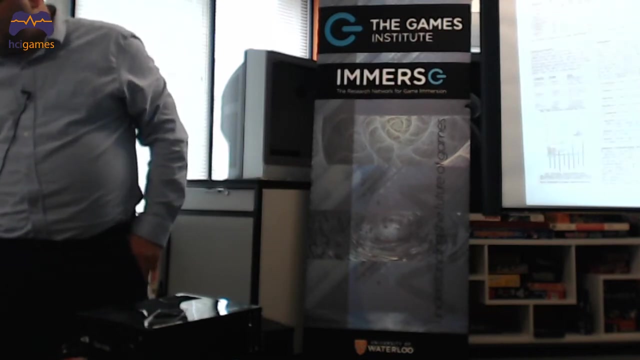 or your player types. So this is basically about creating questions and then evaluating if these questions actually give you the score that they're supposed to give you. So just to bring examples as well here. So what I want to bring is just a quick impression here. 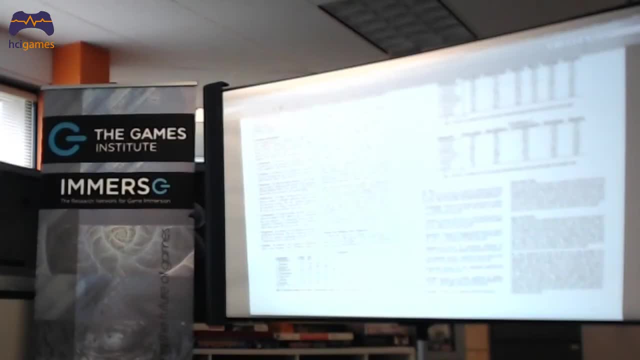 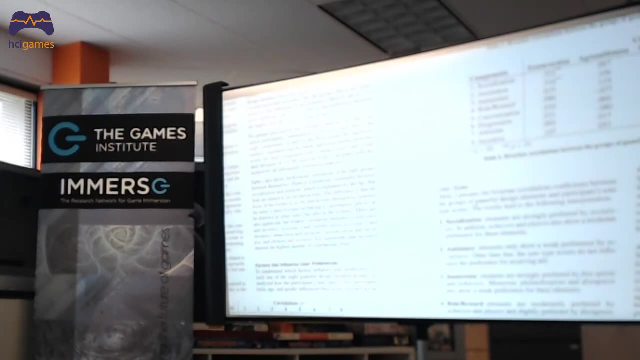 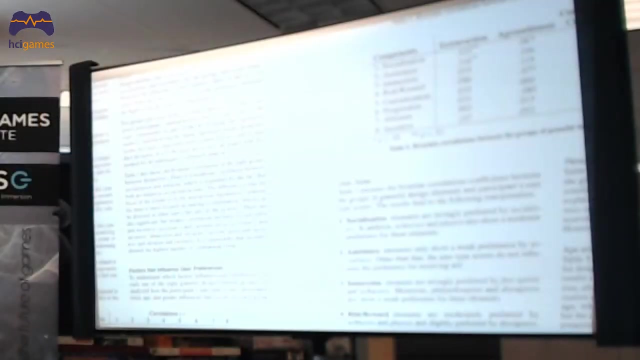 of how these papers might look like, But again, we can have so many different things. Just one example from my papers. So this was an exploratory study. I think the projector and everything is so small you cannot see. Okay, I guess I'll just show this part. 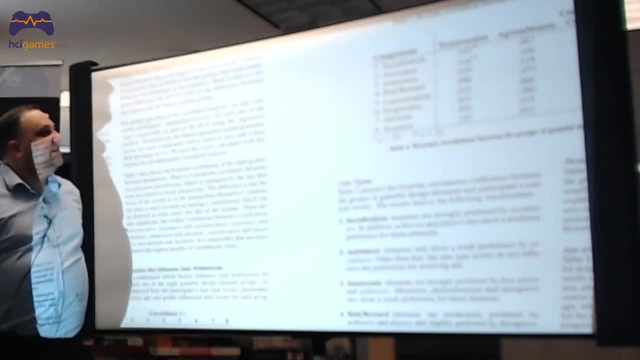 So this was an exploratory study. So we were exploring different types of game elements and different personality traits, for example, to see if people with certain personalities enjoy these kind of game elements more. So we didn't actually have a lot of information beforehand. 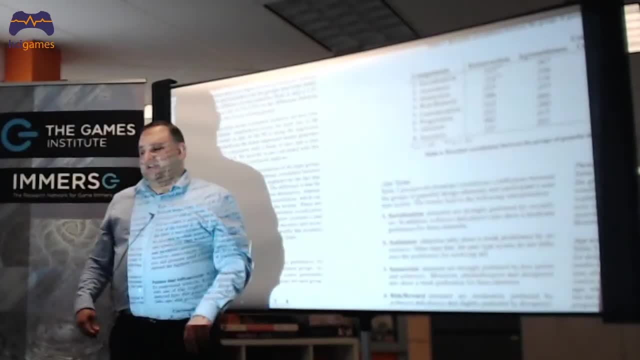 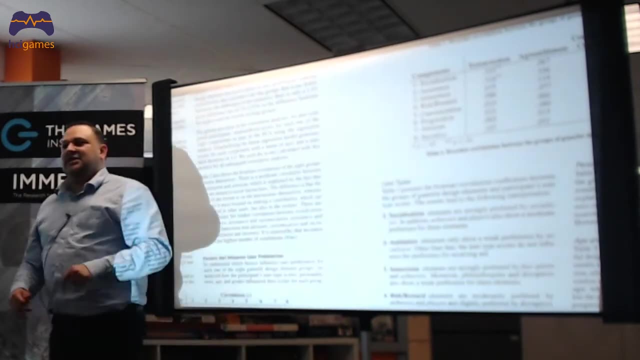 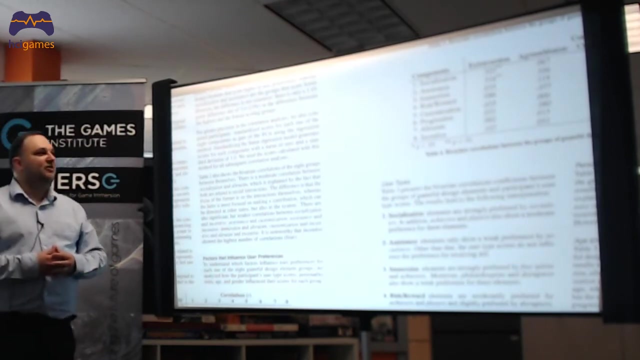 so we were just exploring. So exploratory studies typically have lots of data. like we have different tables in this study, Because then we just There's lots of different things, because we're just exploring, We're just seeing where we find something. 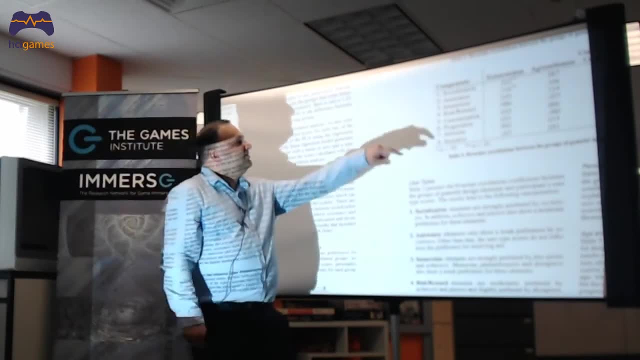 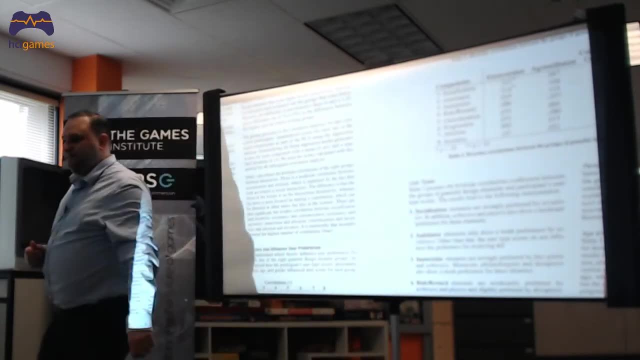 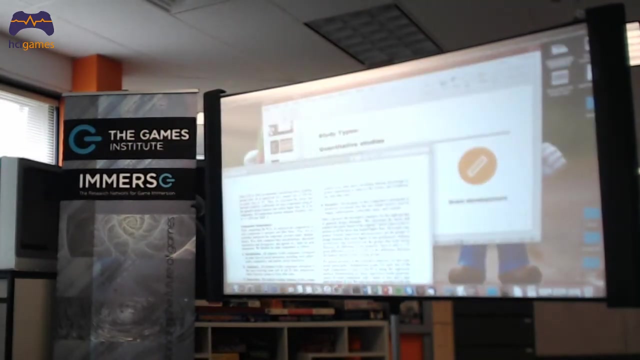 that might be interesting or not, right? So we noticed here that, not surprisingly, people that are more extroverted tend to like more game elements that are referred to social play. So we find things there that might be interesting in our exploration. 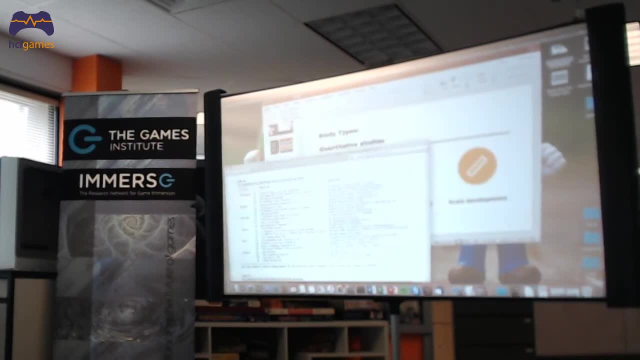 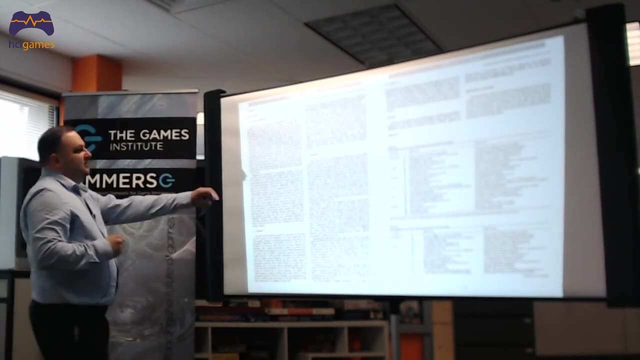 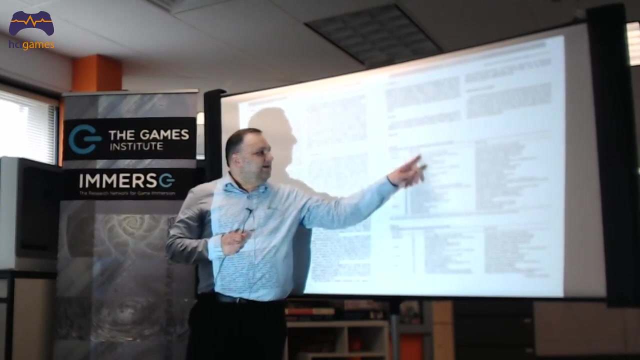 And this other example here is about scale development. So we created a scale here for user types. So this table- I don't want you to read it, but just to see that we have several questions here. So this is a questionnaire that we would give people. 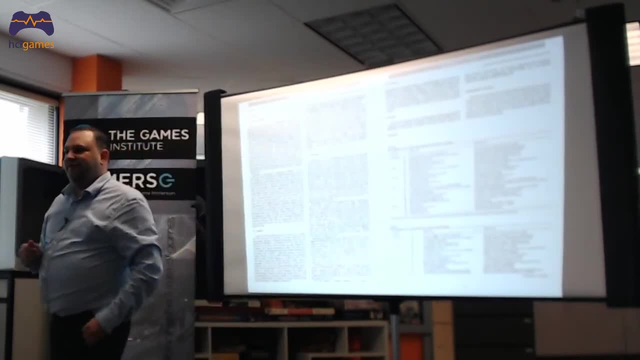 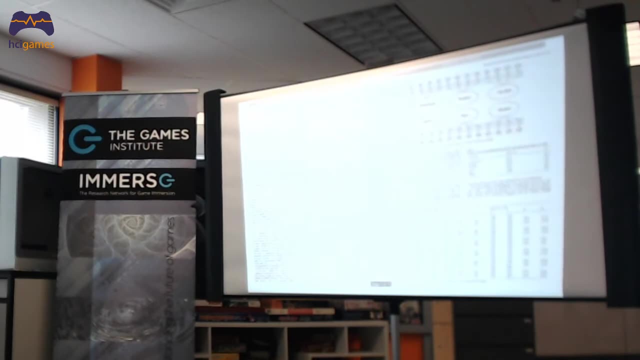 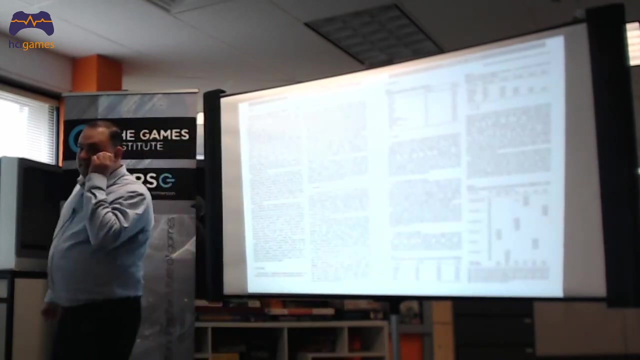 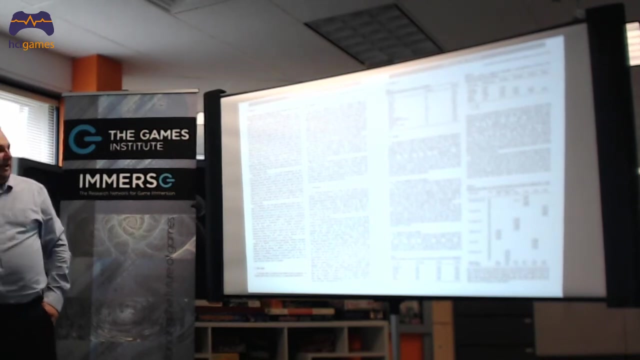 and they would score how much they agree or not with those affirmations right. And then we ask people to answer those questions and we do some statistical analysis to see if people's answers really correspond to the score that we thought should like. I wrote a question that is supposed: 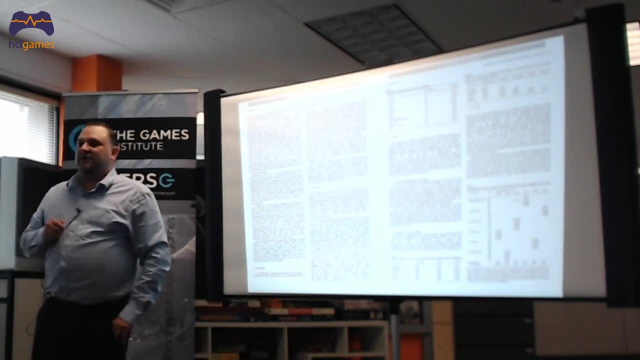 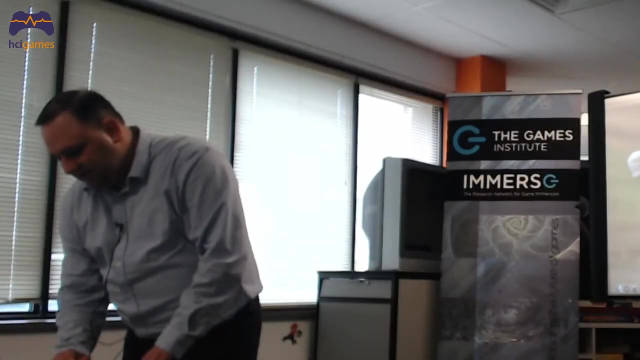 to test people's score on the philanthropist user type, for example, And then I do some statistical testing to see if all the questions that should be related to that user type really are. So if that's the kind of thing that you're doing, 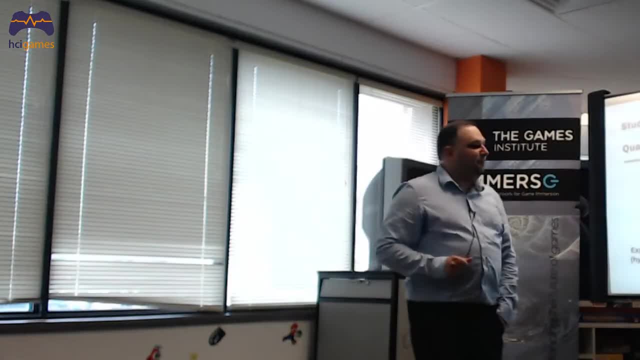 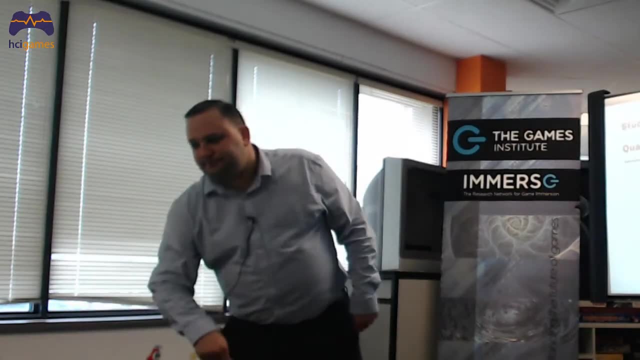 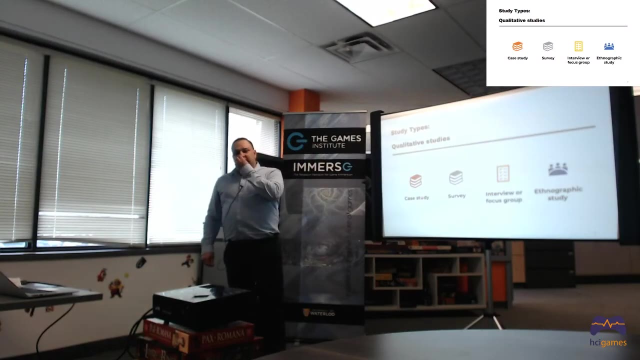 so you're doing a study that is scale development. So Another thing, other type of study that you can do then are qualitative studies. So these happen when you are not measuring things but you are analyzing the quality of things. So this could be. 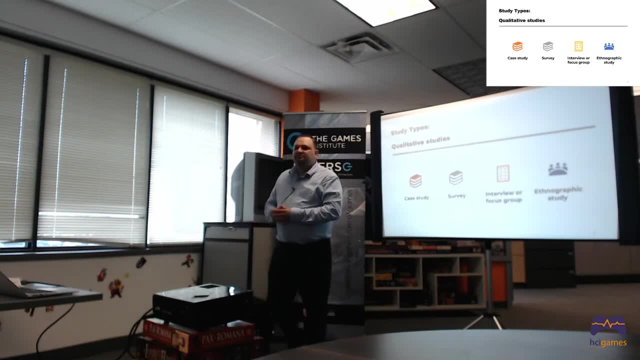 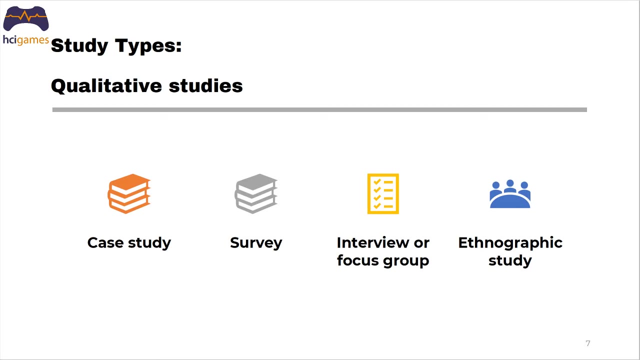 for example, a case study. So you go, you observe one case happening in detail and you try to understand exactly how things are happening, why you talk to people. then that can generate you better insights or something Usually you're going to see. 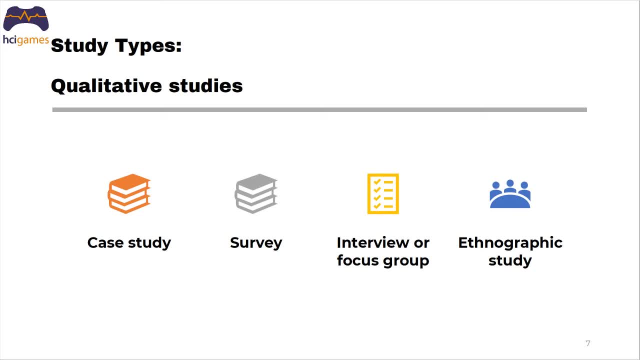 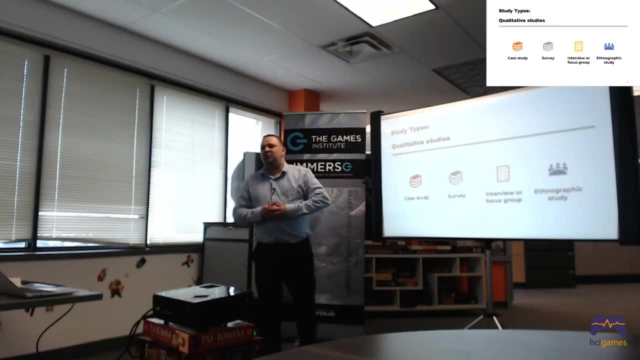 that qualitative studies have this characteristic, While quantitative studies- stereotypes- will give you maybe a yes or no. Yes because it's true or not. They usually don't explain you why. And then qualitative studies usually give you that point, that understanding of 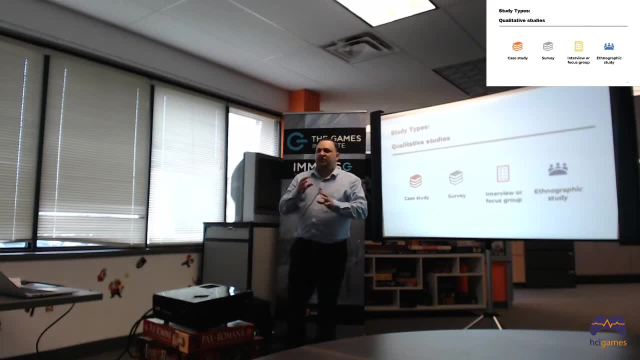 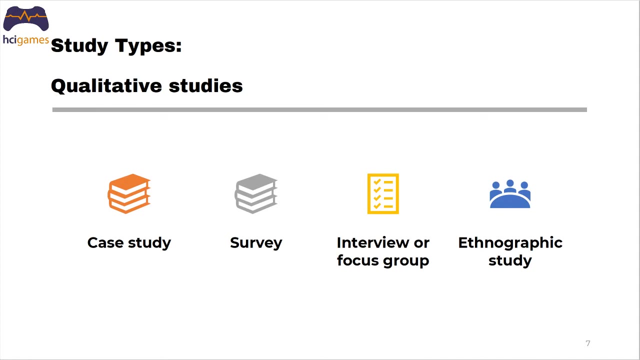 how things are actually happening there, so you can understand the natives, So you can also do surveys. This would be send questions to somebody, But then if it's qualitative, then the answers are not going to be numbers. Maybe they're going to have. 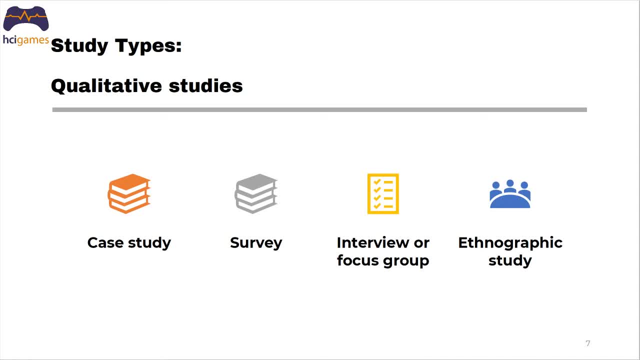 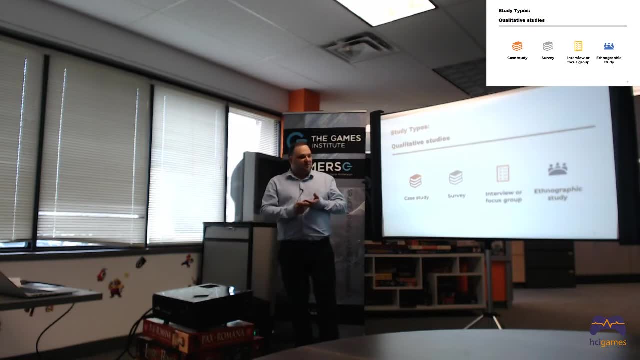 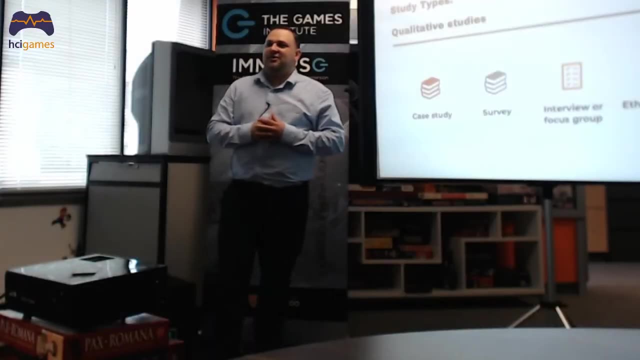 some free text fields there where you let people freely explain something: their impressions about this thing that they used, or why they use the way they do. Any question, people can say something about it, and then you can analyze the answers from different people. 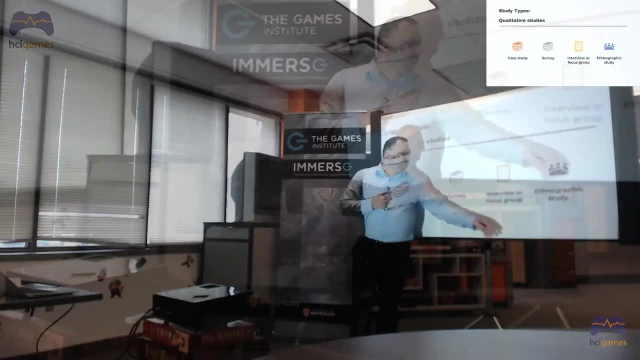 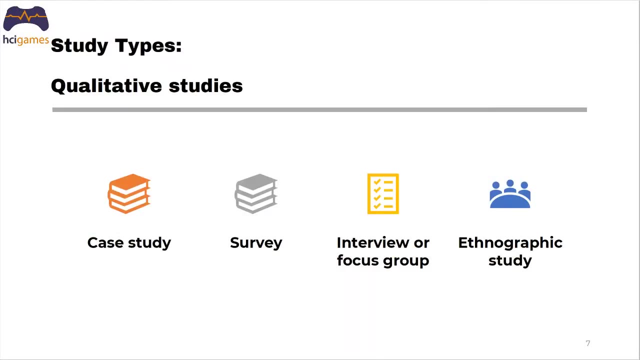 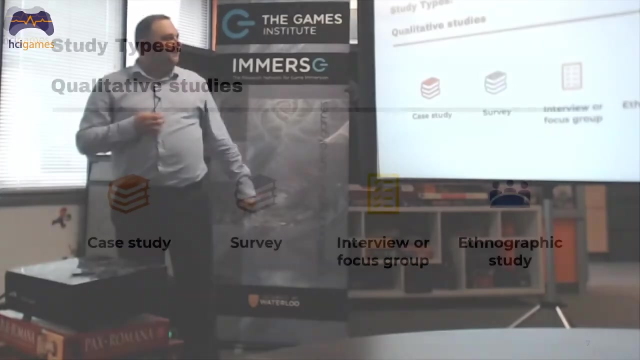 and try to find some patterns there. Interviews or focus groups are similar, but instead of sending the questions like in a survey, then you are interviewing people and asking them about their experiences, about something, their motivation to use the system, things like that. 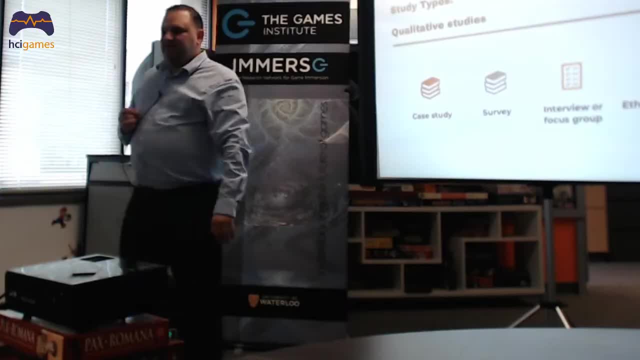 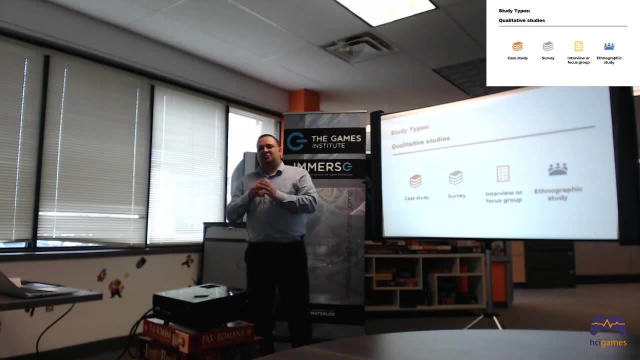 I've seen some ethnographic studies as well, which basically means that you're going to investigate things happening kind of in the real- not only the real world, but they happen naturally in the real world- instead of setting up a lab study. So I've seen an interesting study. 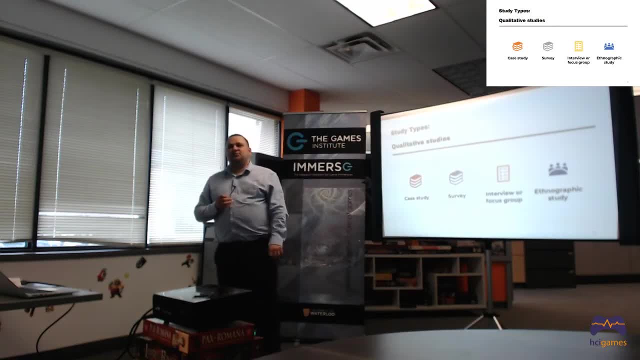 that the researcher spent a lot of time playing World of Warcraft and documenting everything and studying how rewards work on World of Warcraft, how they felt when they used it, when they received rewards and things like that, how he used the rewards. So it's an ethnographic study. 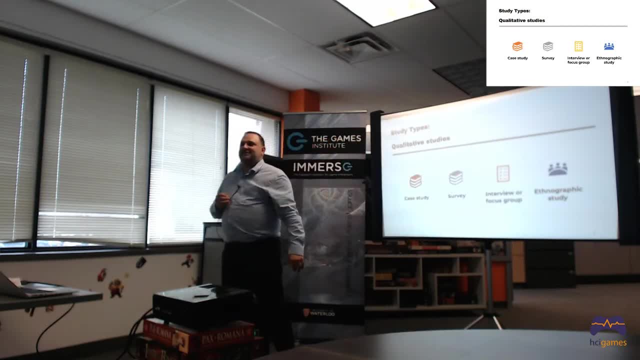 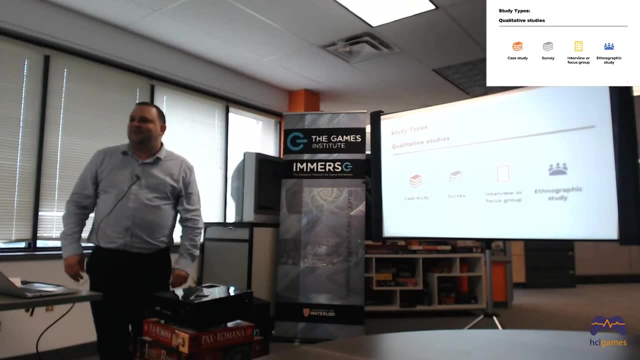 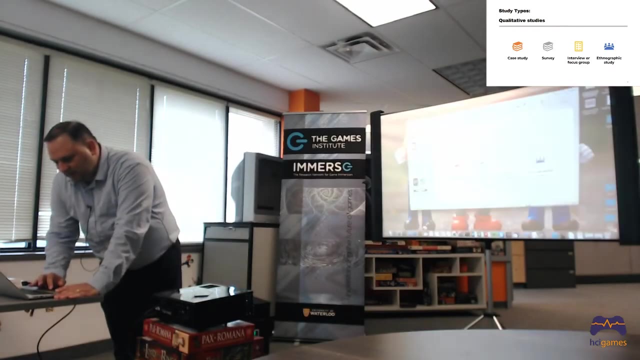 because he was actually going there and playing and documenting and analyzing the experiences. That's an interesting study. right, I have to play World of Warcraft because it's from my study, but it's really interesting And, as I said, while these studies can be mixed, 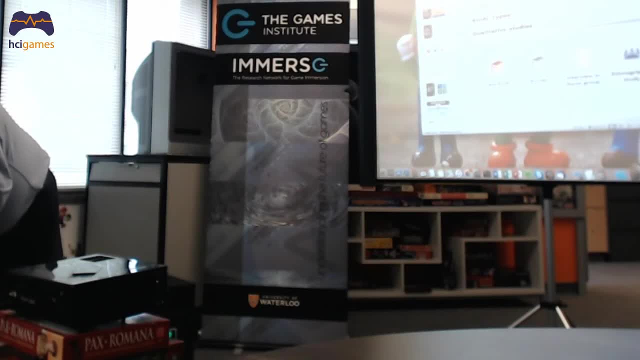 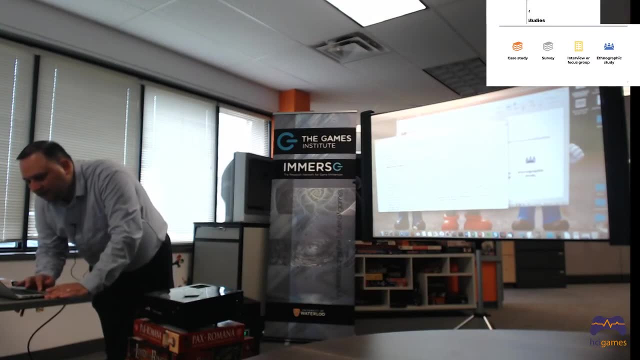 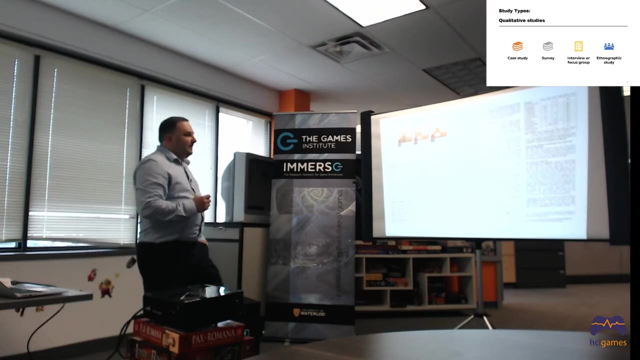 it's quite common to have some initial part of your study where you collect the measures there, So you test if something is true or not, and then you have later qualitative part where you ask people to explain. So this is an example of a study that I did. 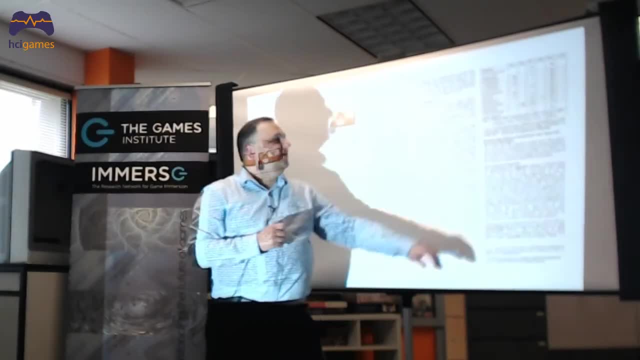 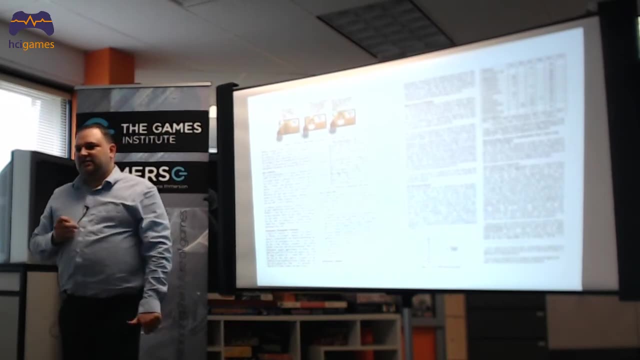 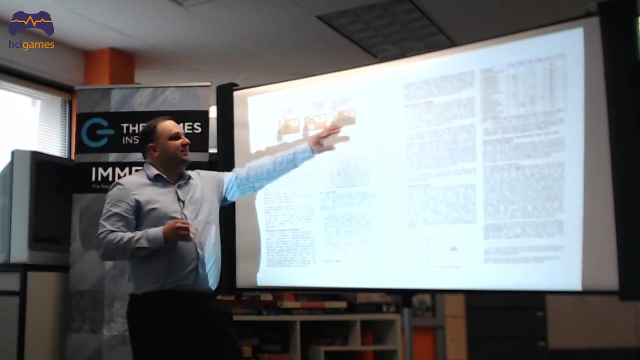 with Rita that was mixed like this. So we have a qualitative part here where we showed people these storyboards of some, I guess, persuasive strategies And then we asked people how much would they feel persuaded by something like this? So we analyzed here. 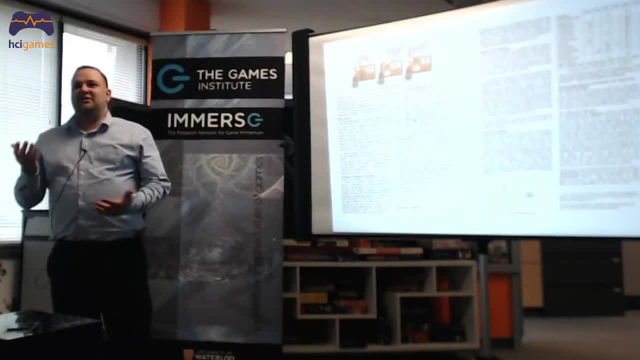 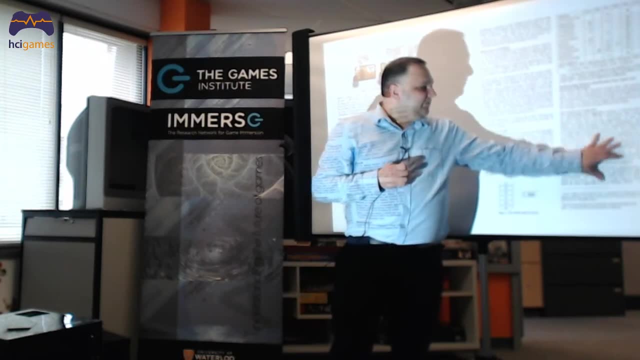 if how much they would feel persuaded was related to their gamification user types. And then we asked them to explain why. And then we have the qualitative part here. We'll go to the next page, But it's basically analyzing what people said, right? 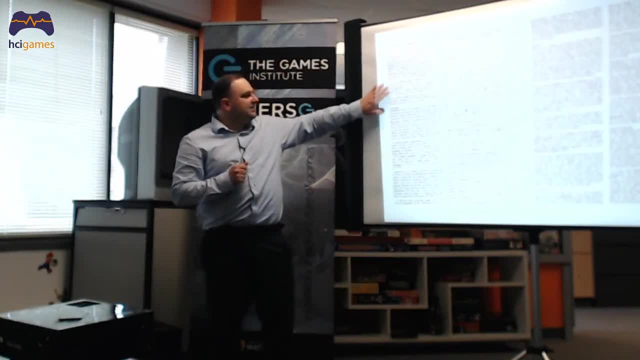 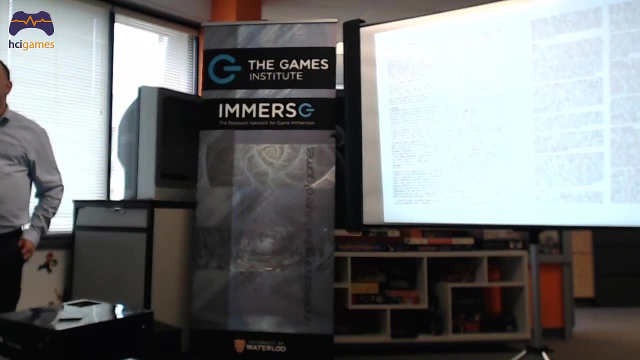 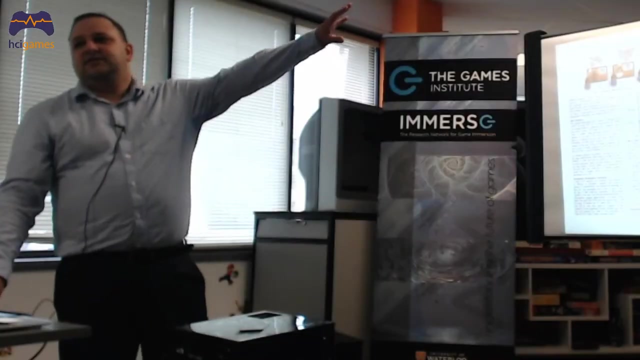 So if you look the parts that are in italics, here are quotes from what people said In regards to explain why, or why not, they would feel persuaded by that story. So we have both elements here. The qualitative part shows as if the storyboards work. 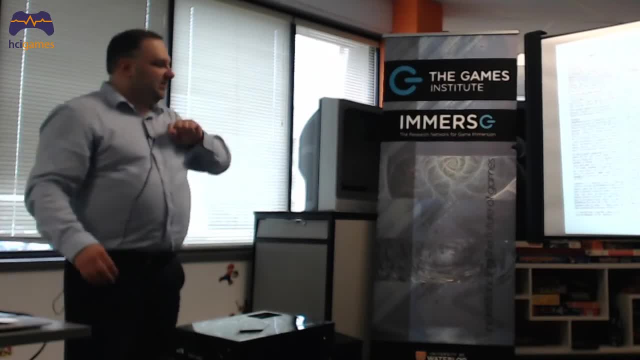 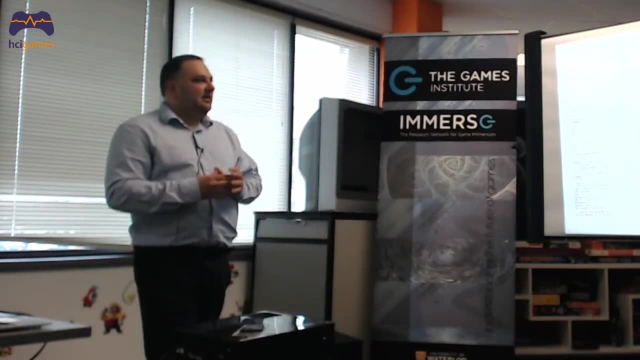 and if they are related to the user types or not, But they don't explain as why. And then the qualitative part: here right, actually read people's explanations and then we try to find commonalities between what different people said that we can do. 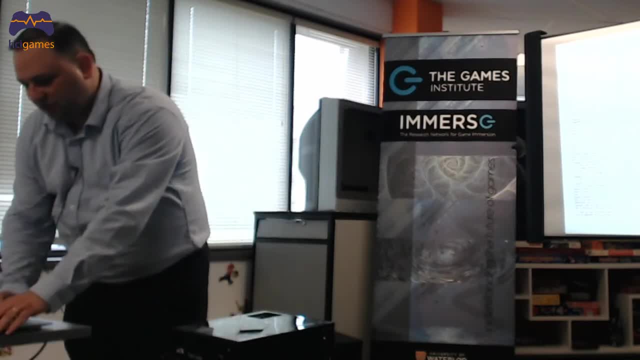 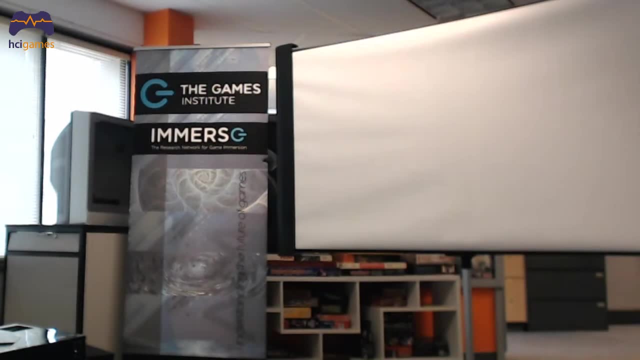 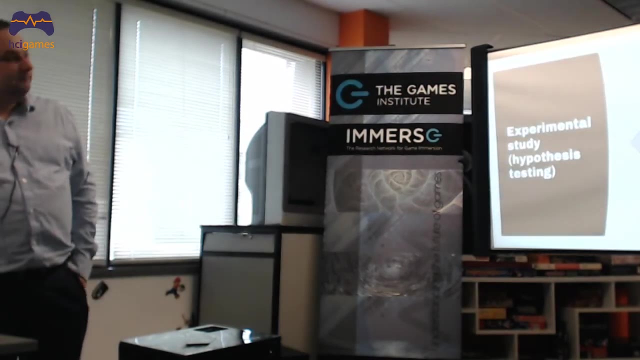 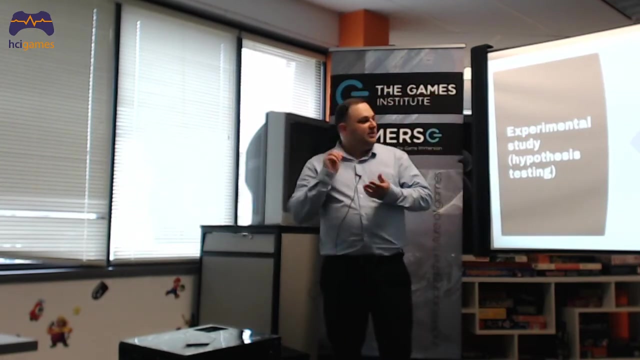 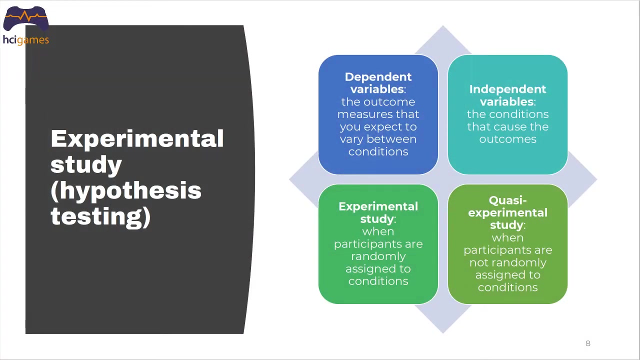 to begin to better understand why those storyboards really work or not. It's the qualitative parts there. So you have your goal, your research question. You decided what kind of study you want to do to answer that research question. If you're doing, 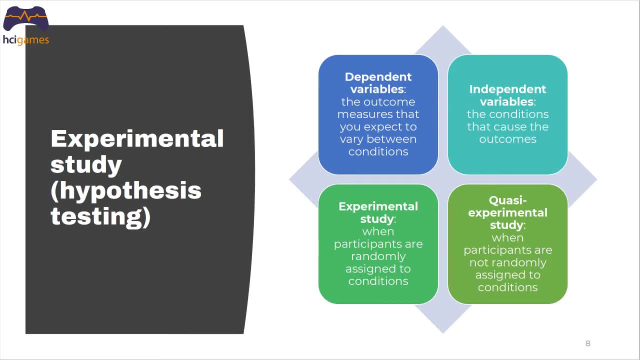 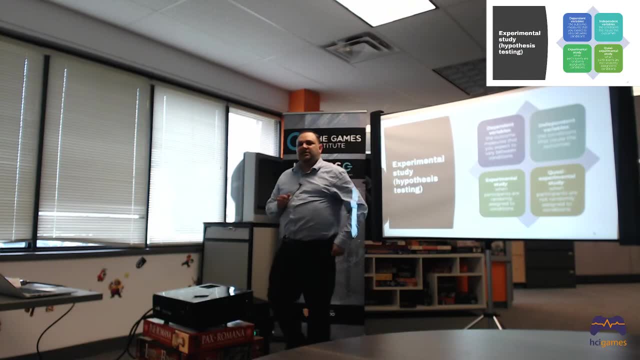 an experimental study, you also need to think about what variables you're going to measure. So usually you would have what we call the dependent variables. So these are kind of the outcomes of your measures and the independent variables would be kind of the cause of that outcome. 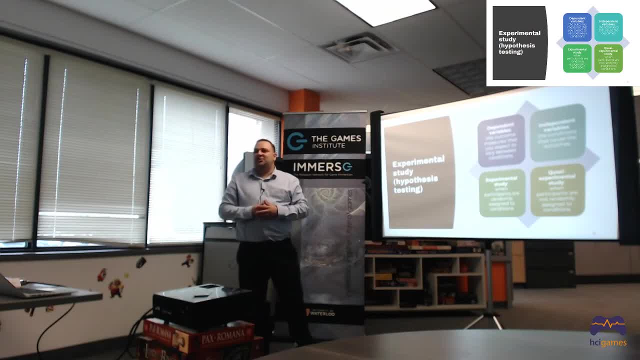 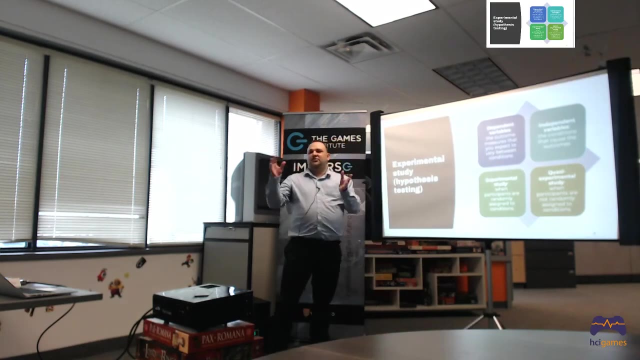 So if, just to give the same example, I'm testing different games- sorry, I'm testing if the same game played with or without sound, it's going to have different levels of immersion. So the independent variable is sound or no sound, right. 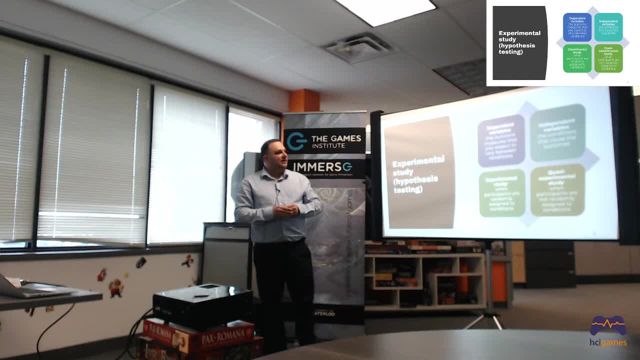 That is what would be causing the differences in the outcome, and my outcome would be the level of immersion that people have when playing that game. So if I'm doing an experimental analysis, I also have to list which are going to be my variables there. 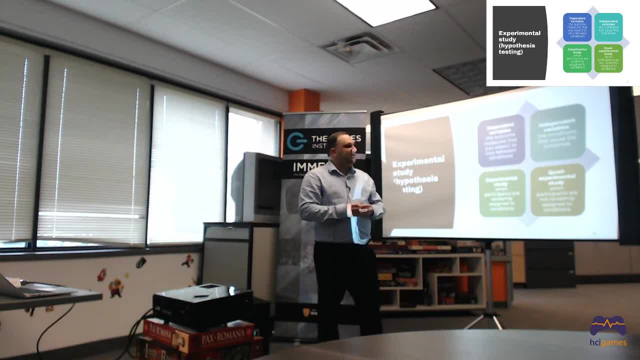 so basically, what are the things that I'm going to measure, what different conditions I'm going to have? just sound or no sound, or maybe sound could be also music or sound effects? So I can have two conditions or maybe different combinations of different sound effects. 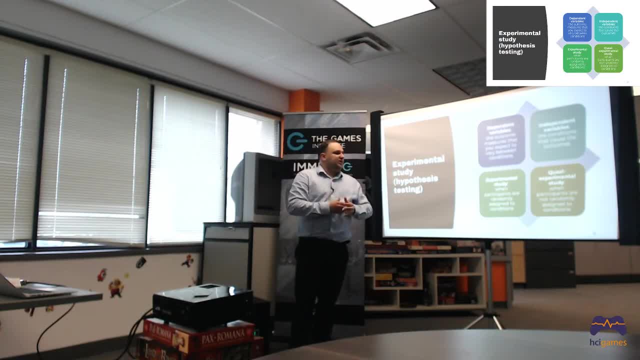 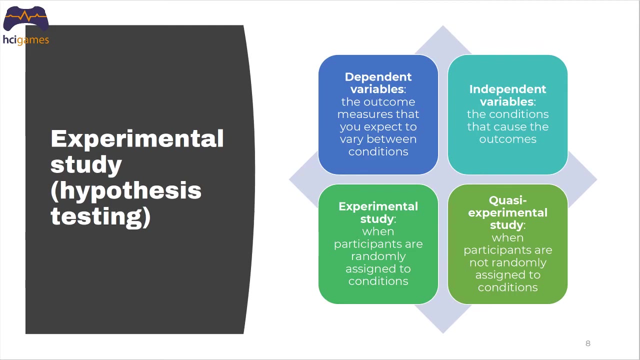 so I might have different conditions. So that's also part of planning what type of study I'm going to do. And for for real experimental study you have to take care that the only thing that you're varying between the different conditions is your condition. 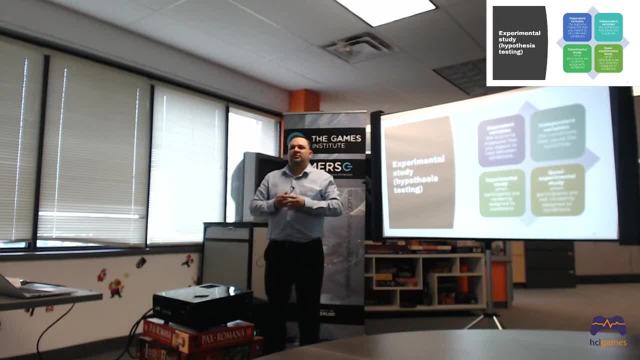 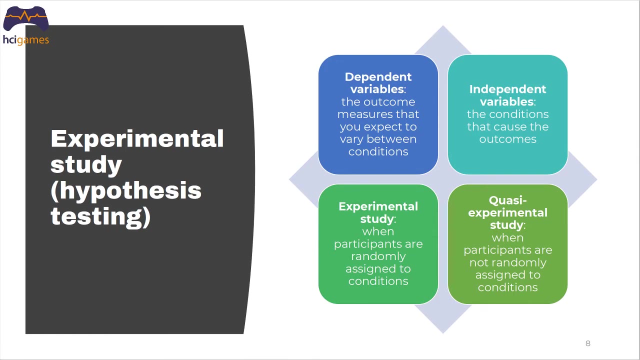 And that usually means that you have to assign points randomly to the conditions to ensure that there isn't anything else that might be affecting your condition there. If you did something like this, for example, everybody from University of Waterloo is going to play the game. 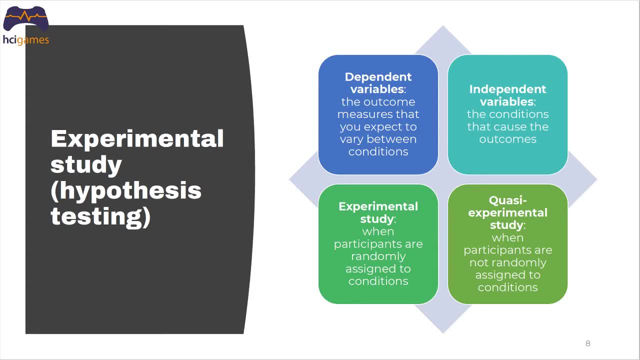 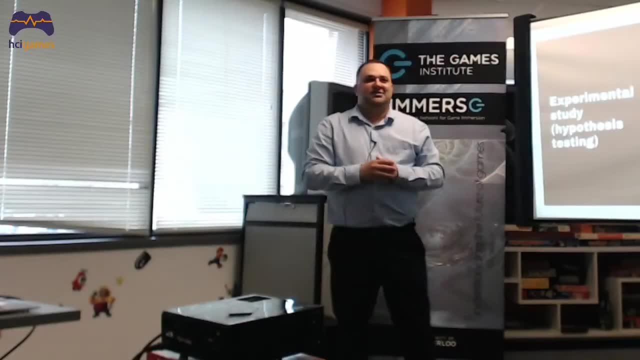 with sound, Then I'm also going to go and recruit people from University and they're all going to play the other condition right. So that's not a good design, because if I see differences on immersion, was it because of sound or no sound? 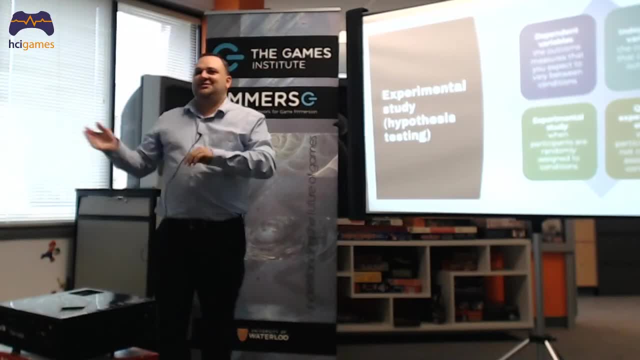 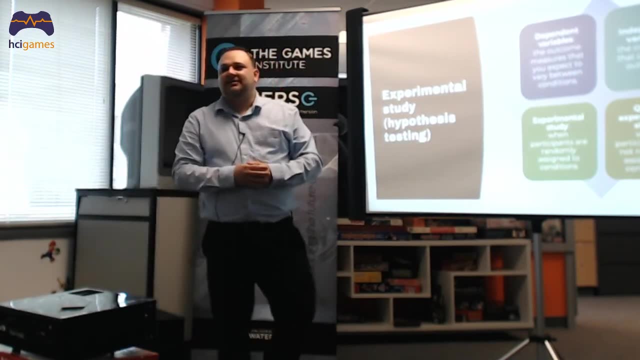 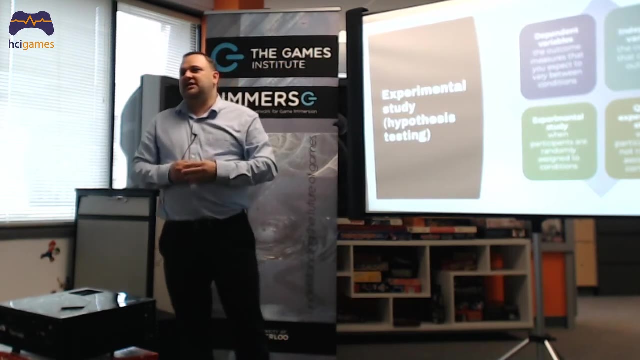 or was it because people are from different universities and then being from different universities for some reason causes people to feel differently immersed on the game, right? So if something like that happens, we have some sort of confounding variable there In this case. 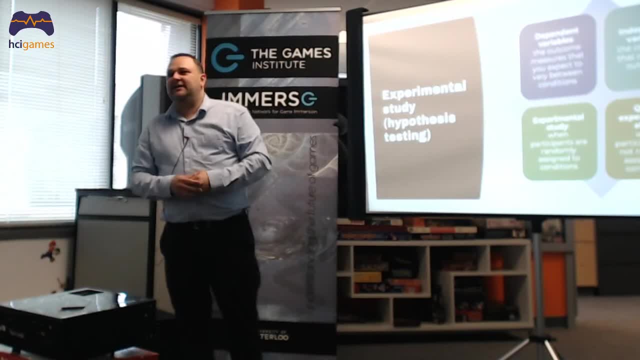 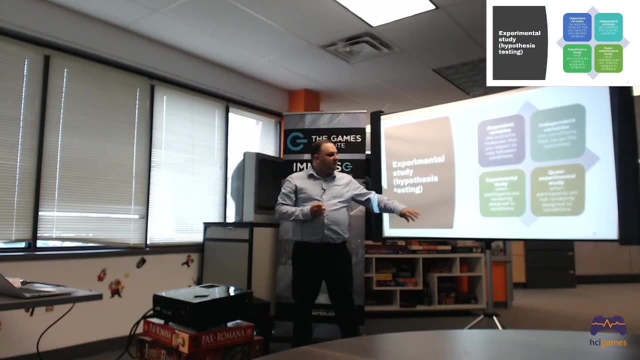 the university where people come from would be the confounding variable, something that might be causing their difference in outcome here. that's not what I want to test. So to have really good experimental study, you have to avoid these kind of things, and that usually involves. 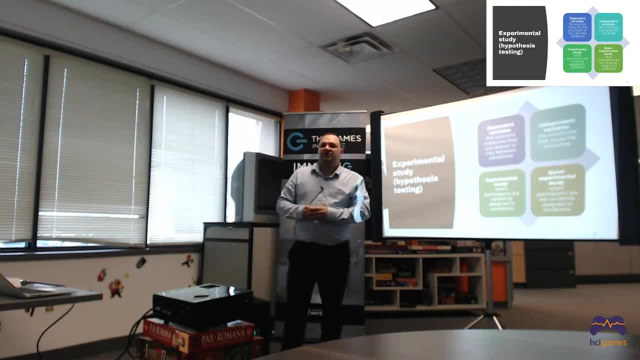 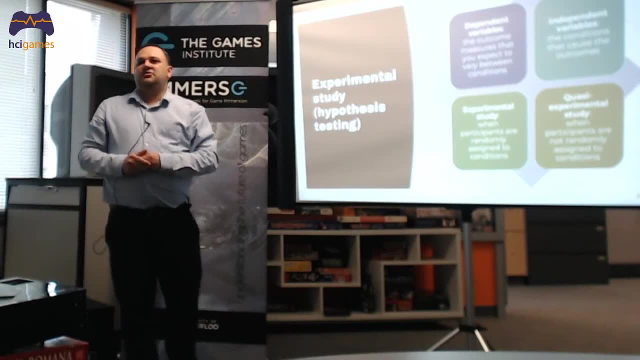 as I said, randomly assigned people right. So you can have people from two different universities coming to Poland, as long as you randomly assign them to the conditions. So in the end you'll have kind of a similar number of people from both universities. 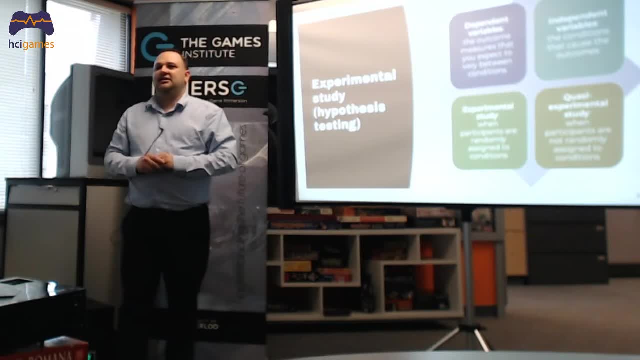 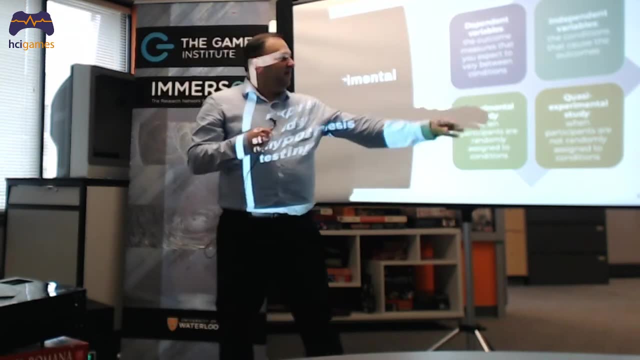 in both conditions and that's okay And the university where people come from will probably not going to be affecting your results. But sometimes you cannot really do random assignment of people to conditions, So when you cannot do that, you cannot say that it's a really. 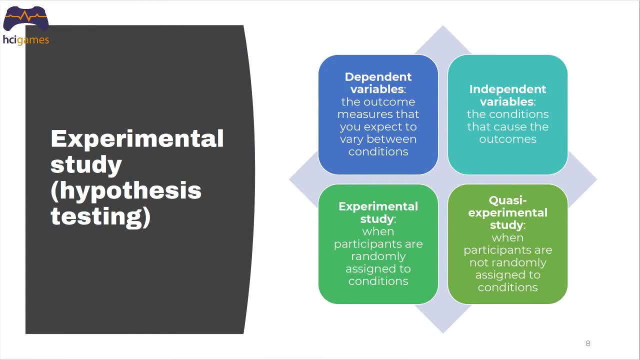 an experimental study, But sometimes you do random assignment of people to conditions, So you have to do what people call quasi-experimental studies. It's almost an experimental study, It resembles one, but if you are not able to assign concerningly, 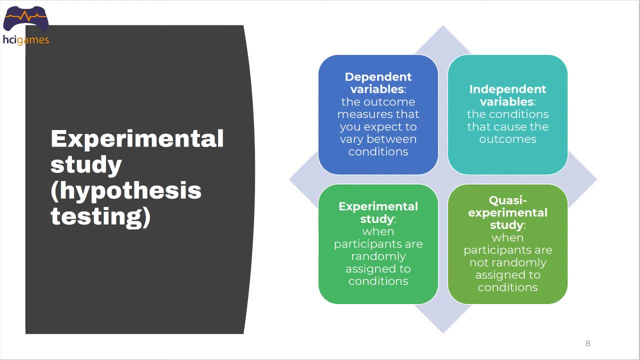 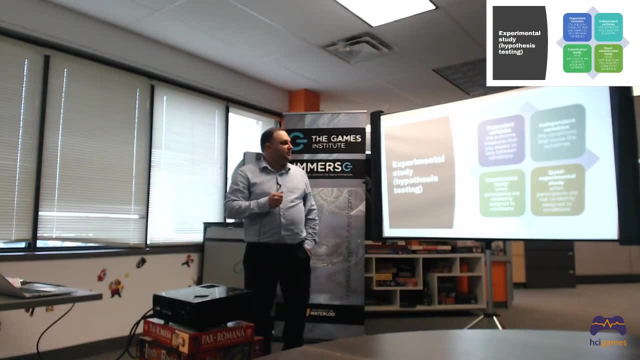 then you lose at least that part there. You might have some confounding variable then that you need to take care of, So you also need to think about that. If you can assign people randomly into an experimental study, then it's usually better. 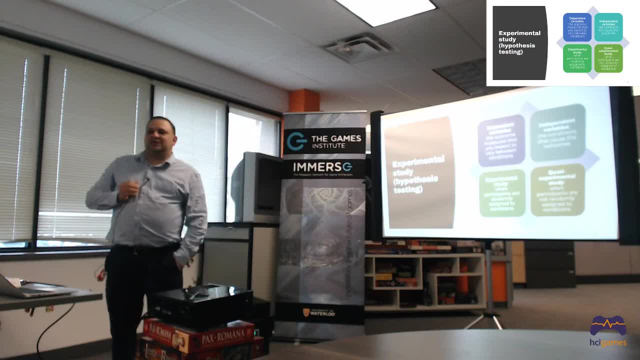 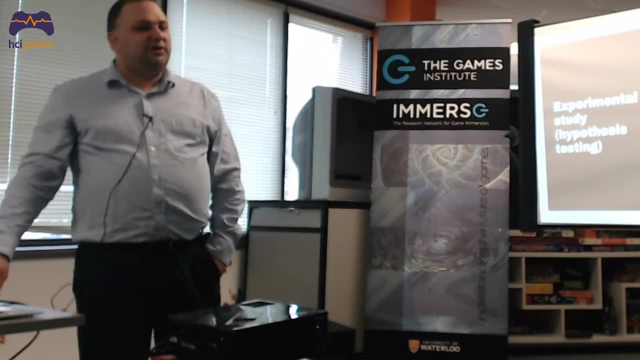 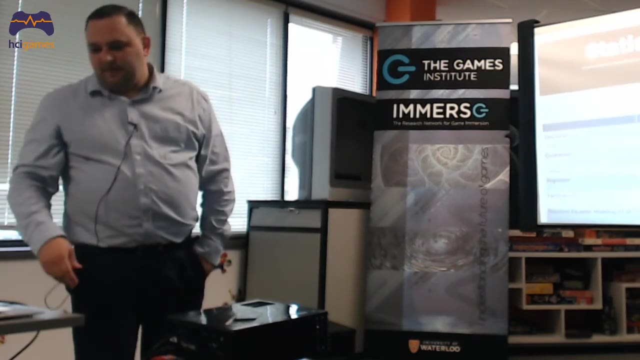 I mean, this is just a very short comment about things that you should think about through, just upon things that you should really study and learn more about them, If you don't how much yet when you are planning your studies, but these are important things. 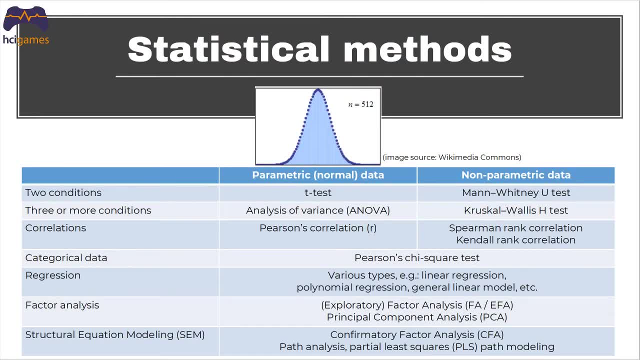 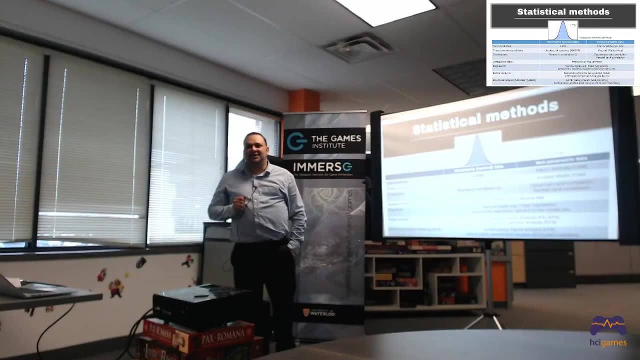 And finally, you have to decide what statistical methods you're going to use. I'm actually going to read off them here and put them just more as a reference, because in fact you want to have these slides and look here and look as a reference. 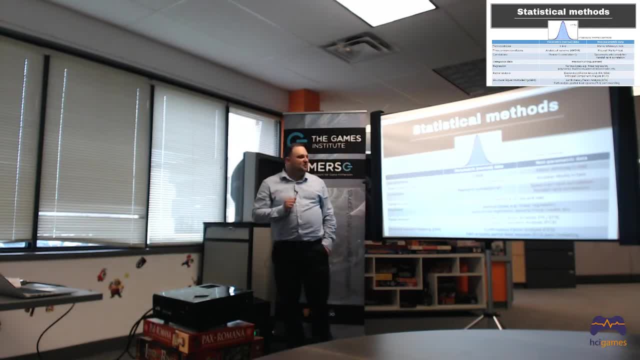 of just the most common methods that I've seen, at least in the papers that I've been reading. There are many, many statistical methods for lots of different applications, So you could probably be doing something like this. You need to know if your 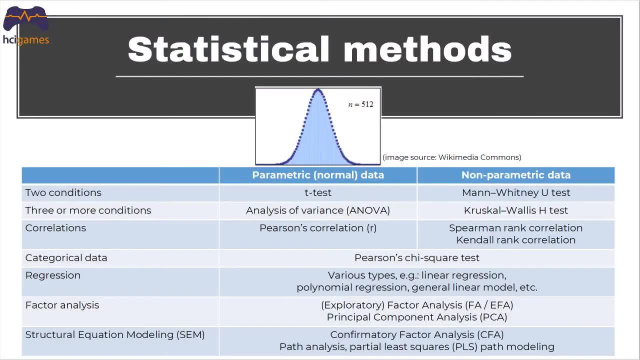 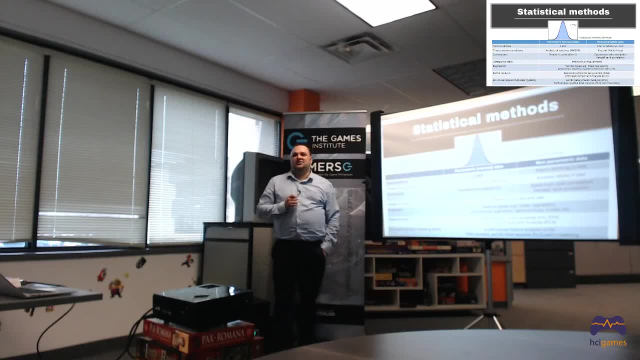 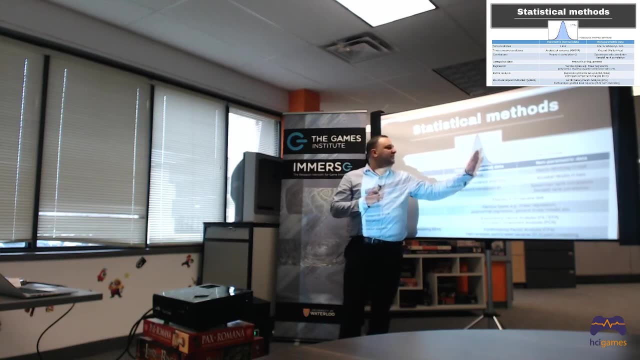 data is normally distributed, or is parameter data, which, if it is, it basically means that when you put a chart of your data, you'll see something like this: like around the average, the sort of people that have that score, And then, as you move, 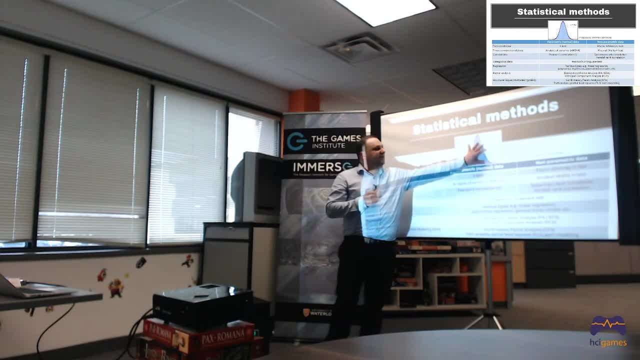 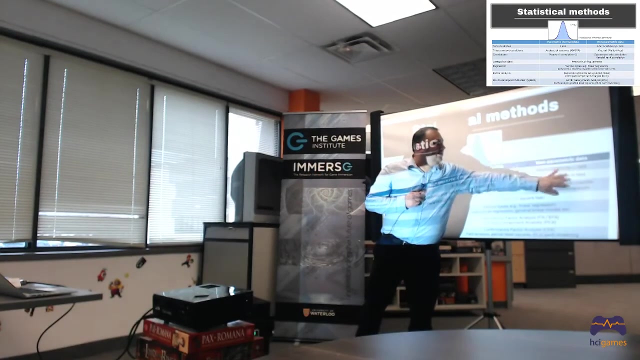 farther from your average data, you'll see something that's very different from this. So if you have people with different scores here, then this would be a score and the number of people that have that score. So if you don't have something, 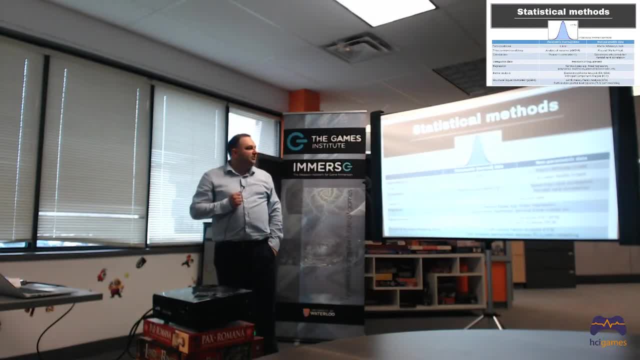 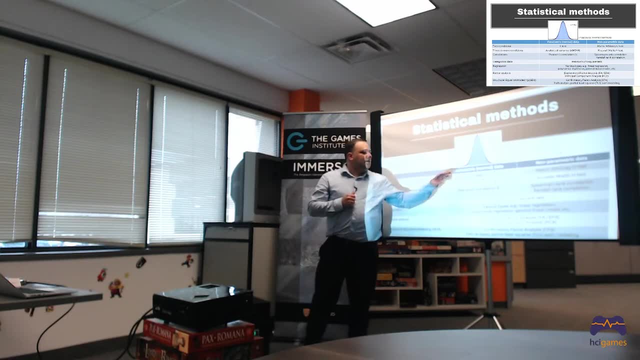 like this, then the kind of statistical paths that you're going to use for some of these results are going to be very different from what you usually think about. So most of the time you cannot do this decision when you're planning your study. 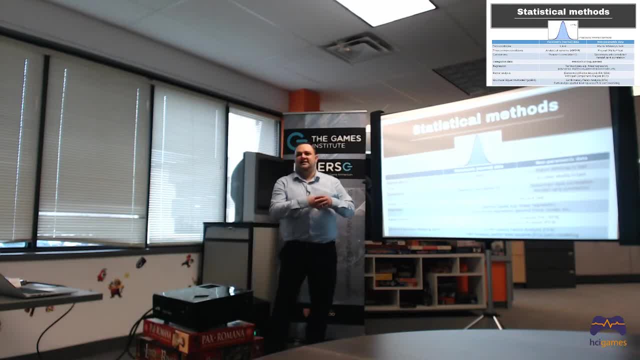 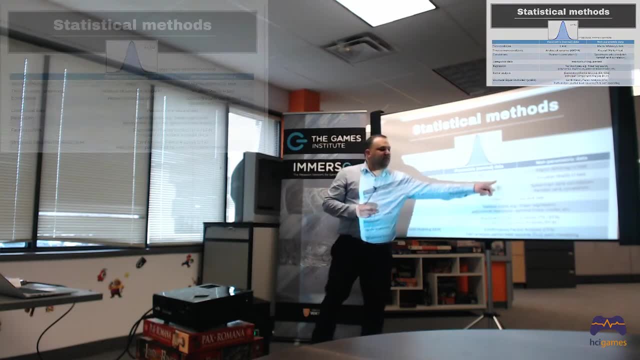 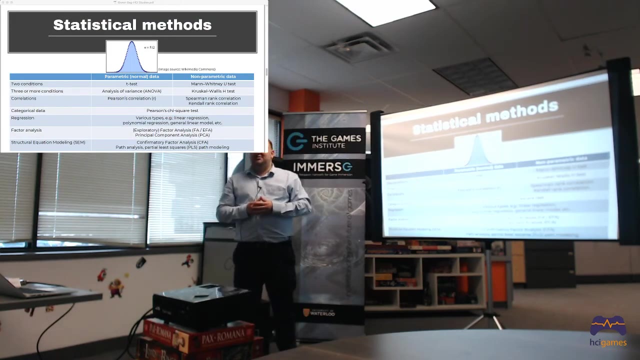 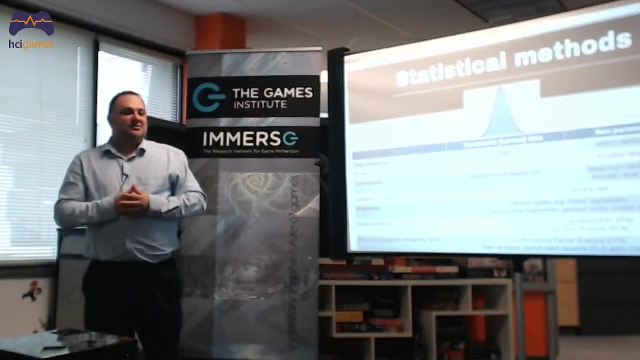 because you need to actually collect data and then test if it follows a normal distribution or not. So if you do the analysis of variance and the results of that, probably at least one of the reviewers is going to tell you: did you check if the 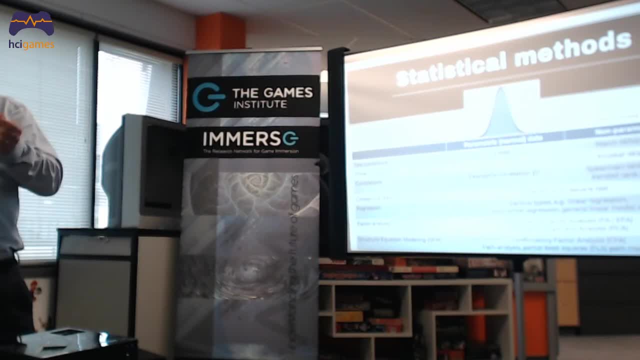 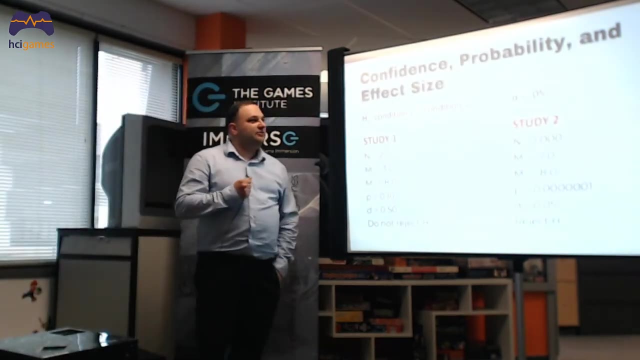 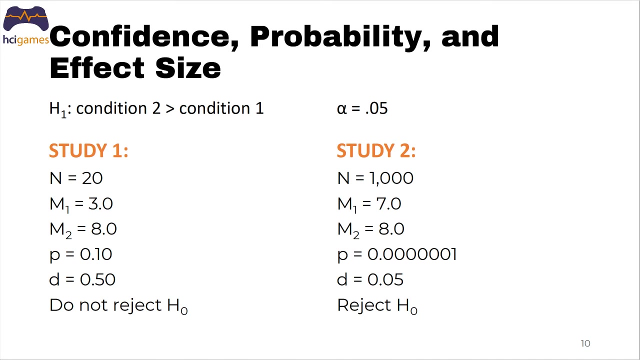 data was normal before doing the analysis of variance, because if you did not at least show some confidence that your results are right, Okay. another thing that you also need to worry about now is not in planning, but when reporting your results after you've done the 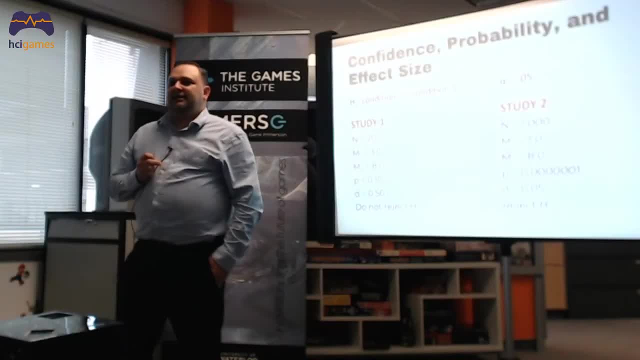 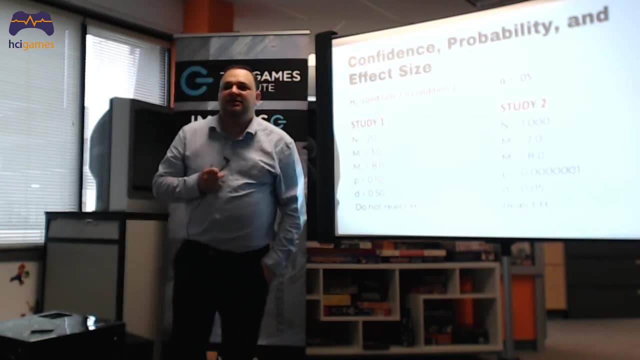 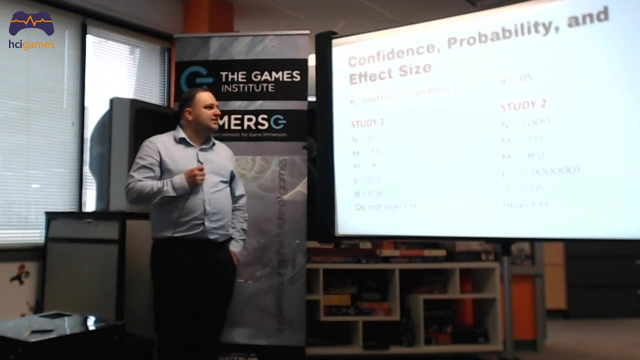 analysis is that the probability of your hypothesis being true or not and the effect size of something are not only in HSI studies but also in HSI studies, so you need to be careful about that when reporting your results. For example, let's say I did. 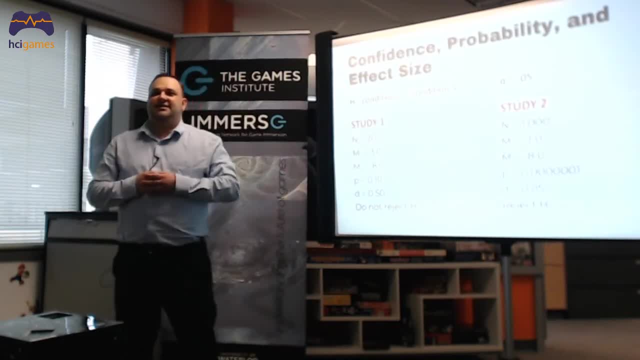 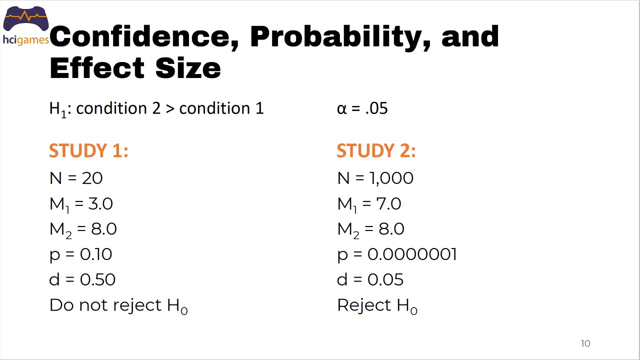 my study there. let's say, I created a new, improved controller for virtual reality and I want to test them. so my hypothesis is that condition is going to be much worse than what it was before. So you might get something like this. let's say: 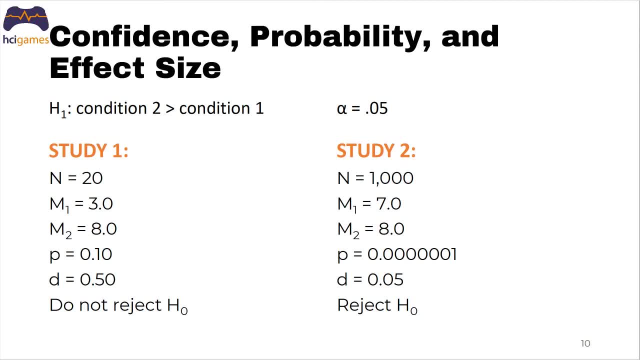 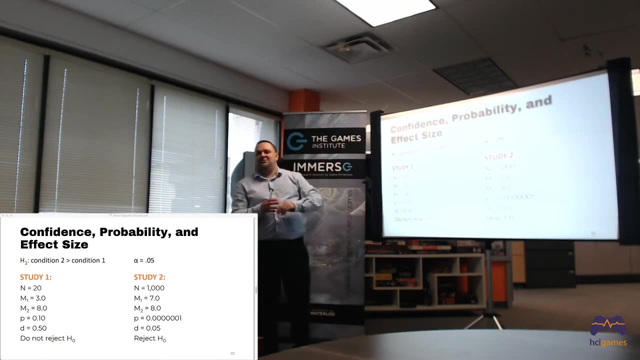 you measure something on a scale of 0 to 10, how well did people perform with that controller? and, on average, people that use the original controller scored 3 and 0,, for example, But something that might happen since you only have a few. 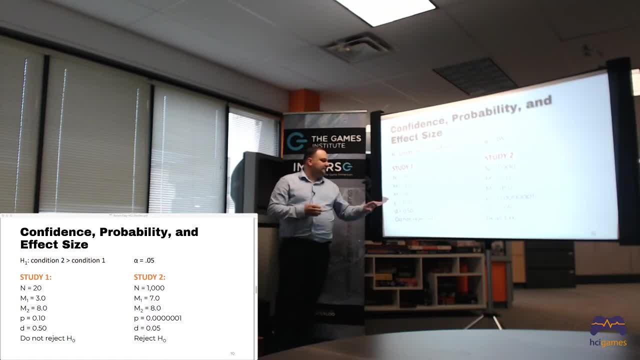 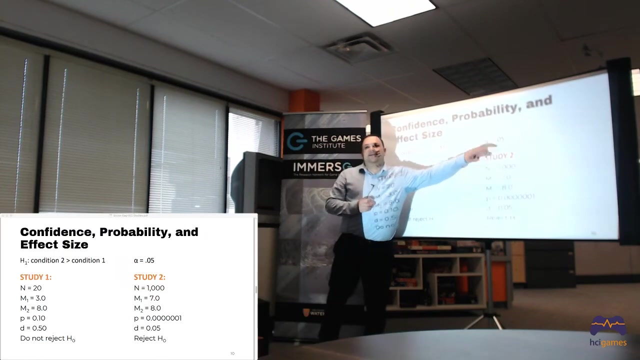 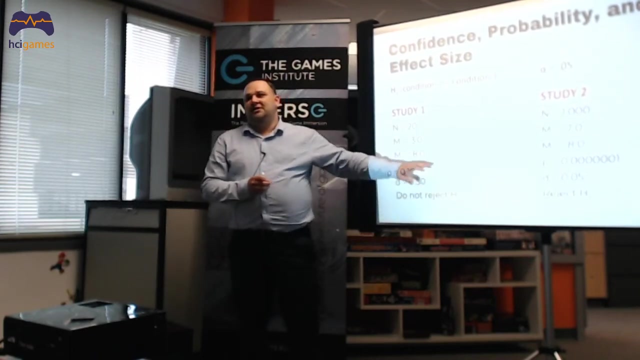 people is that you might have a probability that's not very good. so usually when you're doing testing processes like this, you'll define, before calculating your statistics, what confidence you want to have and what you want to do in the process. So what I'm going to 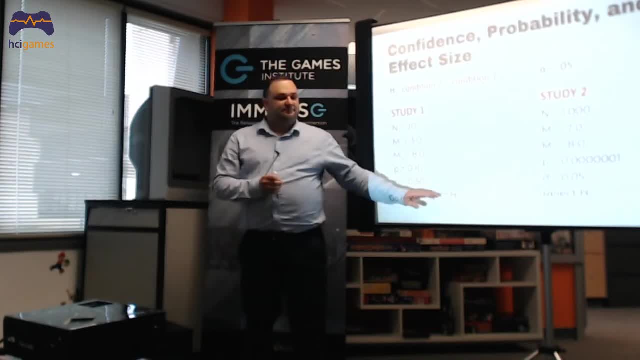 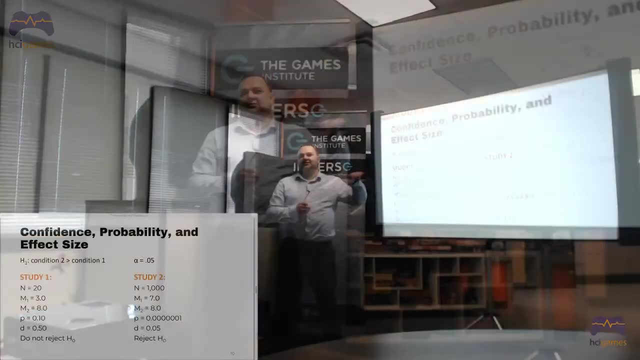 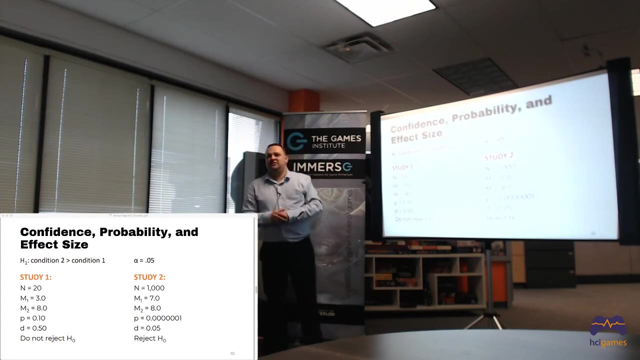 do is. I'm going to do the same thing that I did with the old controller and the new controller, and then the whole year I recruit a thousand participants and make 500 use one controller, 500 use the other controller, and now let's say a lot of. 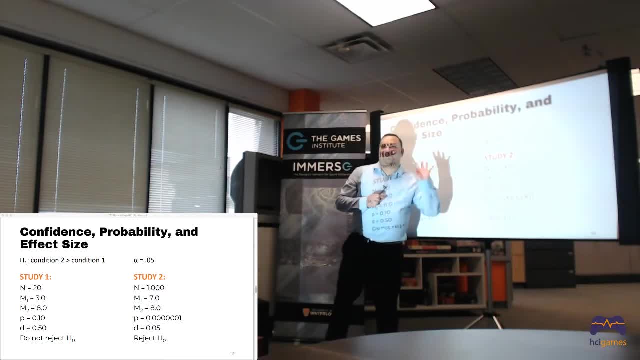 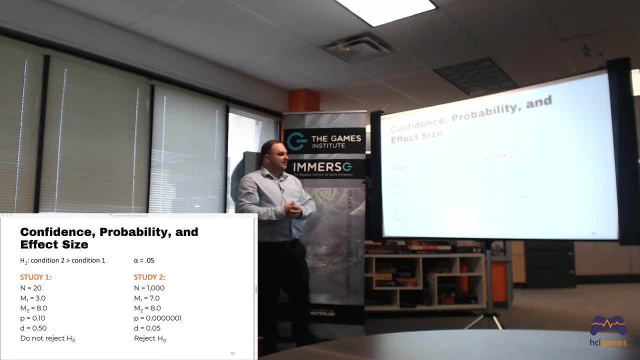 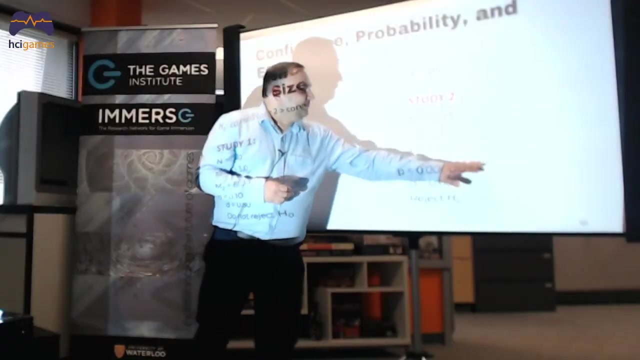 people that used the original controller scored an average 7 on my performance test and a lot of people that scored that used my new control test. usually the software only shows zero, but I put like a bunch of zeros in a one to make it look nice. 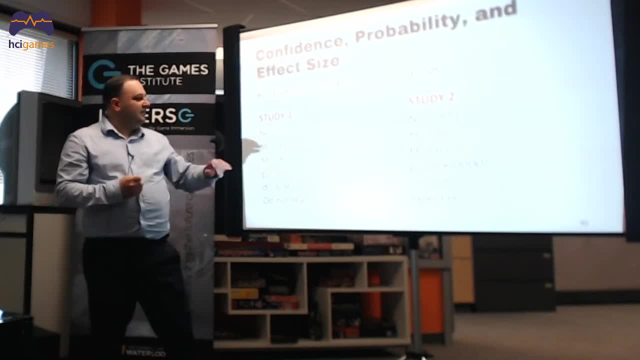 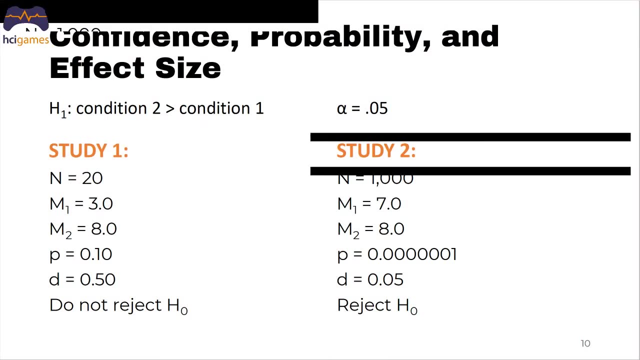 But anyway, what matters is the probability is much lower than my confidence there, Then I can safely reject the new hypothesis and I can assume that if better means going from 7 to 8. maybe yes, maybe not. it's not much difference, right? So that's. 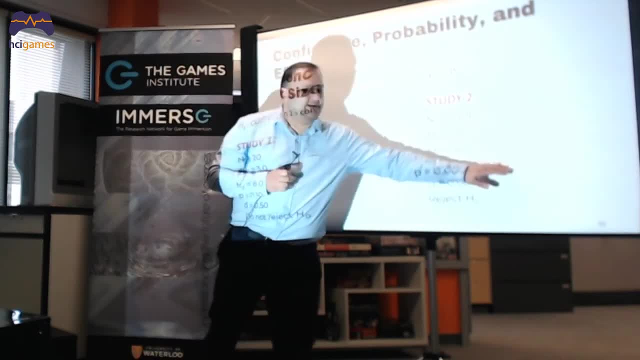 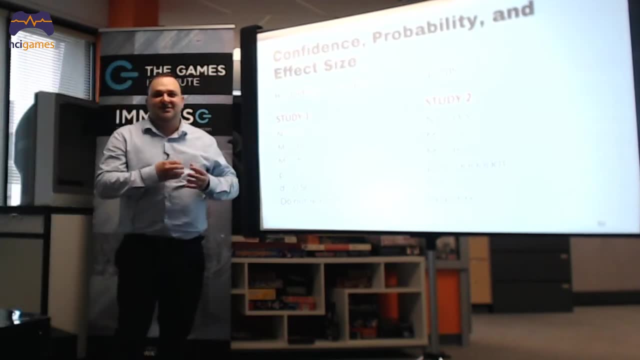 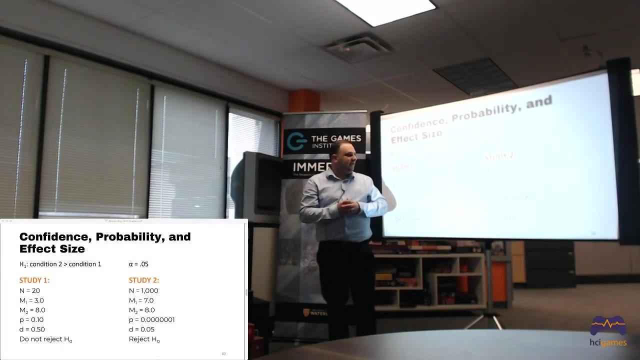 what I want to highlight, because sometimes people just look at this number here and, yes, I'm very sure that my controller is much better. but my controller is better, yes, because I have a lot of participants. that's why you can be really sure. but the difference between them 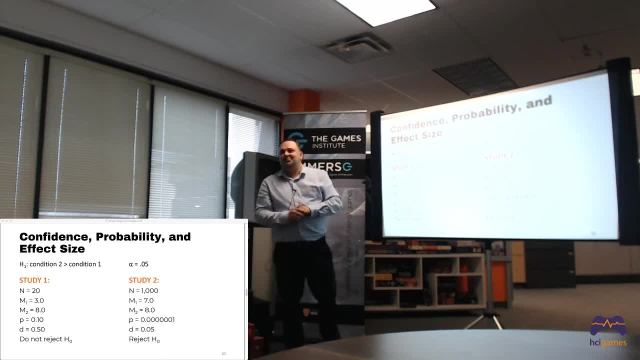 was actually not that large, right? So it's better, but it's just a little bit better. and then you would have to calculate another number, which is effect size. So you had five points of difference here, right? So here you saw a large effect size, but 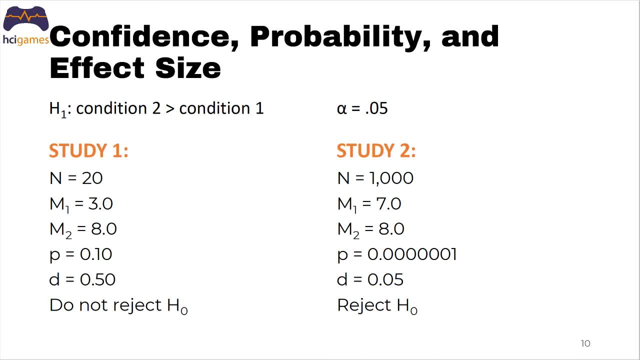 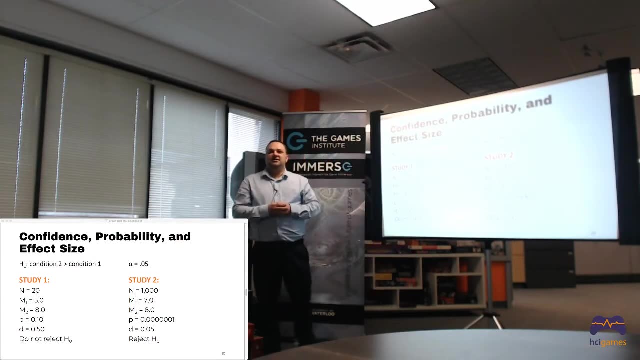 since you had just a few participants, you were not very sure if this difference was because your controller was really better or just because randomness, just coincidence, because of the people that you invited, etc. If you have a lot of participants, you can be sure that you have. 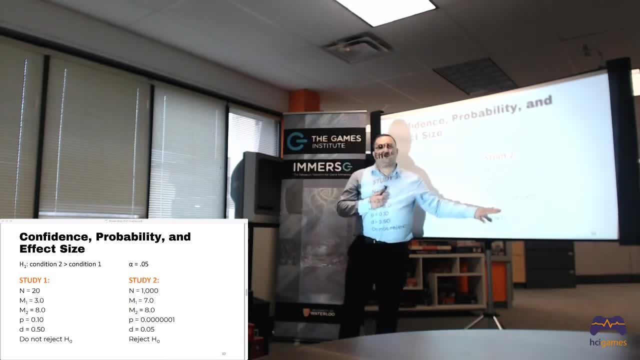 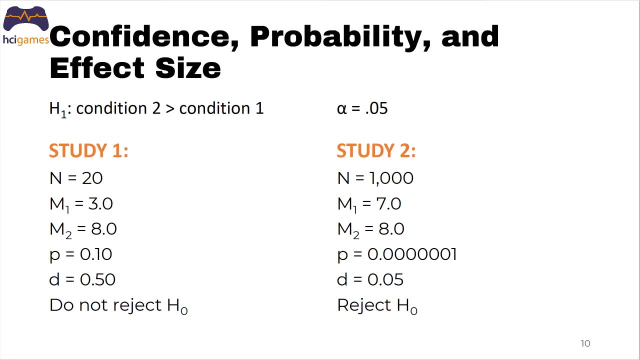 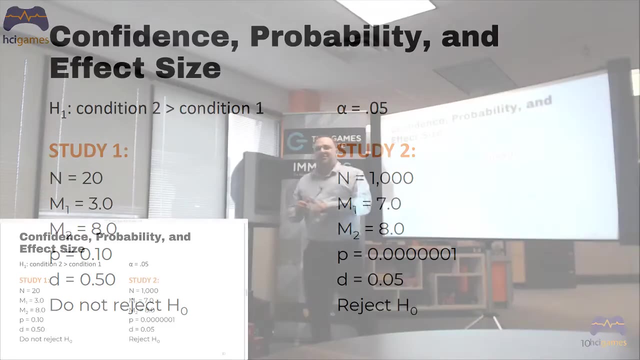 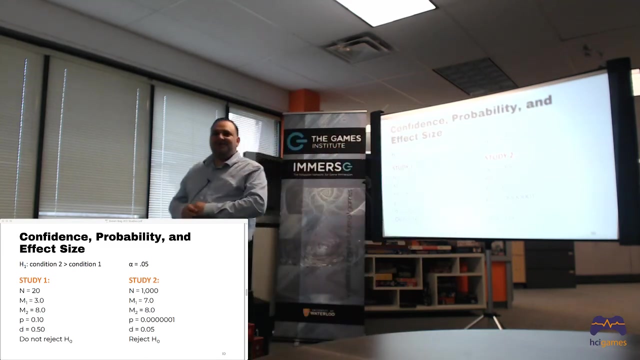 significant results, but you have to check what's the effect size as well, and it can be something small, So you could still publish all these in your paper. you made a test. you're very sure that your controller is better, but you have two controllers and yours. 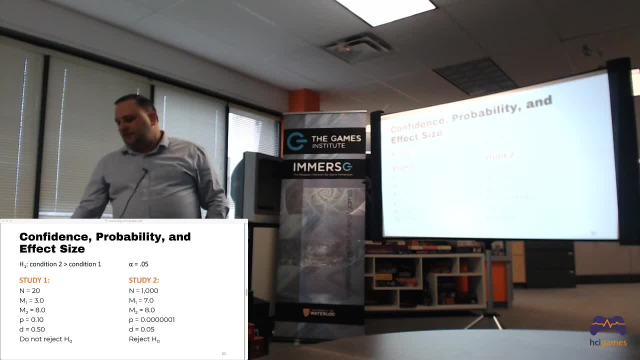 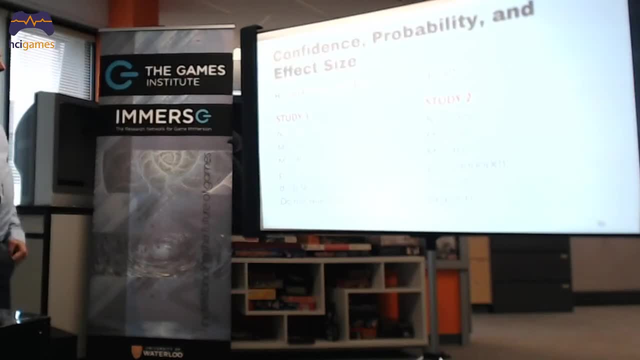 just a bit more than the other one. So things to worry about when you are reporting the results of your study. People are really really asking for effect size and for you to be clear about how better the things are on your testing. because at this point, 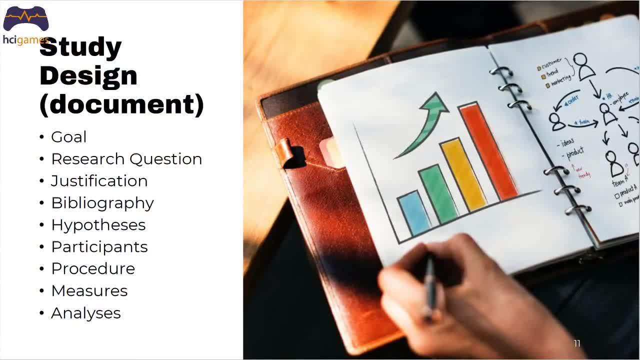 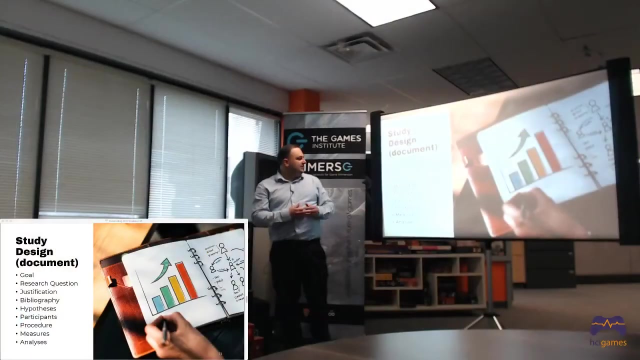 everybody realized that just being careful about what you're doing is going to affect the results of your study, So you have to be very careful about what you're going to do. I suggest writing a document with the goals, the research questions that you have. 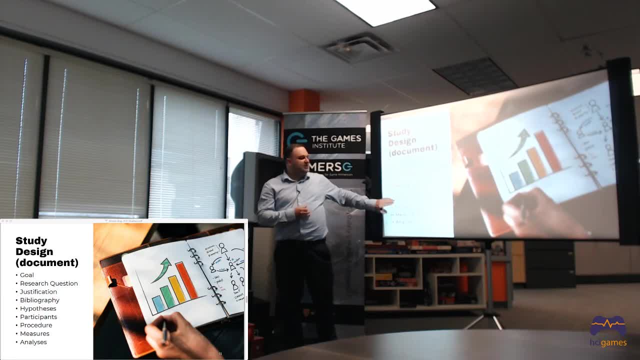 that justification why you're doing this study, the geography that you use, what are your hypotheses, who are the participants that you're going to recruit and what's the procedures or what participants are going to do, what they're going to measure and how. 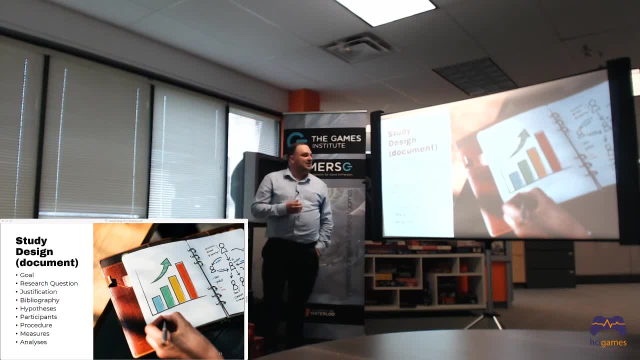 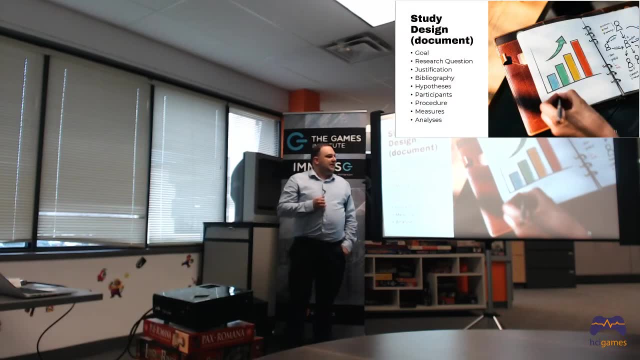 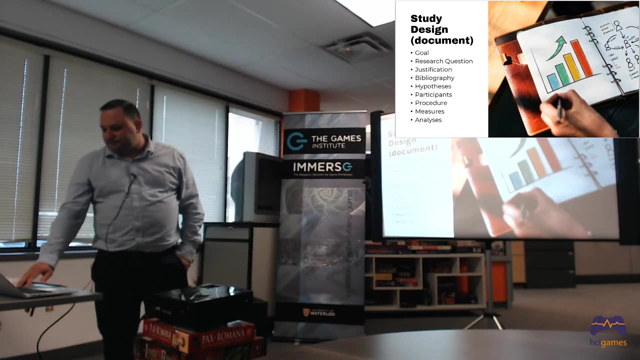 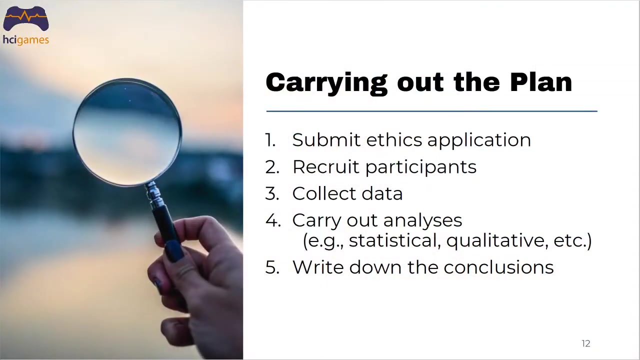 you're doing so. you can give suggestions, you can improve your study, you can communicate with people that might be helping you run the study, so everybody knows exactly what to do. You also have to submit applications to the ethics office and approve your study. 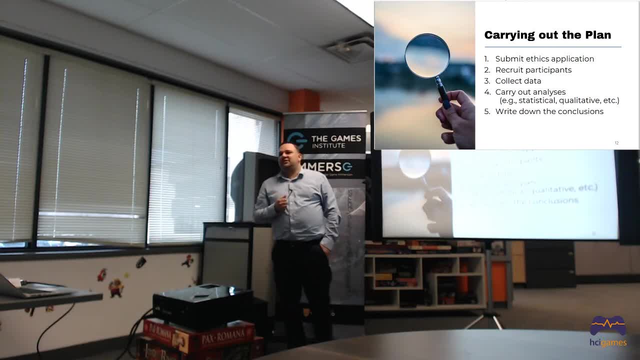 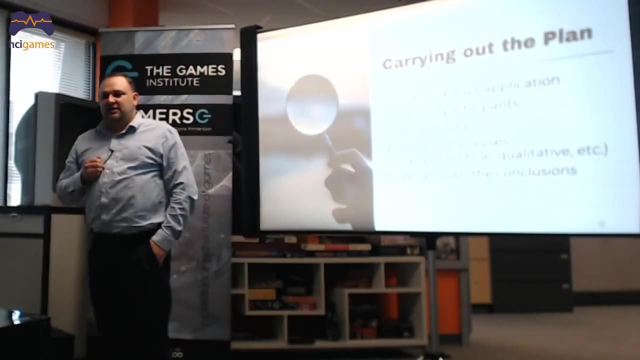 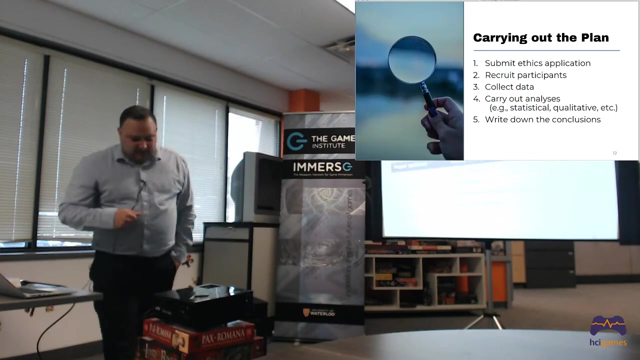 and then you already have all the information that you need on your design document. so you just have to pop your information into the ethics application form. Then, after you've approved, then you can recruit participants, collect all the information that you need And, hopefully, 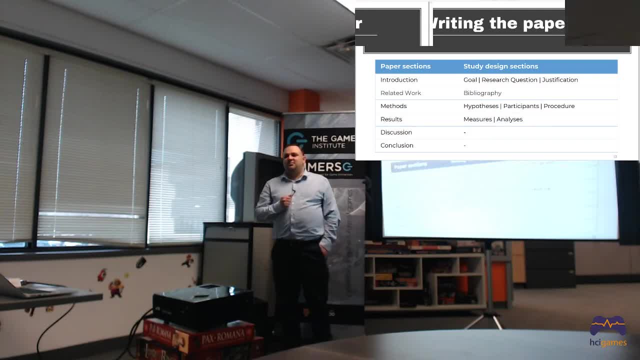 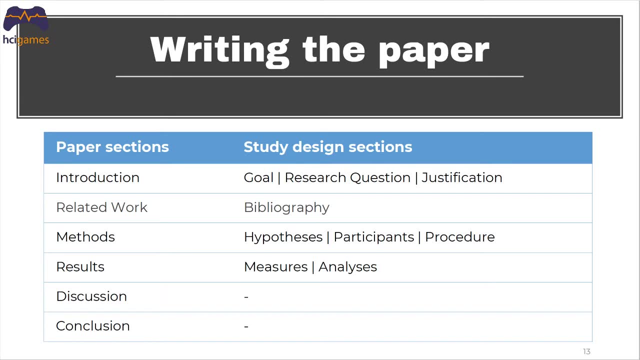 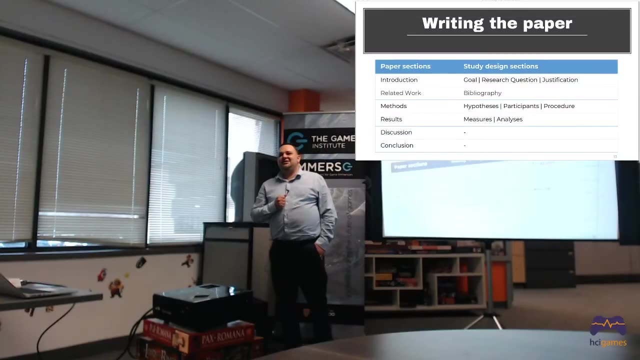 you have favorable conclusions and you're going to want to publish a paper about that. Now, if you did write the study design document, then you already have your first paper draft. It's nice, right? So that's the thing that I have, this. 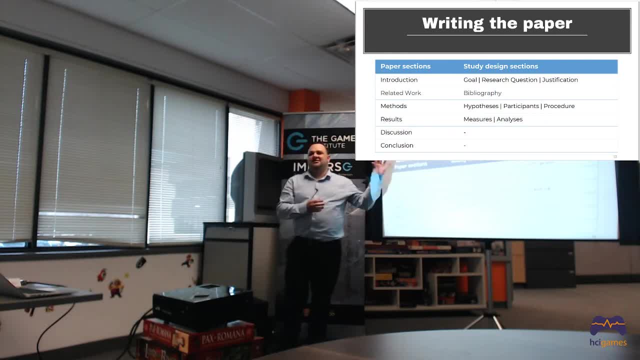 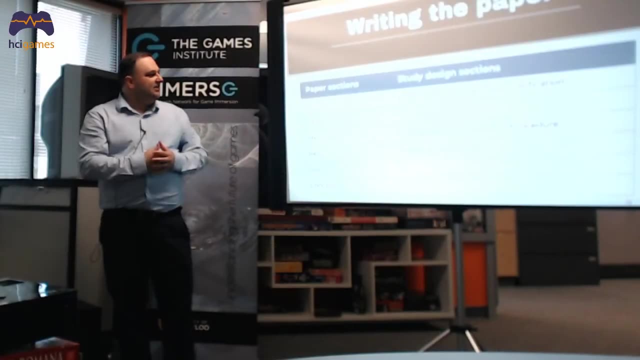 clear story about exactly why I did this, why this analysis and how this analysis helped me solve the research question. because if you want to do that in the end, then it's confusing, right? If you have done everything in the beginning, it's. 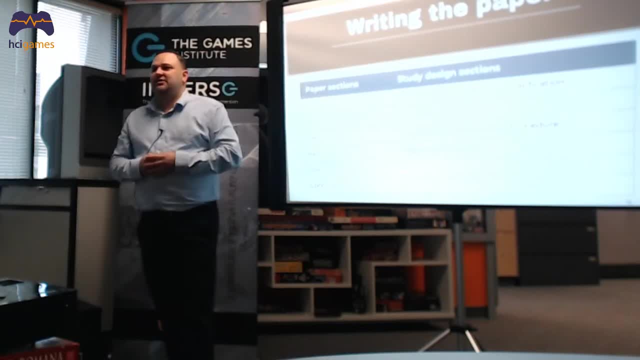 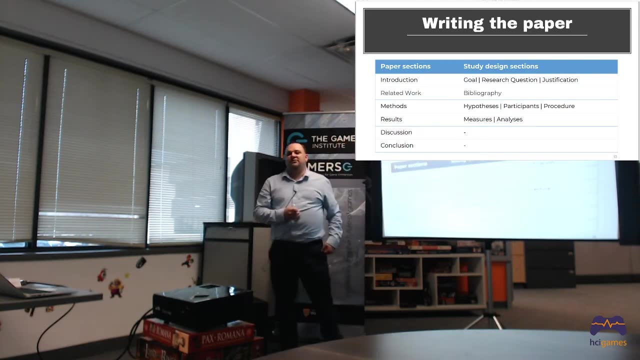 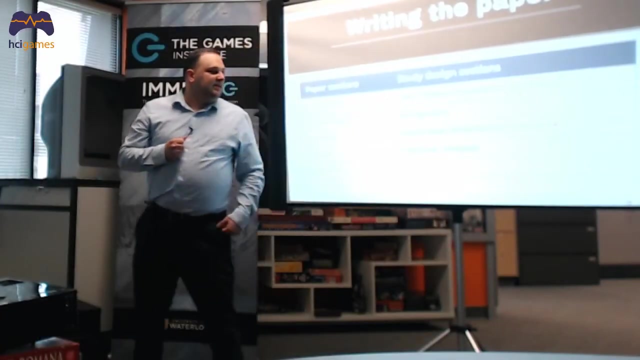 much easier. The first thing you have to do is to look at the data that you have in your paper. The second thing is to look at the data that you have in your paper, So you should have everything already in your design document: The results. 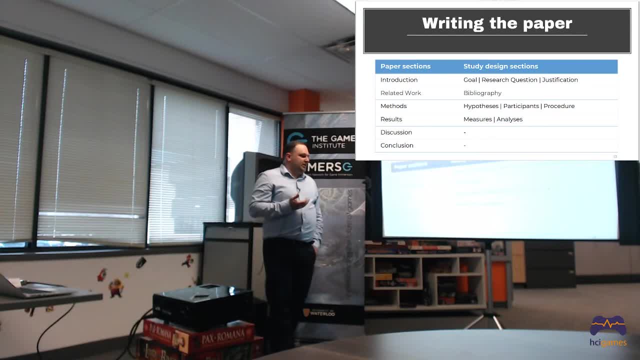 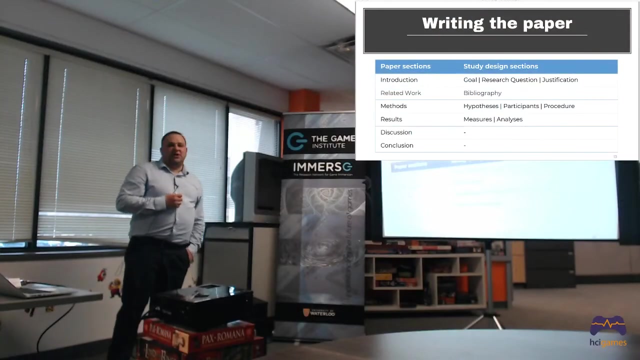 are going to be the measures and the analysis that you did. So your design document already had information about what you're going to do Now, here and then, of course, just the discussion and the conclusion of your paper, the reports that you're. 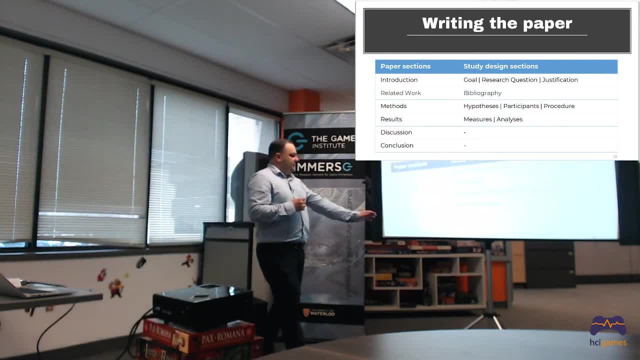 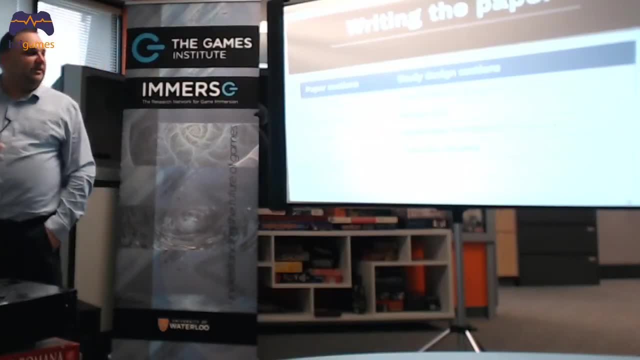 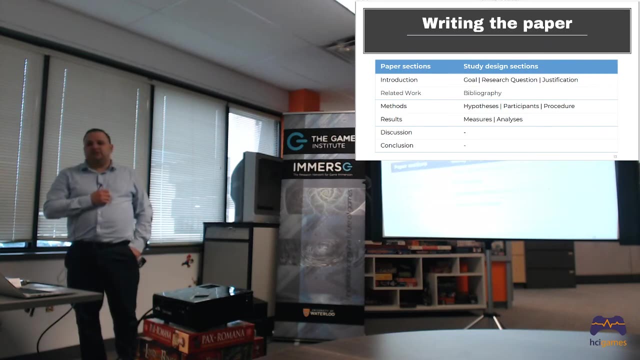 going to write up after you've done your study, and that didn't come directly from the study design, Although even in the conclusion you're going to go back to what you had in your design document. So, yeah, I've been doing. 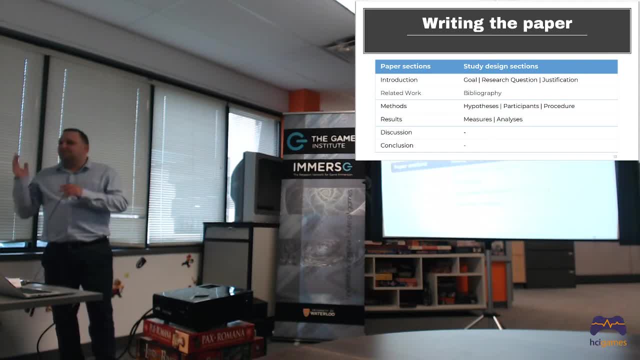 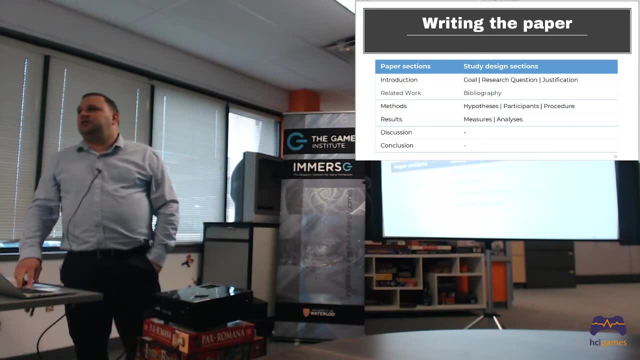 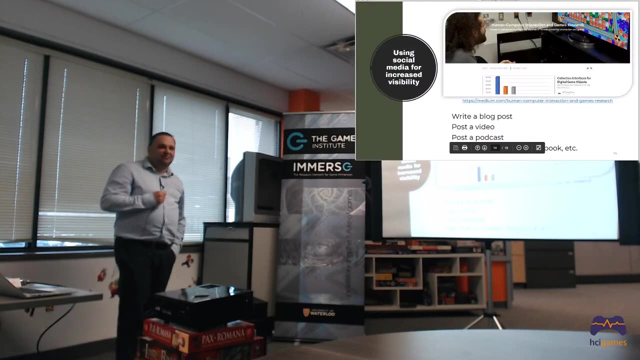 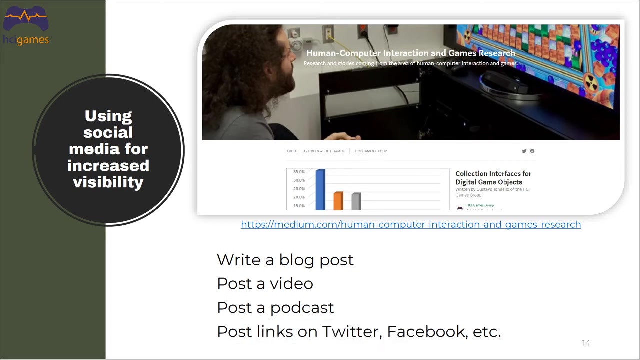 that now and I feel it's much easier to get to the moment of writing paper and I have everything clean in my mind today, Justifying why the paper is the way it is. So, of course, writing the paper and publishing it is. 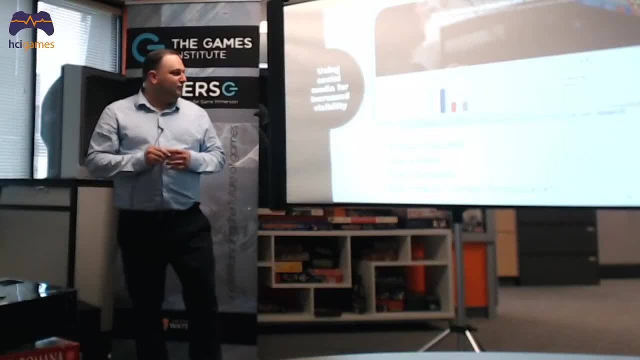 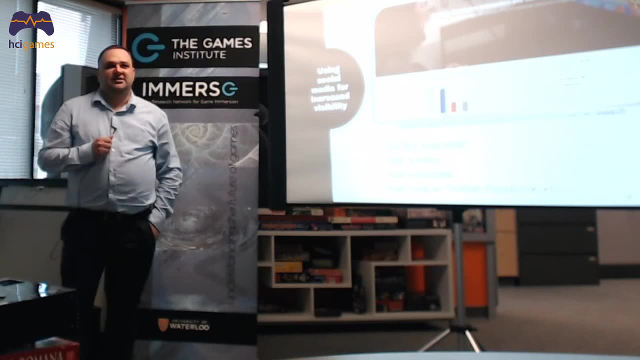 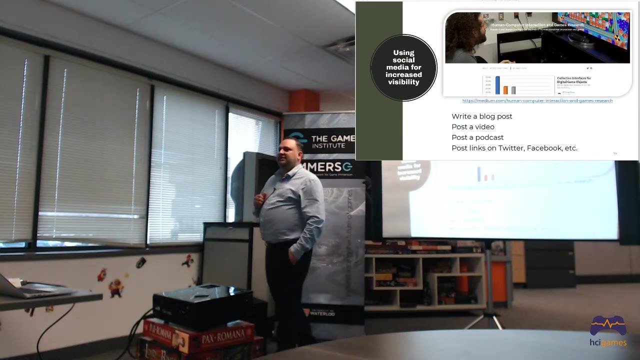 an essential part of research, but in our group we've been doing some other things as well to bring more visibility to our papers. It's been very interesting to see the papers that we've published. This is an example of a screenshot of our 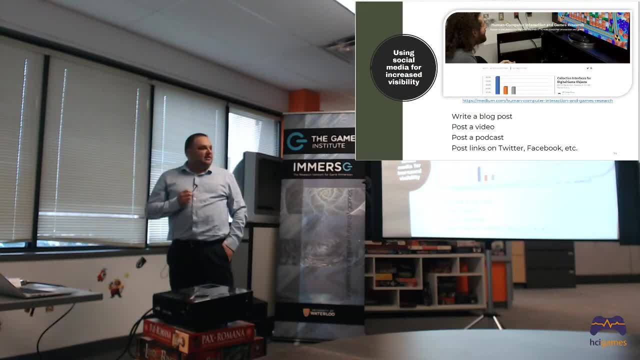 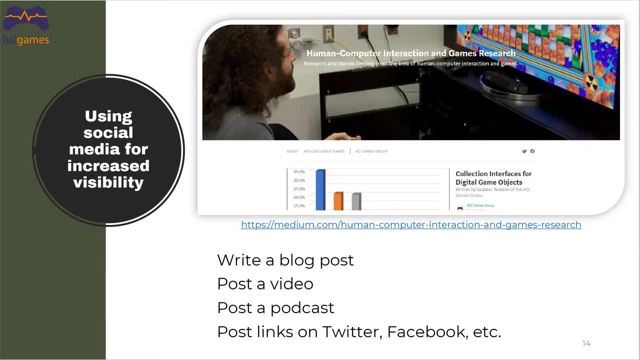 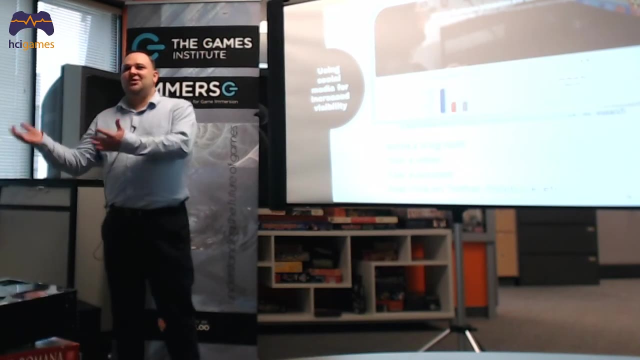 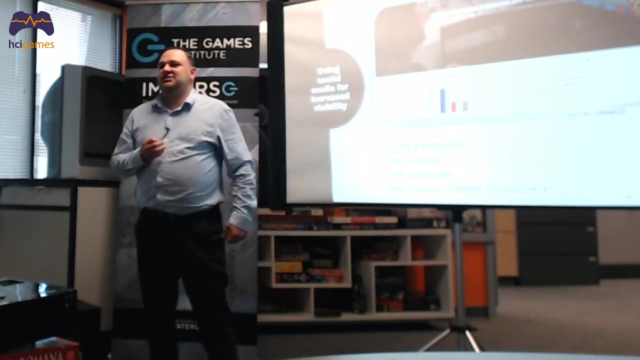 reading log for our Inside Games group, where we have this amount of papers there. In my case, having blog posts about my identification papers allowed them to be well-known and read by people that they read. They gave me feedback and showed interest in my work. 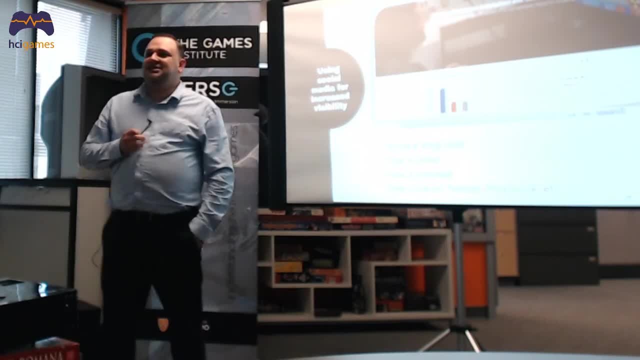 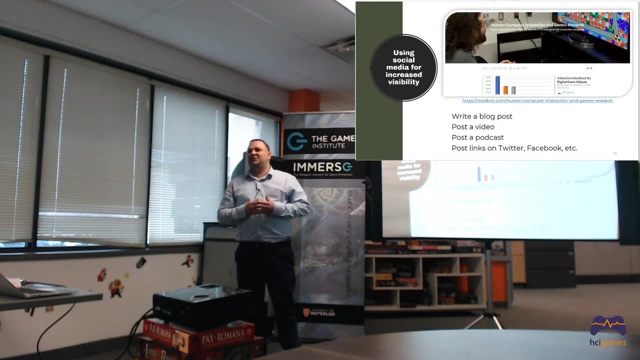 I'm sure it will help even other researchers find your work. It's much better to just read a nice summary of somebody's work first, to see if it's really what you're looking for. If it is, surely you're going to want to. 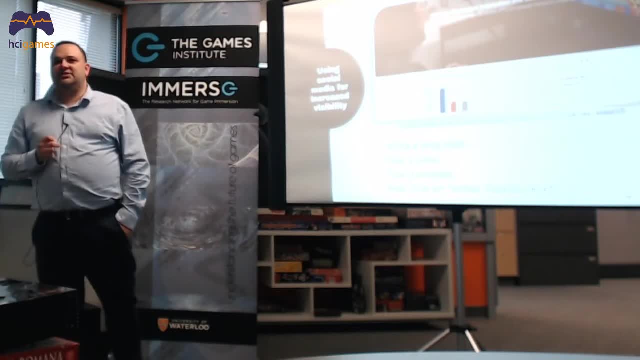 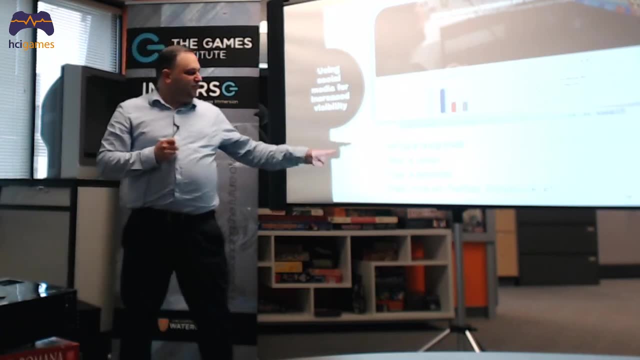 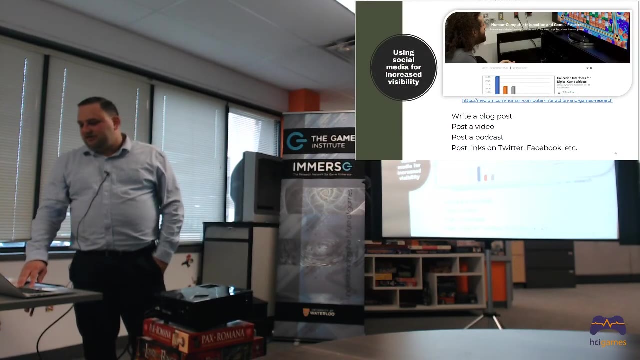 work with videos as well, talking about the research and podcasts. So everything helps bring visibility in a way that's very interesting to do. I didn't put it here, but publishing on social media sites like Research Game I find has been very helpful. 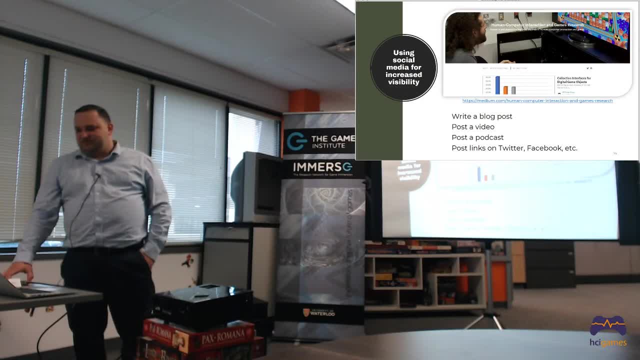 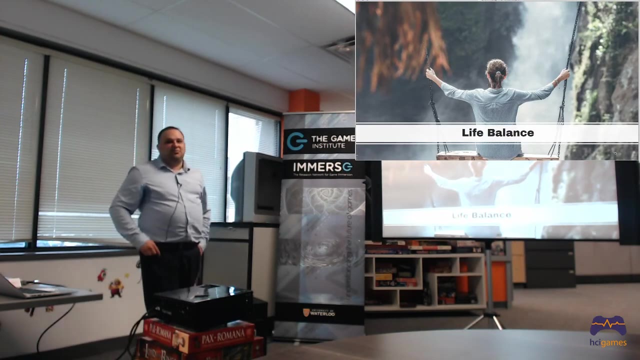 as well, not only for people to find out about an interesting paper from another researcher I know, and that was really related to the topic that I'm working on. It's really something interesting to do as well. Okay, so that finishes the large 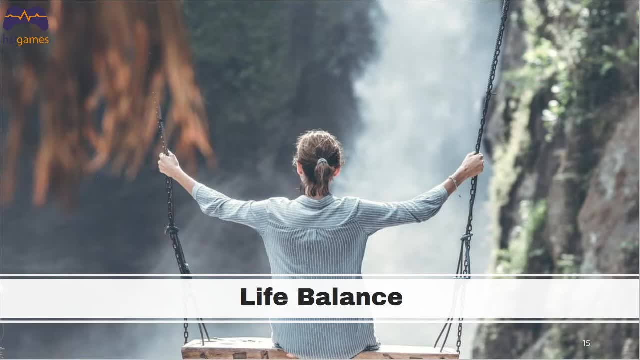 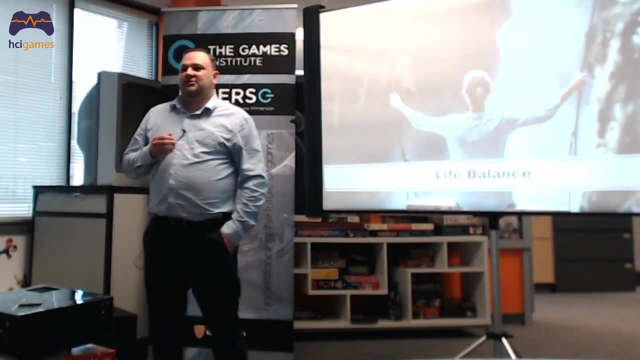 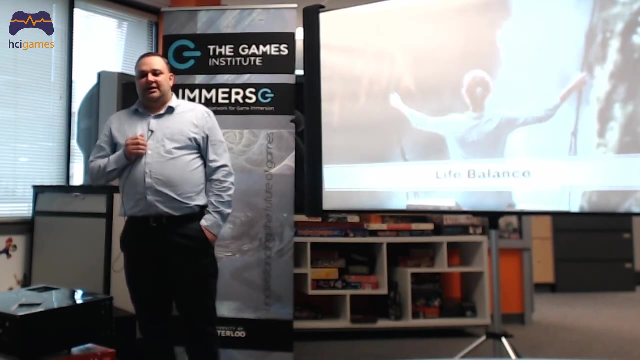 part of planning studies. So just for the last five minutes I just wanted to comment as well that you see it as a graduate student, you need to think about how to balance things as well, And from what I've seen, I think people do. 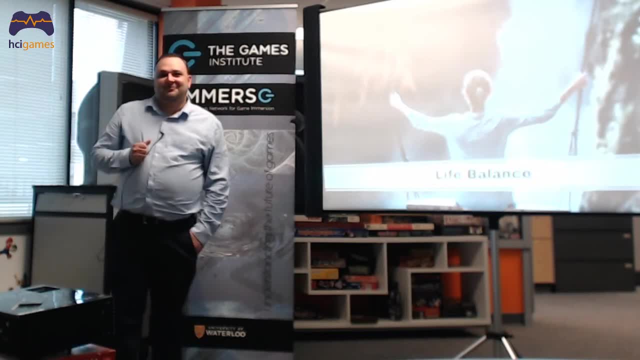 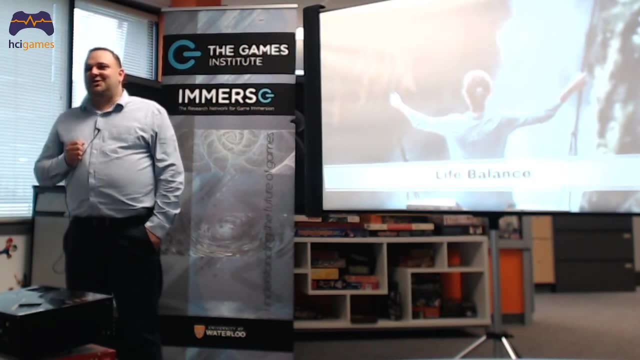 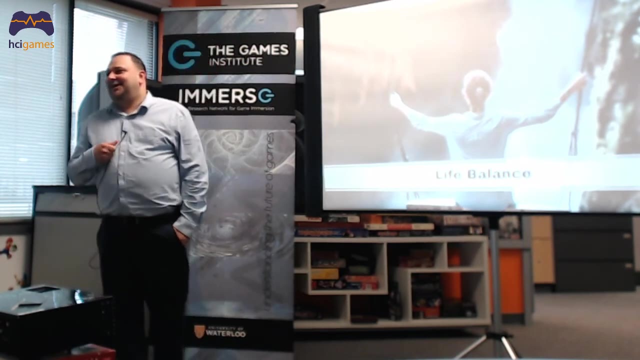 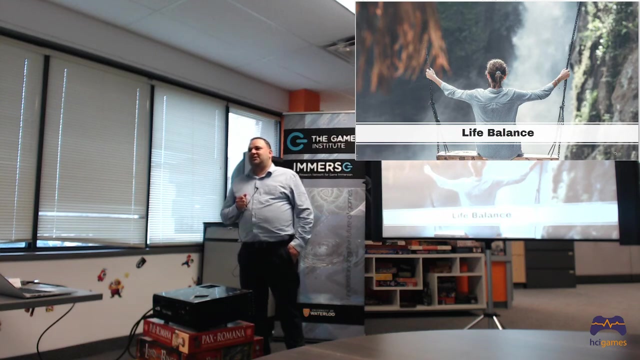 this really well here, without just bringing it to reinforce, because if you look for some sources, I mean, I've seen people commenting on internet that if you keep working too much, all the time you're just going to burn out yourself. You're. 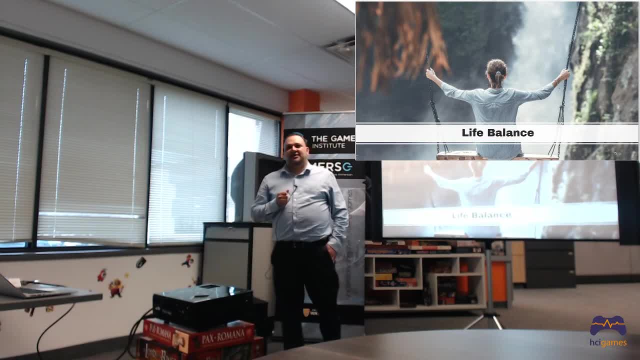 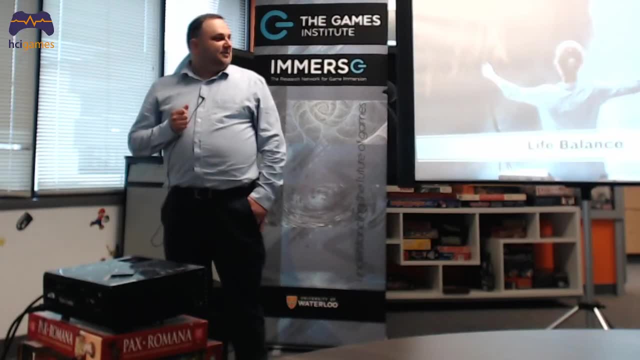 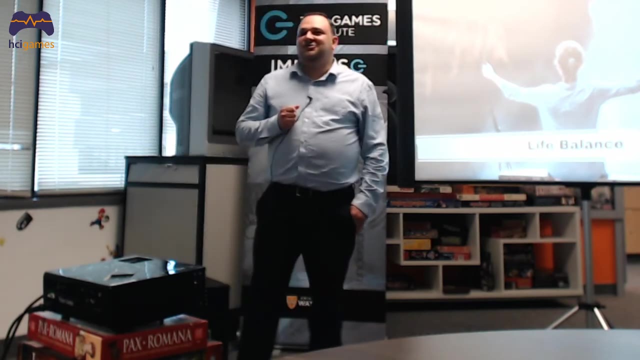 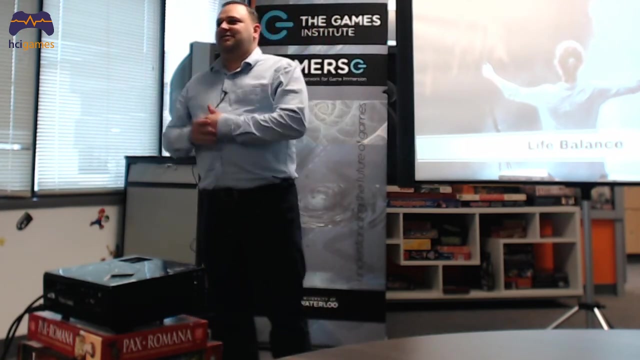 going to be really tired, And after you burn out, no matter how many hours you try to work, you're going to be productive. So I think that's a good strategy. Graduate school students are going to be productive for the rest of their 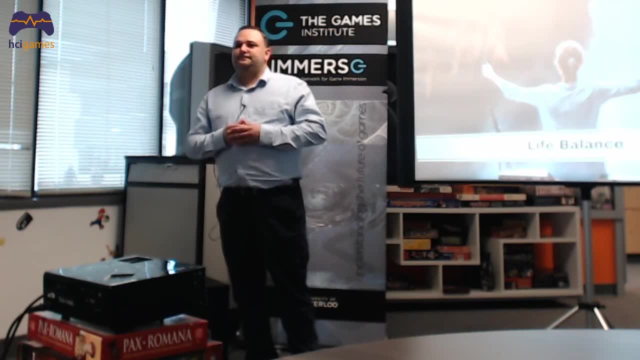 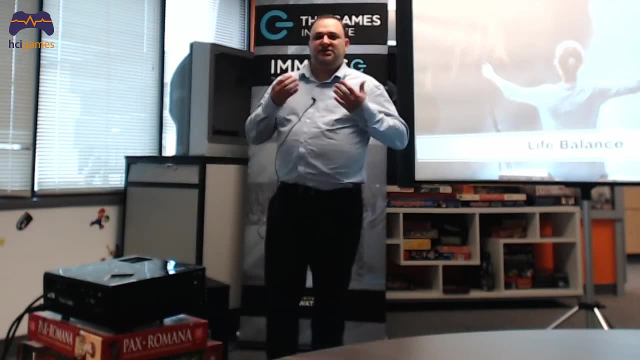 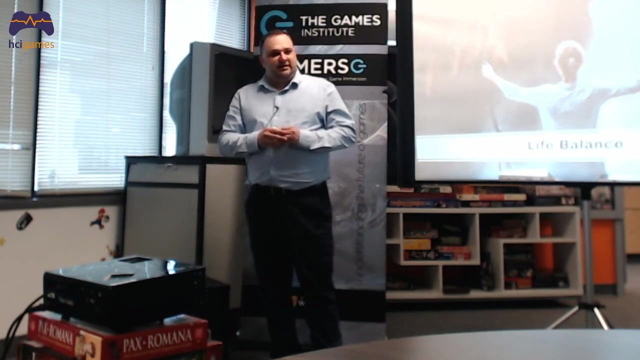 lives. So I think that's a good strategy, And I think that's a good strategy, And I think that's a good strategy. I think that's a good strategy. I think that's a good strategy. They should do things differently. 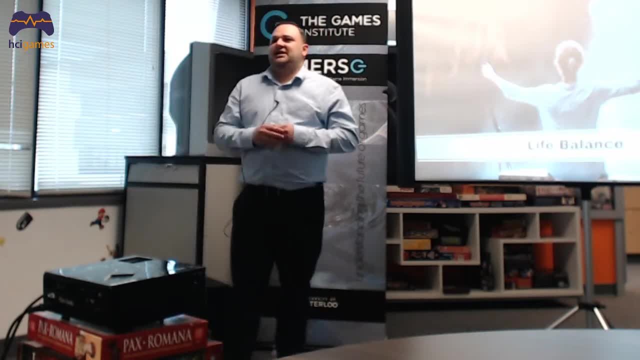 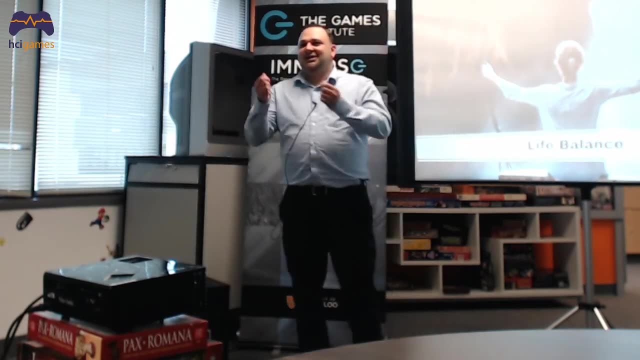 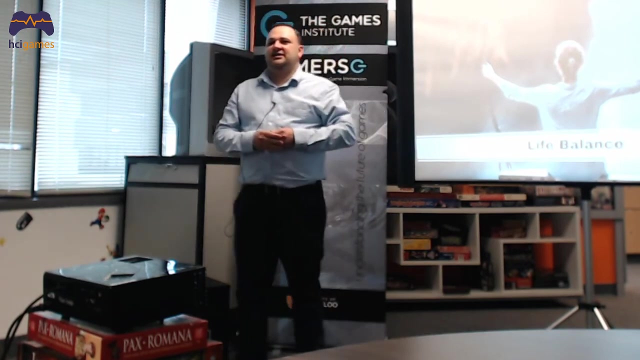 Absolutely. yeah, you are working at the same time as students. Working the same time navigates how you work, wondering what this goal. you try to work from these hours until these hours and then after that we're going to do whatever it works for you to relax and to rest. 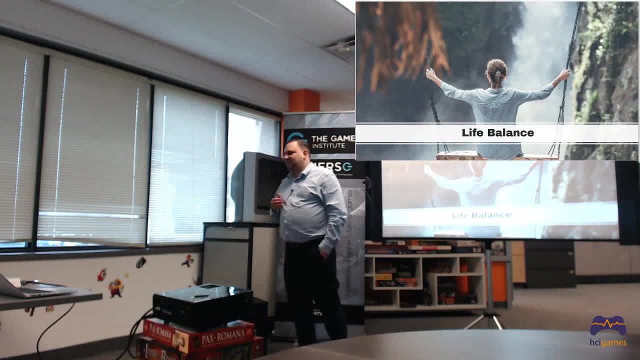 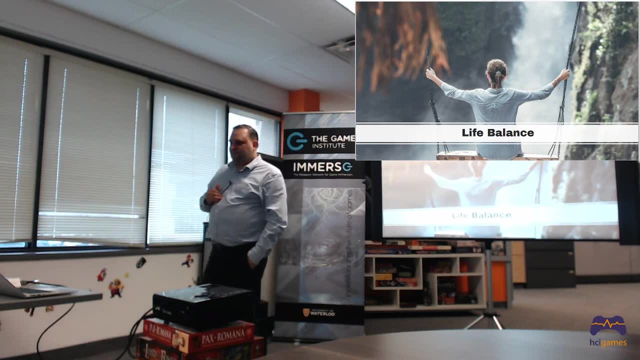 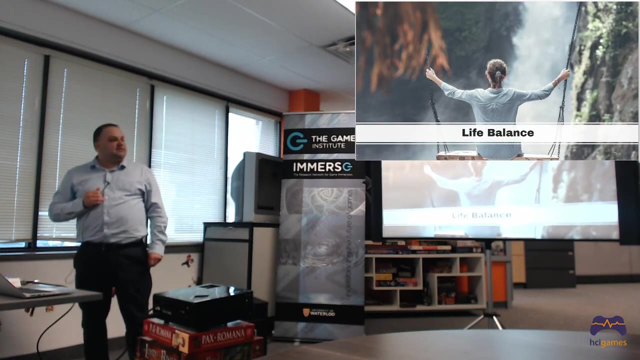 After work again the next day we'll be playing games, not going to the gym, not going outside if you're at a school. so whatever works, At least in my experience. productivity is much higher if you have a balance and you are working a normal amount of hours. 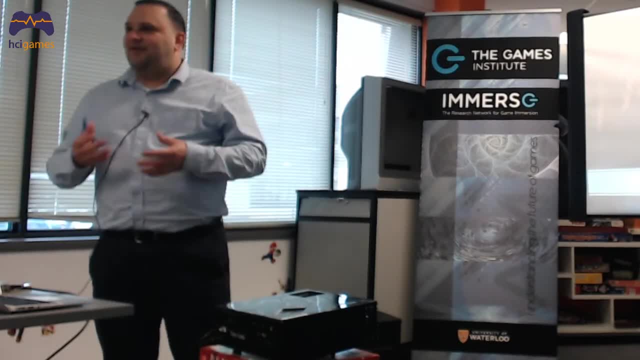 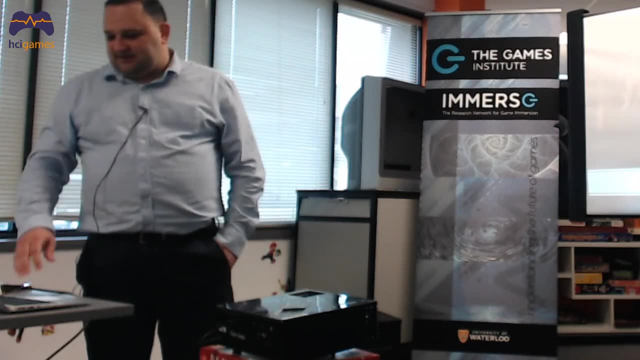 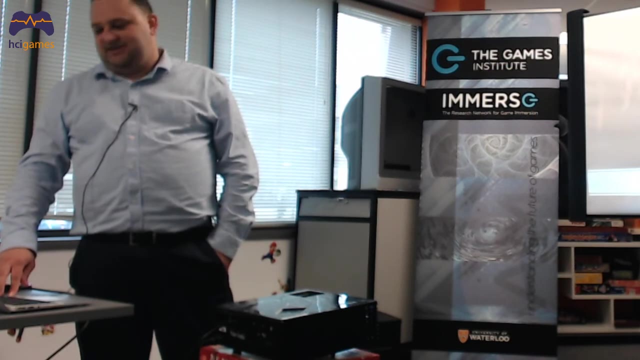 than if you were working long hours all the time. Our work is intellectual work, so we're just not productive if we are too tired. So if you hear somebody saying that if you don't work long hours for years, you won't succeed as a graduate student, I don't think that's true. 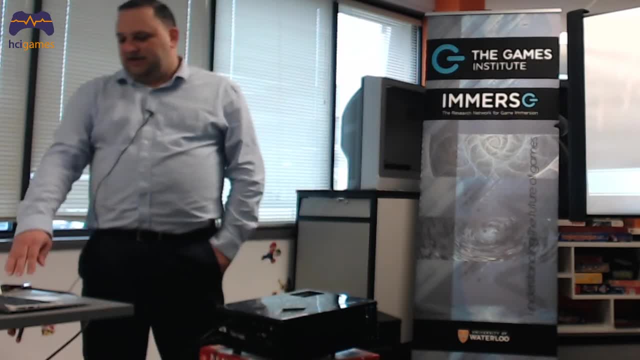 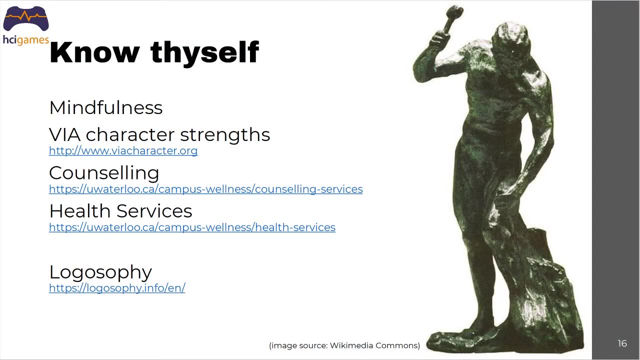 I think that having a good balance throughout those years is what's going to increase your productivity. And, of course, sometimes things have peaks. Sometimes you have a paper deadline and then you're going to stay up until they finish your paper. but it's fine, right. 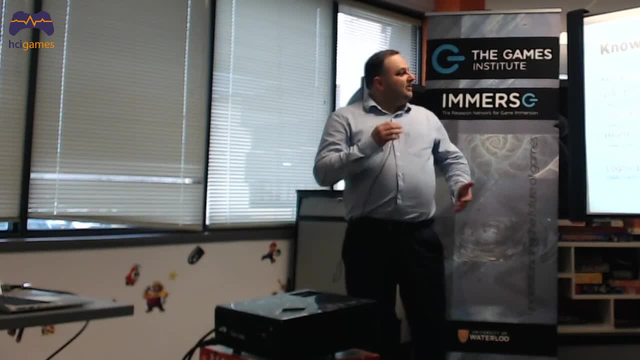 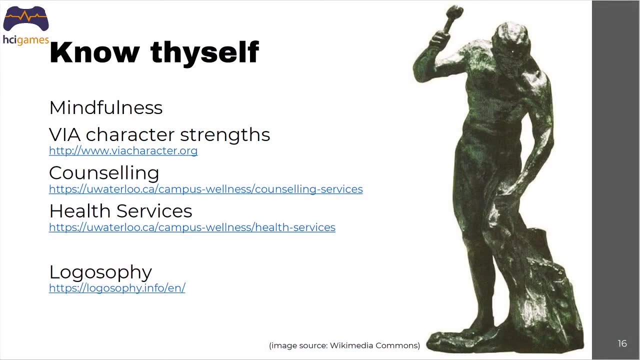 It's not all that bad. And finally, the last thing that I want to bring is this expression: It's even written in old English and people have been talking about this since ancient Greece, so know yourself. But I wanted to bring this because I feel for me. 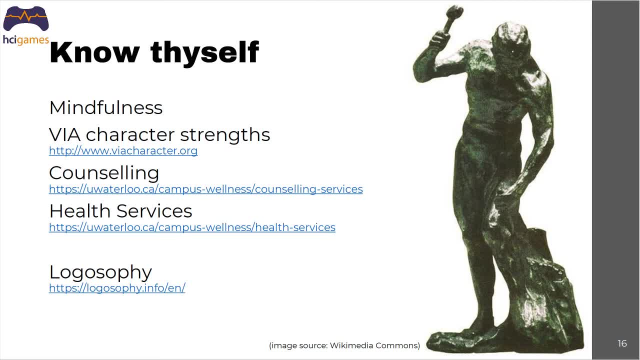 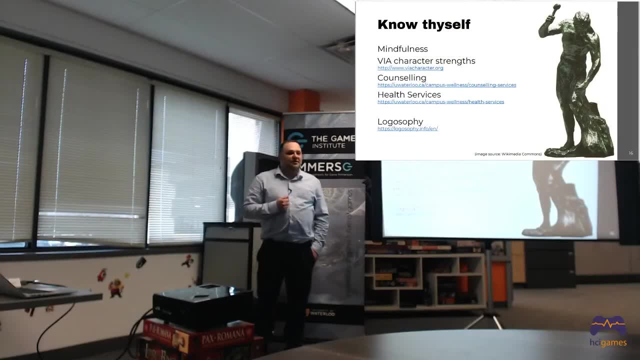 this has been something important as well. This is not only for graduate students, actually. This is for anything that you're doing in life. If you know yourself better and you better know how to deal with situations, it's going to be easier for you to succeed. 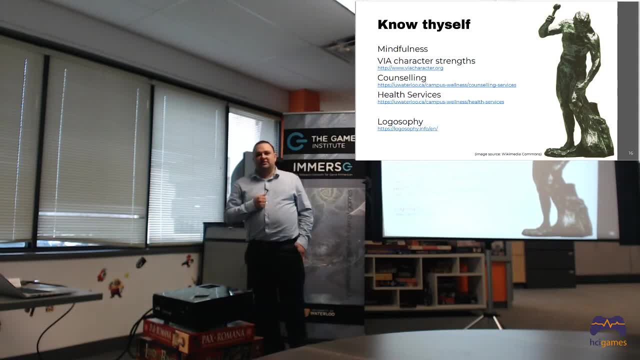 But especially for graduate students. people say- and have statistics say- that it's usually more difficult psychologically than being a graduate student and working a regular job, So this becomes even more important. So what I'm trying to mention here is to learn about yourself as well. 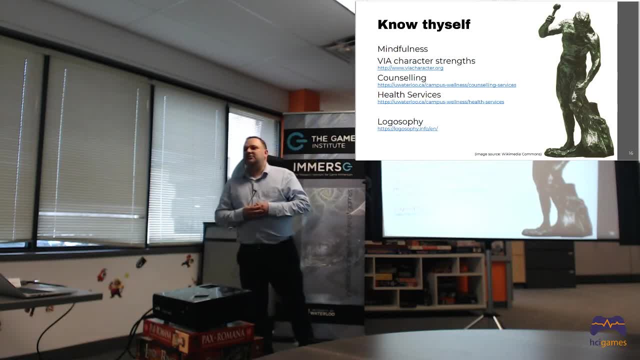 How do you feel when you encounter difficult situations? How do you manage them? What can you do? Because learning about these things really can make a difference. It's usually something that you can't do. Right, Right, Right, Right. We're just not taught at least as much as other things. 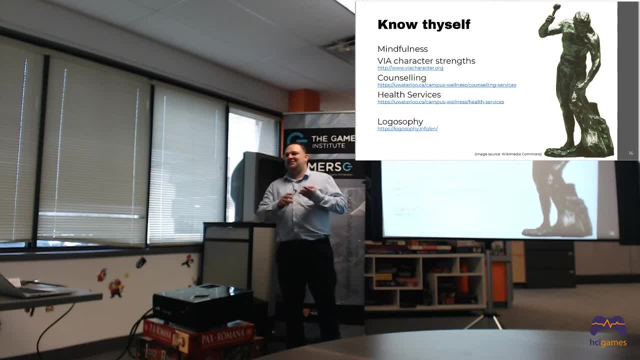 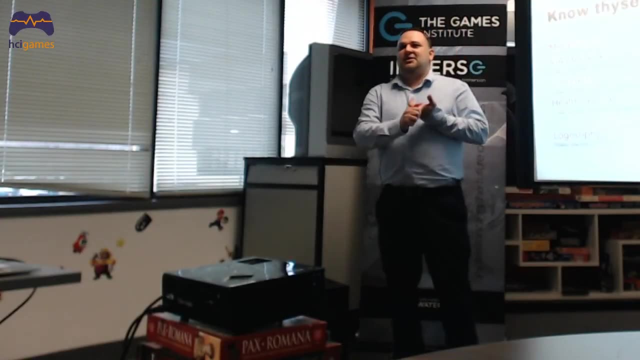 We learn about science, about statistical methods, and we learn about things, But usually if you don't co-study about yourself, you might not learn anything about that. So try to learn about how you can manage it. Think like you are in a stressful period. 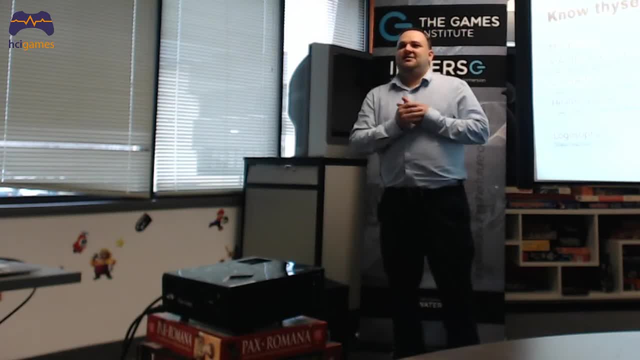 with too much things to do. How can you handle that? Maybe you had a conflict with someone that you were working on. It makes you sad. How can you work with that? Maybe you tried something and it didn't work. How do you deal with that? 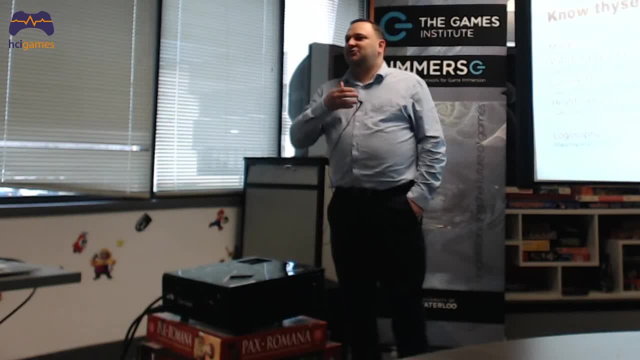 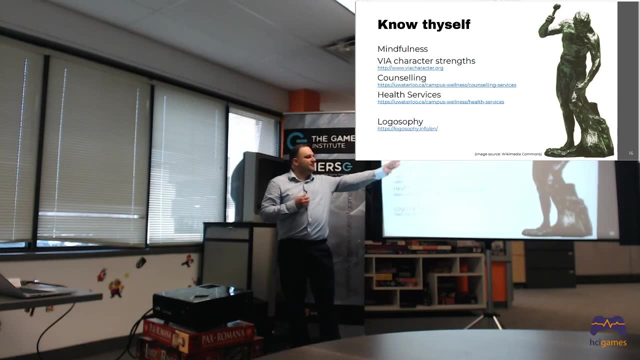 So these are all things that we can learn how to do better, And there are so many different ways. I just put here some of the things that I've heard about. heard people talking about, So some people have been saying that they've tried mindfulness. 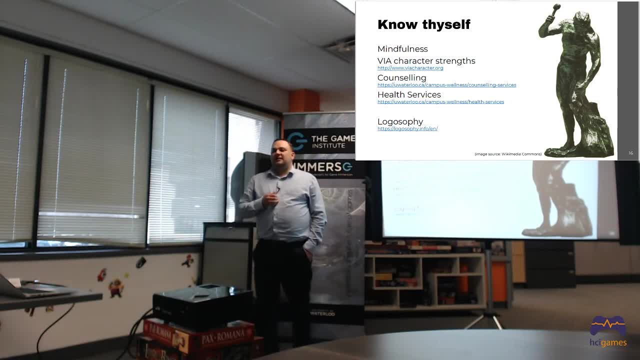 which is meditation, and it's helped them to better understand their feelings and better cope with them. to try this now from psychology, these wild character strengths. You can take a normal task and then it gives you a list of what are your psychological strengths. 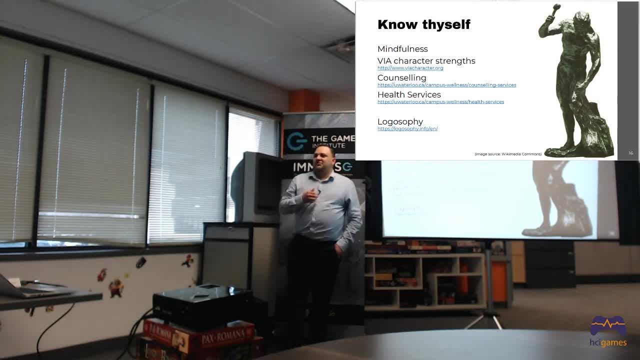 and what are you looking out to put on so you can focus on using your strengths and your feelings when you try to study about the things that are your weaknesses and learn about them how to improve? And, of course, I hope everybody knows that. 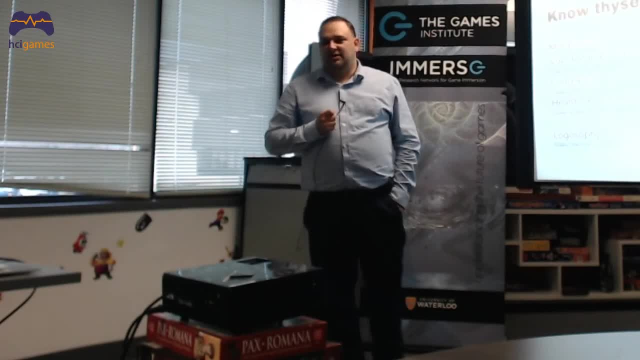 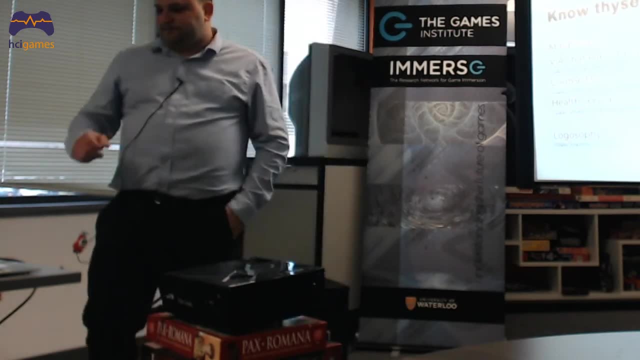 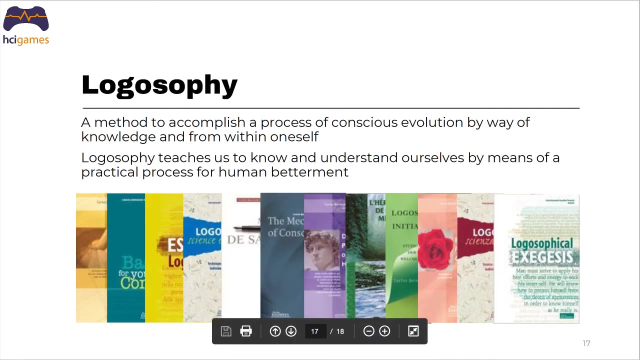 but if you need help, the university has resources here with counselors and doctors that you can reach. also talk to somebody. And I put the last item there, which is for me, what I have been doing for years at JCCC, Sorry, 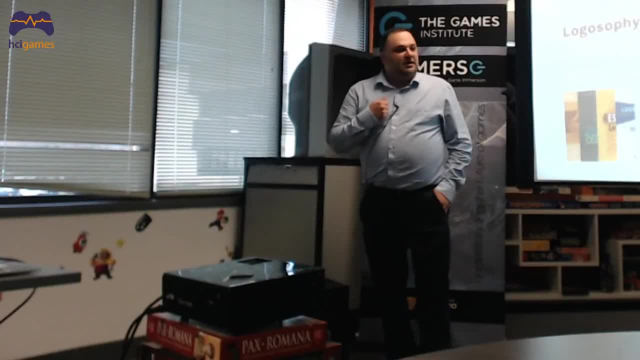 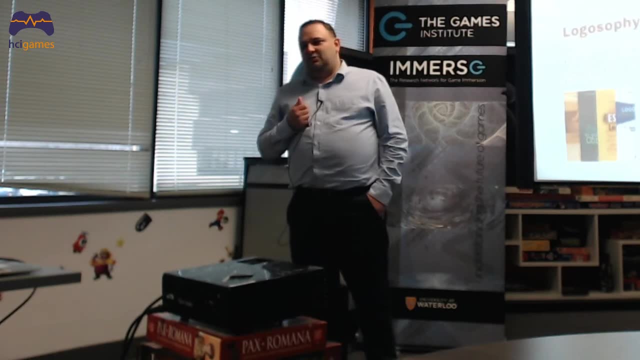 I'm a graduate student and it has been really helpful is student philosophy, which is a method that helps to exactly what I said: help me study myself and understand why I do things the way I do, how I feel the way I do. 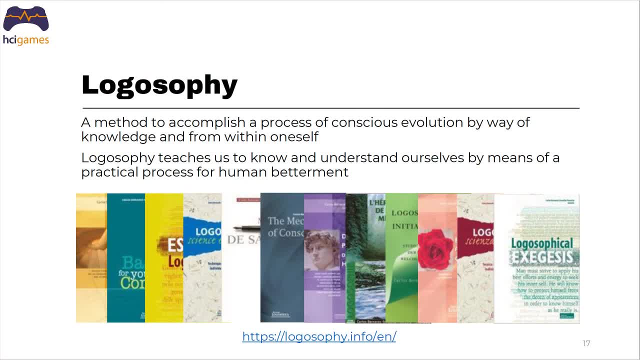 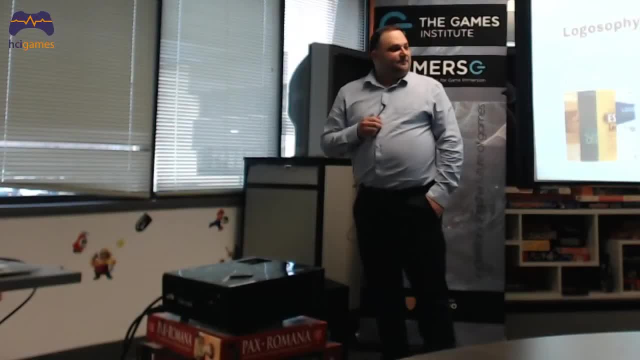 and how I can do things differently, how I can learn to be more patient, how I can learn to feel better. I could learn to speak in public better, which for me was quite difficult some years ago, but now it's easier. So just to mention there, because we are on time: 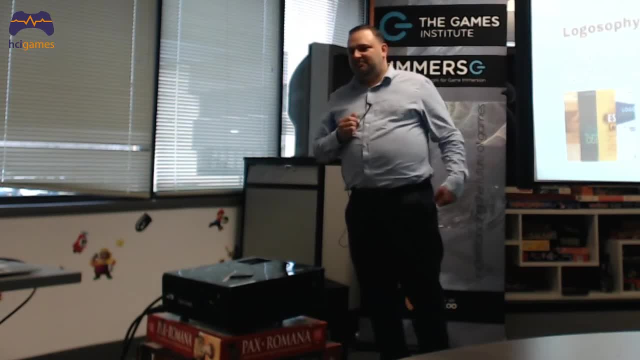 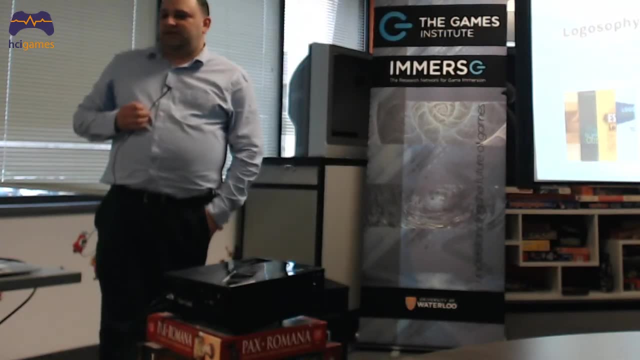 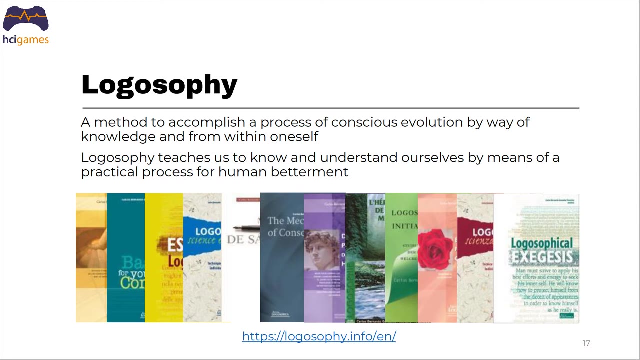 but if that seems something interesting to you about philosophy, I know a lot about it And there is a website there with information, books you can download, of course, that you can ask for. So if that seems interesting, ask me about it and we can talk to you. 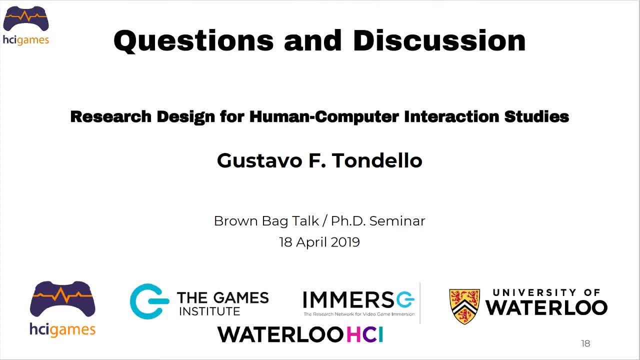 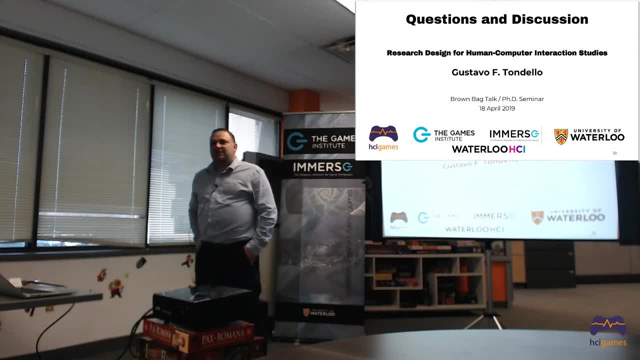 So thank you for listening. This was a bit longer than I expected, but if you want to ask something or to comment about something that I talked about, or if you have any interesting experience or tips of your own, so if you want to bring it last time. 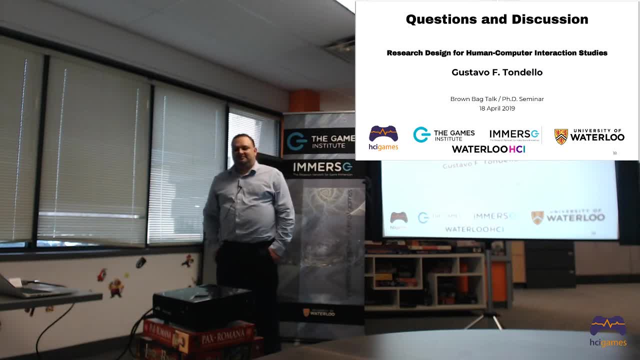 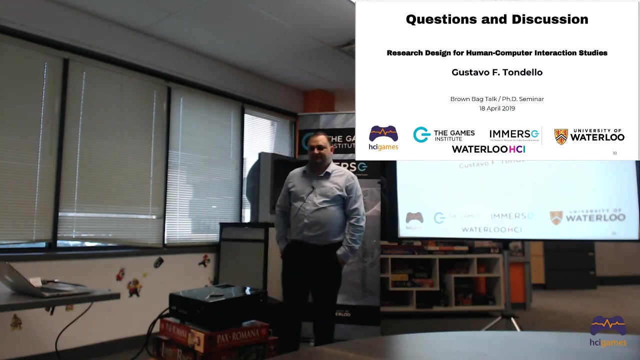 Any questions or comments. I actually have a question relating the beginning of it all, because a lot of students struggle just to kind of get into that mindset of you know how do I even find something that's worthwhile in this field? Do you have any tips for students that are interested in that? 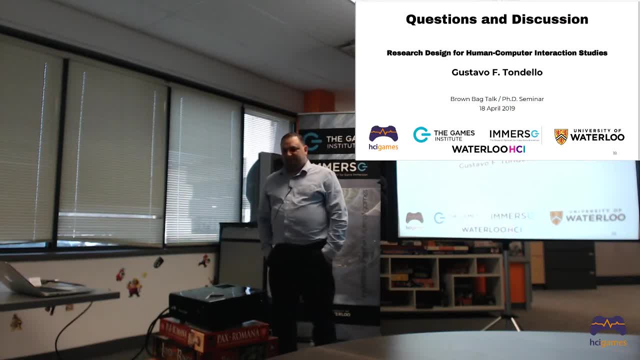 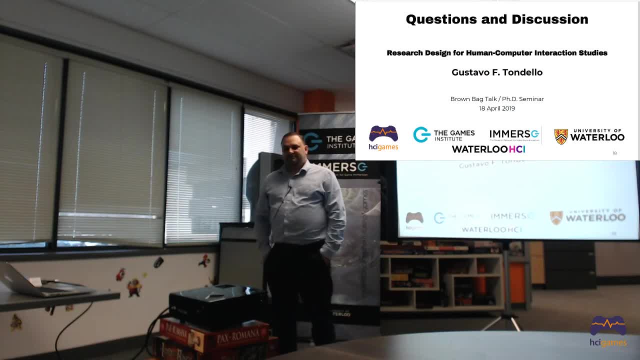 that does everything and anything. How you know? what strategies would you suggest? can they apply to focus? Now, in your case there was a specific coincidence that things worked out the way they did. you know that might not apply to everyone, Yeah. 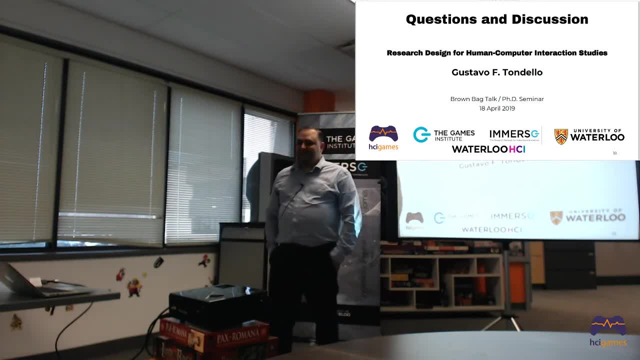 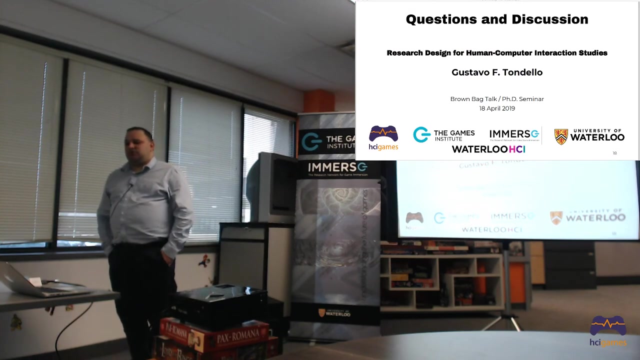 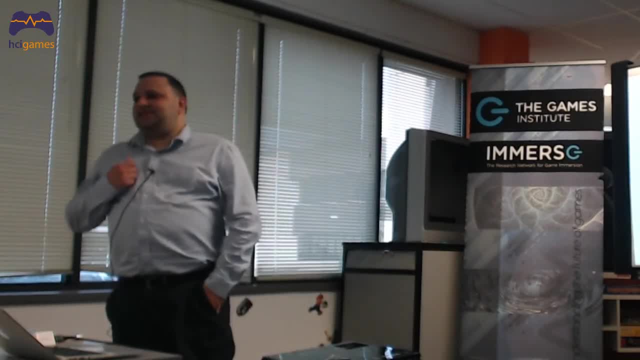 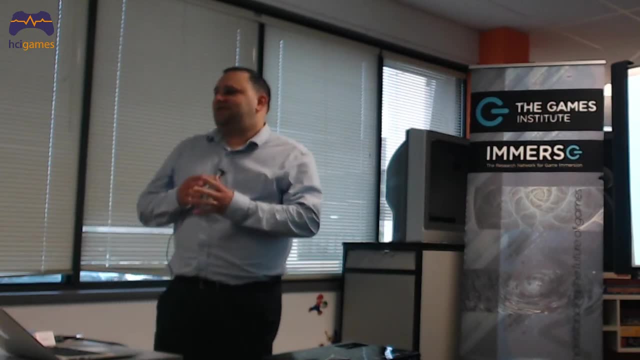 First, as I said, HCI is a very large field. So if you just start to do anything HCI, you're going to be lost. So first, I think you need to narrow down to within HCI, specifically where you want to work on. 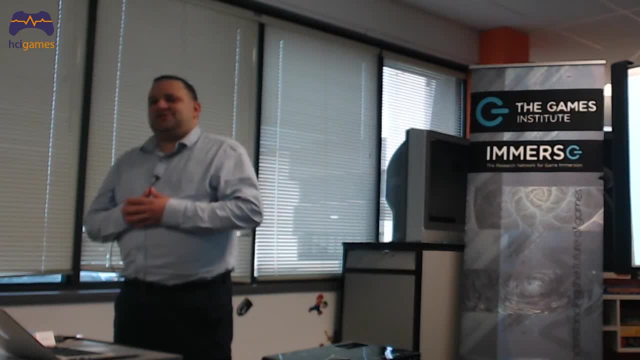 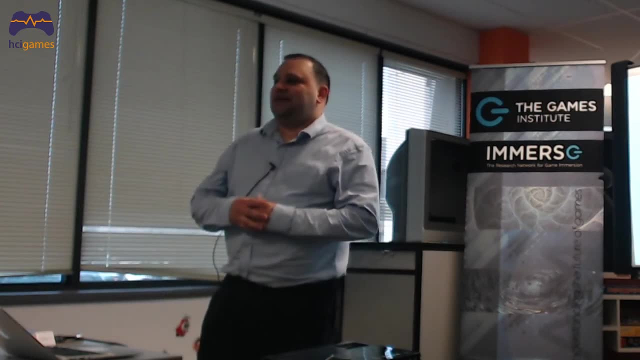 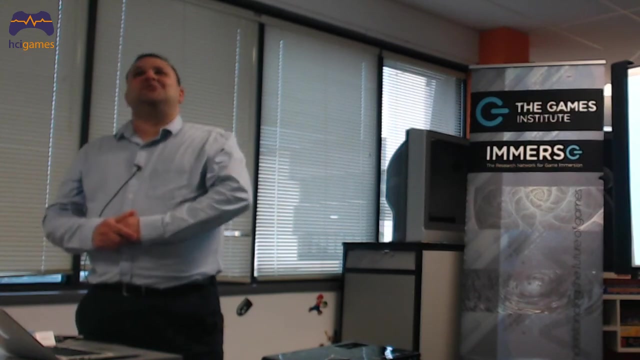 And for that, I think it's just a matter of preference, because there are so many different things that can work. So what do you want to work on? It's just you have to decide. Once you do that, I think that don't then sit on your desk and try to come up with an idea out of the blue. 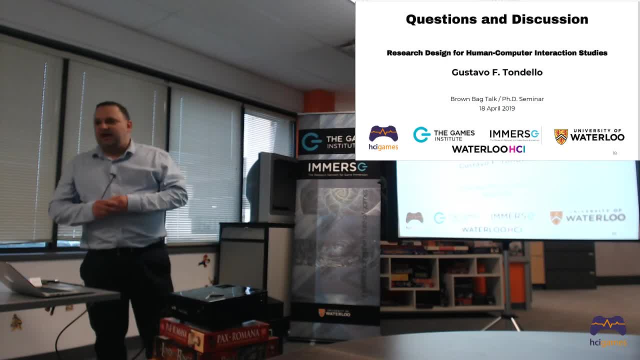 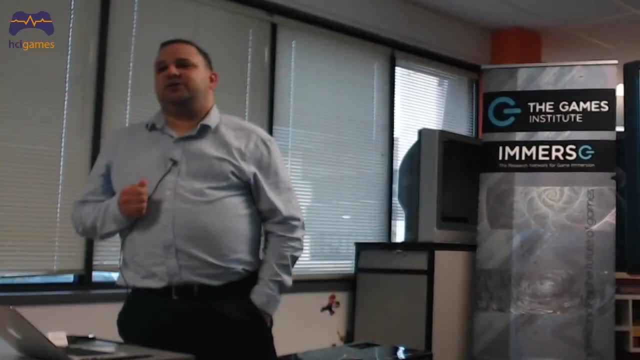 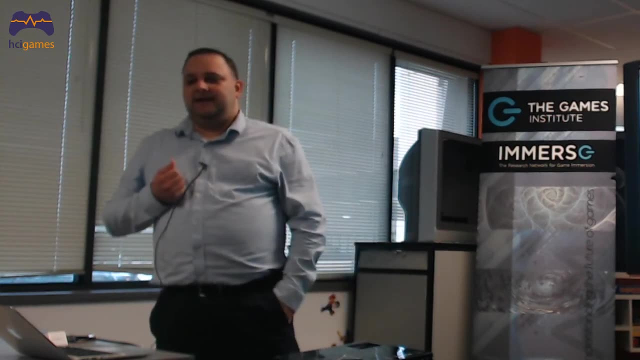 Okay, It's hard, And once you have what exactly where you want to work on, I would say go and see what people are doing there. Read papers, Go to conference, Maybe go talk to people here at the GI and ask what they're doing. 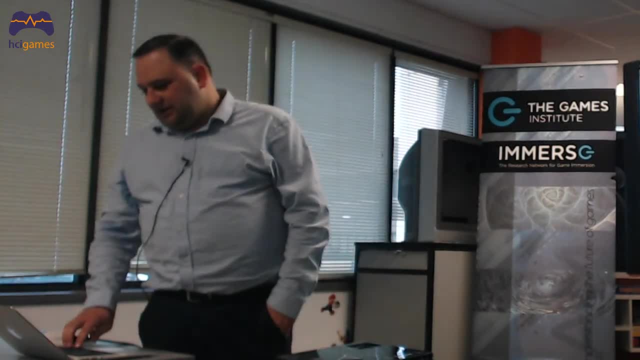 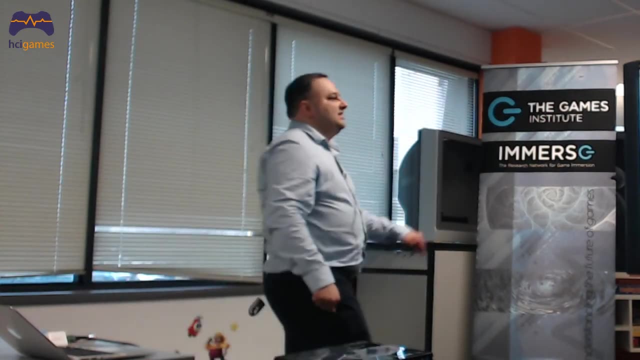 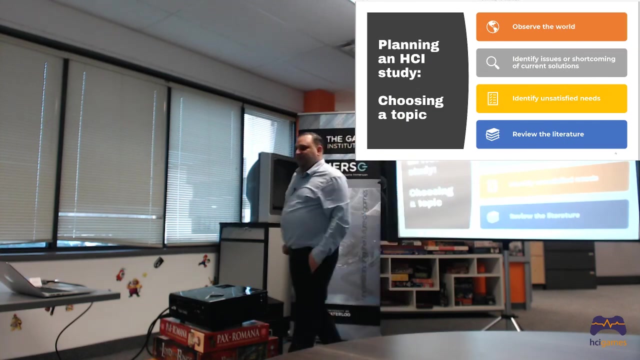 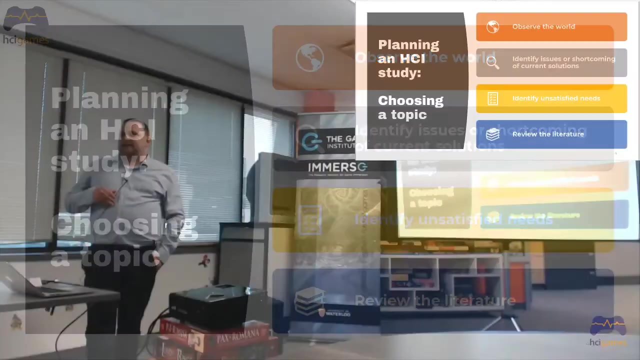 Try to look for those things as I have them. This slide: These are the things. The next slide: These are the things I look for when we are looking- Okay, What people are doing. Try to find things that have an issue or a shortcoming that maybe you can try to solve, or try to identify someone saying that they need something that doesn't exist yet. 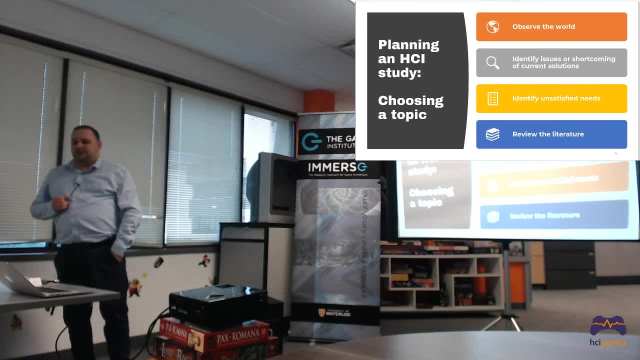 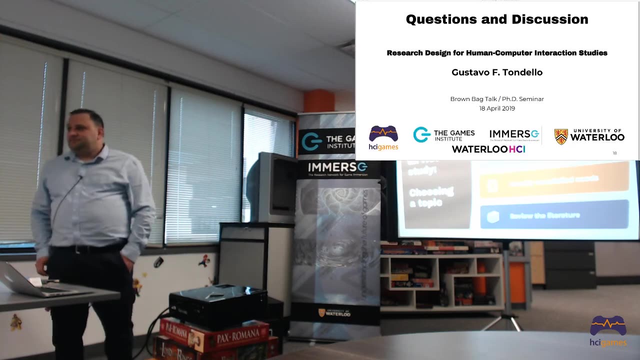 So maybe a person that is going to solve that need. That's what I can suggest. So, in terms of knowing thyself and self-improvement and such, You mentioned a couple times how early on you weren't as rigorous in your study designs, your statistics, as you have become. 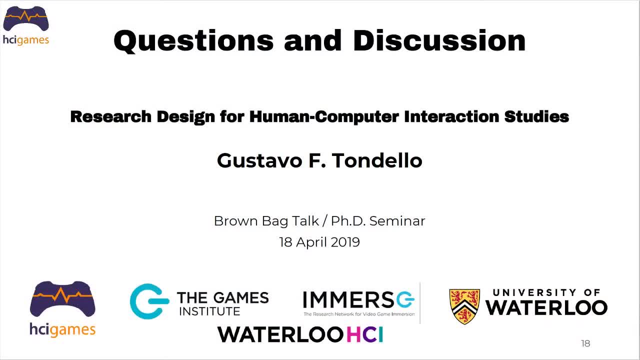 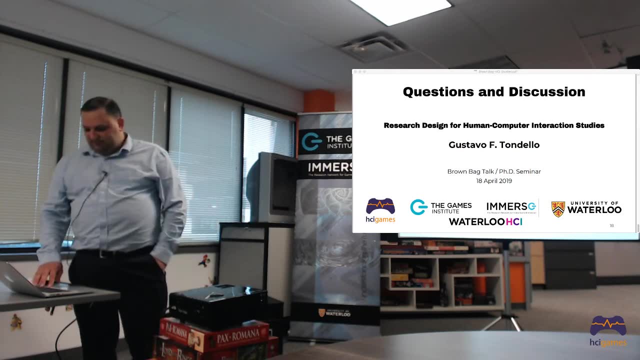 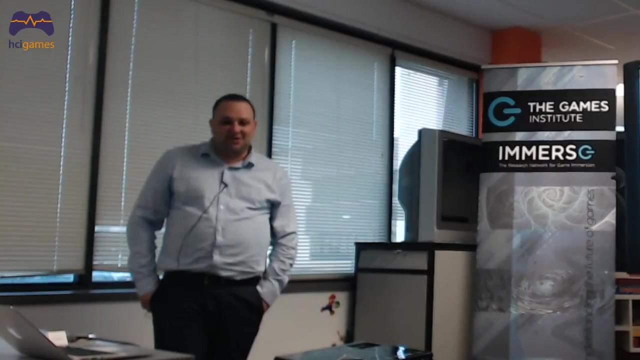 Is there something, now that you're close to the end, that you can identify? you're still working on That. you've begun to work on. Well, Let's see What can I say. I mean learning. One thing that I'm always working on is learning statistical methods. 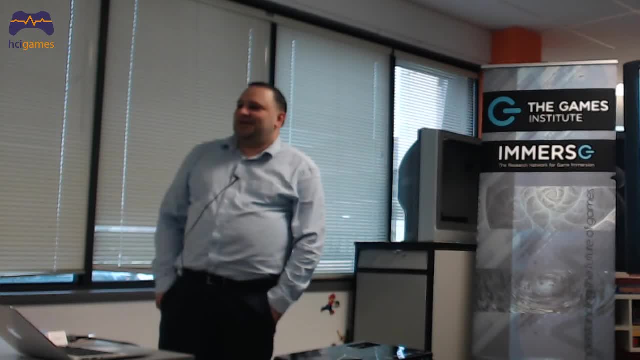 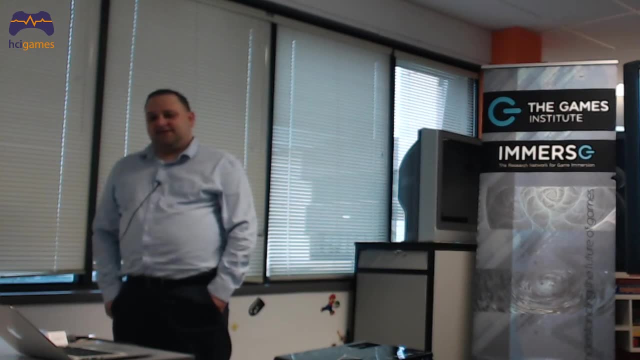 I didn't learn them all in the beginning. I think that's. There's just so many that I just don't. I did try to learn them all in the beginning, But in the beginning I love reading a book to have an idea of what methods are out there. 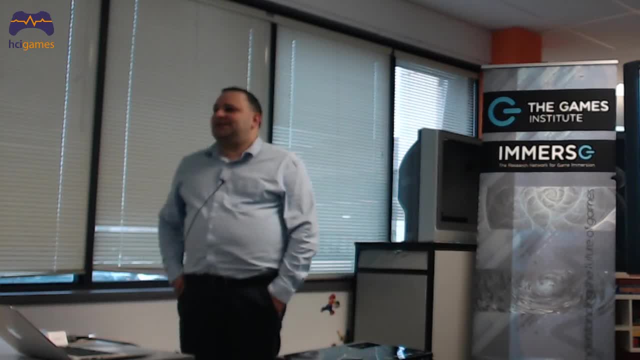 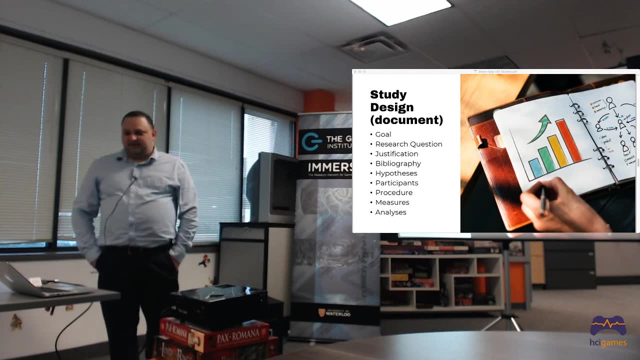 But then each time I do a different type of study And I have to look for it And I need to go there and study that particular method to use for that situation. So learning statistical methods is something that I'm always doing And yeah, 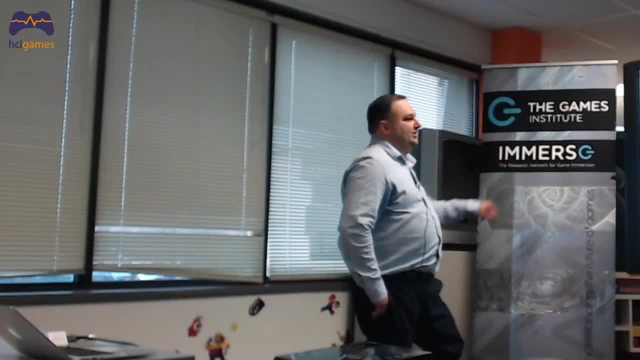 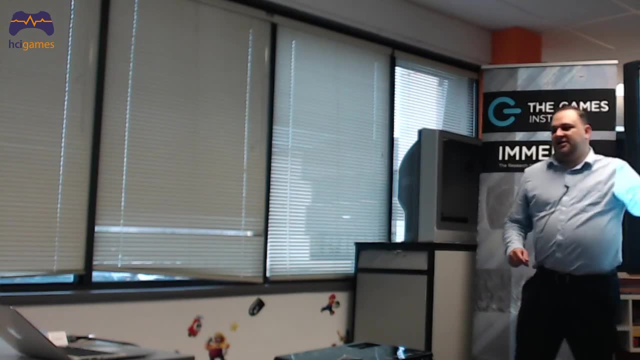 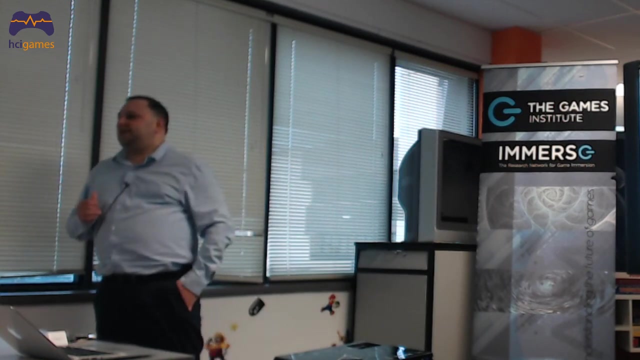 Something for my current studies. Something that I'm trying to improve is actually this part here, Like having preparing the study, Having already in mind What I'm going to say later, How I'm going to present that study. So I've just begun doing this for my studies.